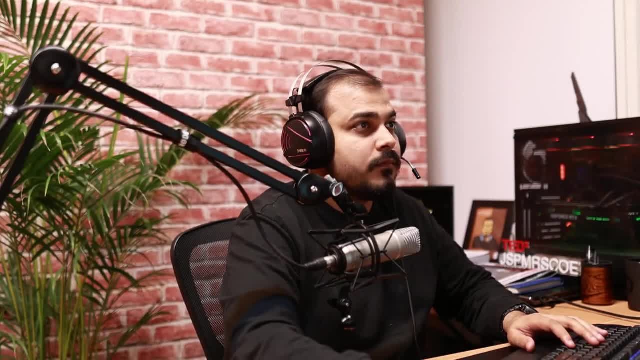 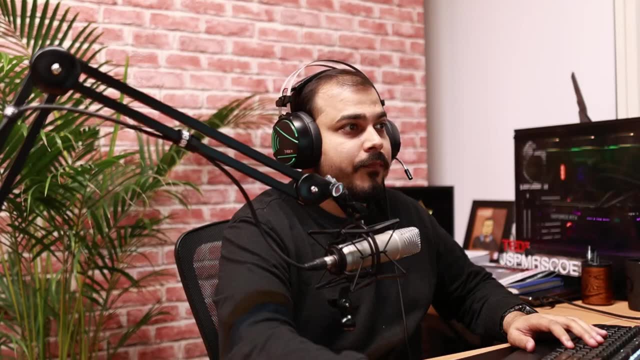 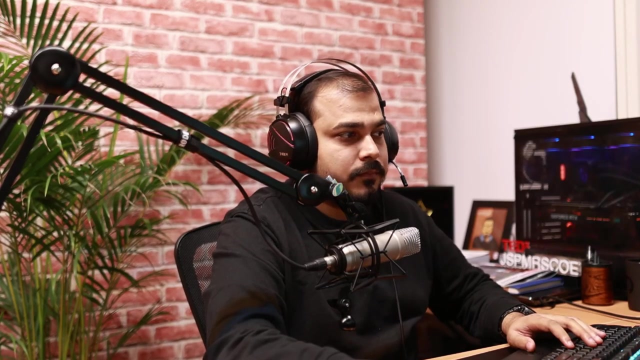 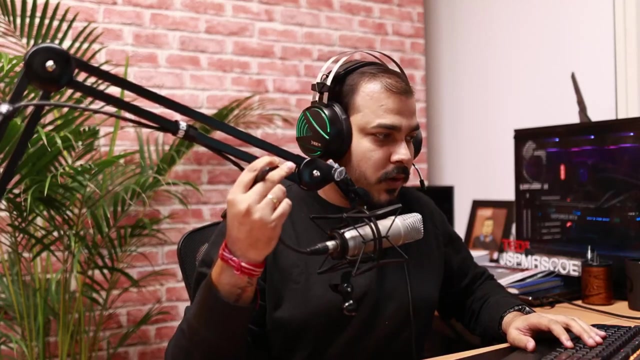 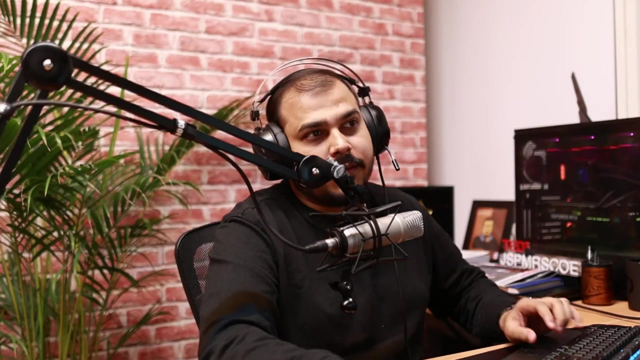 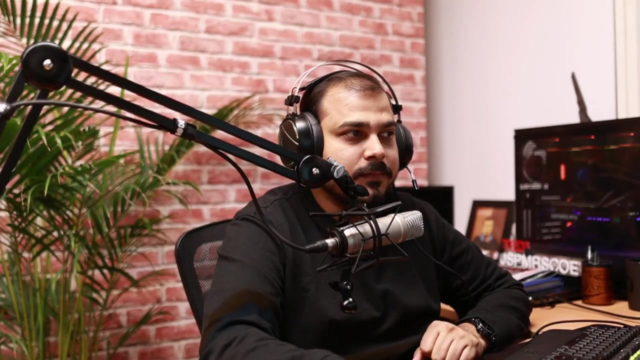 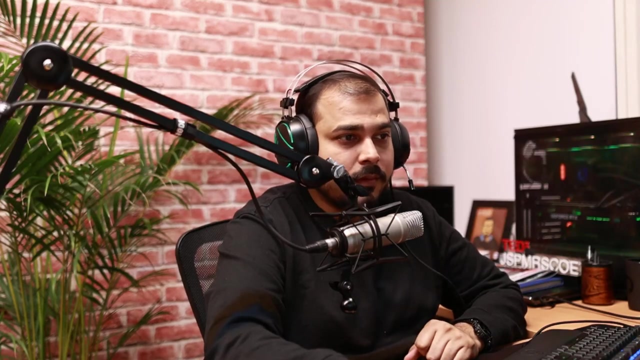 Thank you, Hey guys, am I audible? Can you give me a confirmation, if you are able to hear me out quickly? Hello, hello guys. Am I audible? everyone, Yeah, perfect, Yes, yes, everybody, Yes, perfect, I hope everybody. I am audible for everyone. 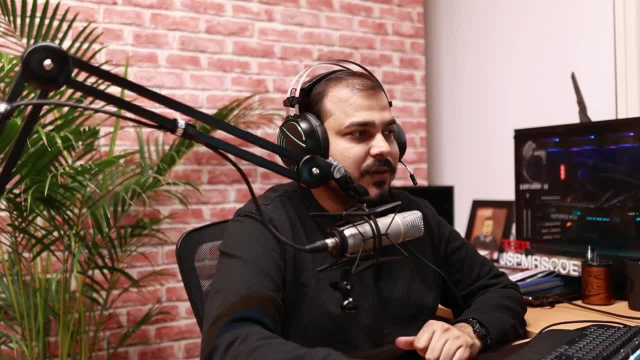 Please hit like if you are new to this channel. And yes, today is the day 5th. I am sorry I could not take it before because, again, due to some of the other work I was involved in many things. 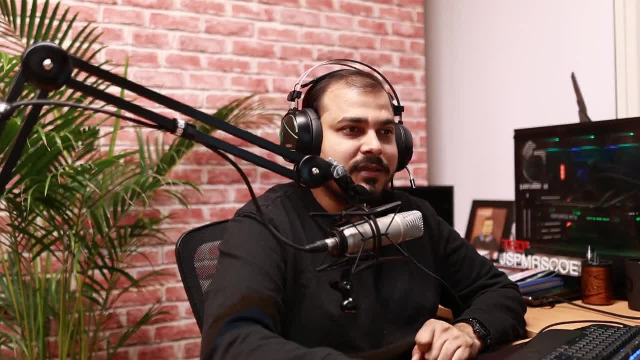 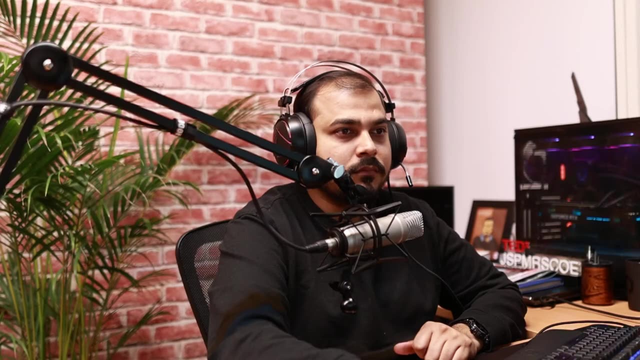 So I could not take. But anyhow, today we will try to complete CNN. It's a simple imitation, Right? So we will just be starting in some time. Yeah, Hello, hello everybody. So another 2 minutes. 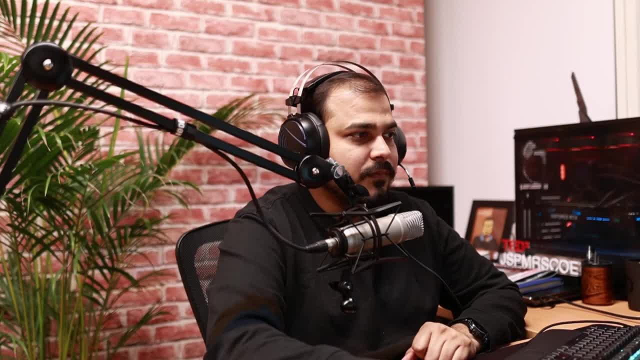 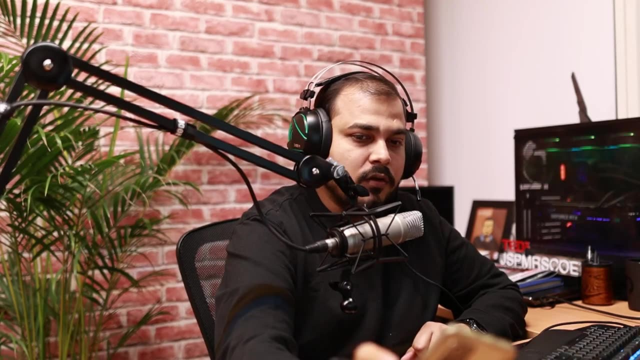 So then we will probably start, But I hope everybody is doing fine. Well, So today I will try to finish up the day 5th as planned and then probably will go with NLP section. community section- Community session. 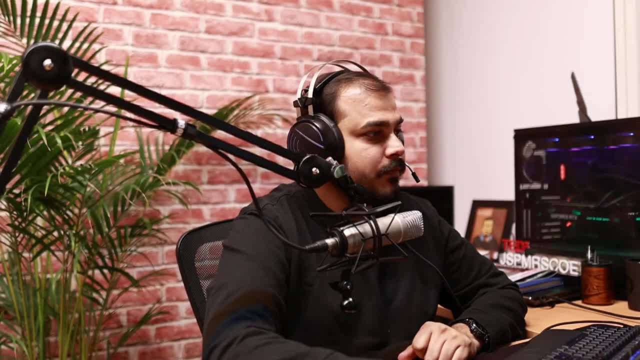 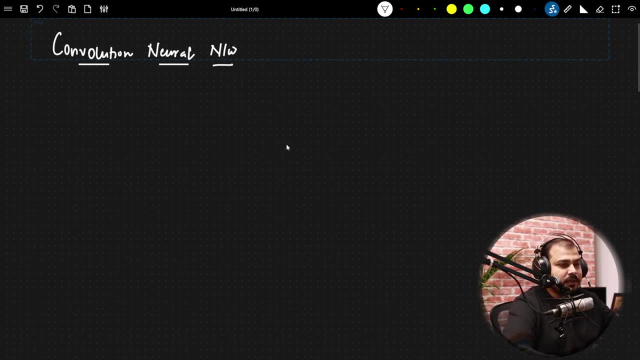 Okay, Okay. So today we are going to discuss about it And, yes, you know, we will discuss in such a way that we will try to first of all understand how does cnn work and then we'll try to do the implementation, and probably a week or 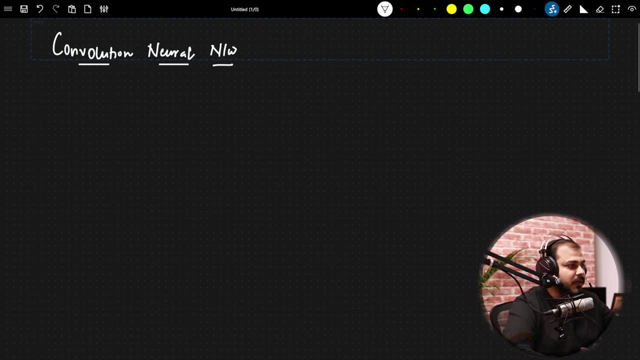 time we'll also start nlp classes, okay, so nlp again. that will be like day five, five days live session on that too, as a community part, okay. okay, as you all know, we have already discussed about ann. now we have seen the theoretical explanation, right, and then we also saw the practical part. and when we were discussing 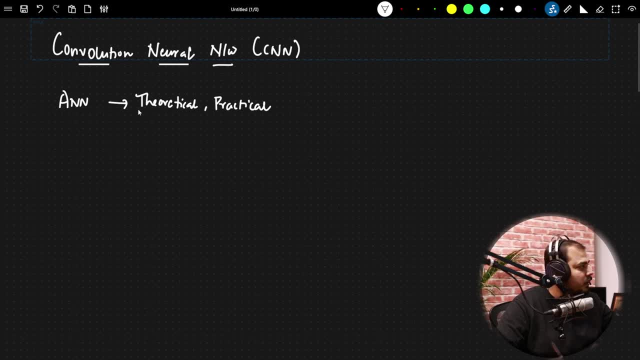 about optimizers, loss functions and all the things in this, but in today's session we're going to talk about the practical part and then we'll talk about the practical part. in this session we are going to discuss about cnn. cnn will focus on understanding what exactly. 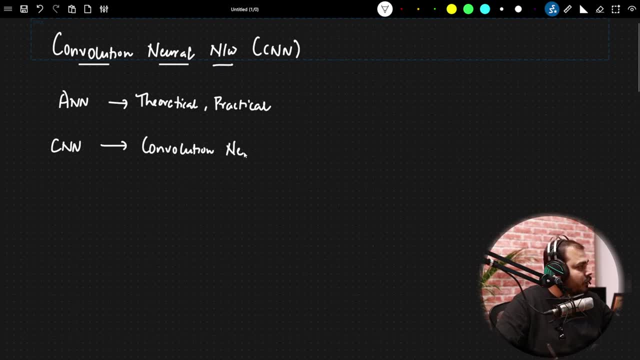 is convolution neural network, convolution neural network and how specifically it works. whenever we talk about convolution neural network, we are basically going to mostly discuss about images and, let's say, video frames, right. so whenever we have images and probably we want to work with that, you know specifically related to, you know, different kind of images itself, some of the tasks like image. 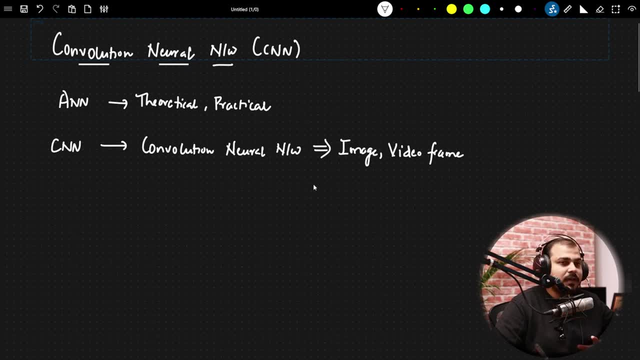 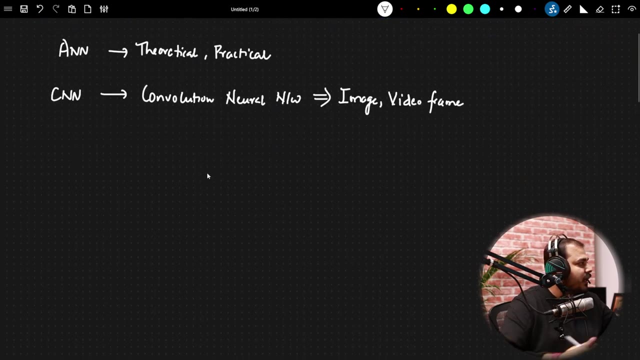 classification, object detection, which we specifically used, a different kind of cnn networks which are focused more on detecting objects in a specific images or videos itself. right, so, as as usual, the agenda will be that we will try to divide this entire topics in understanding. first of all, uh, we'll try to understand about cnn versus human brain. okay, because this is really in. 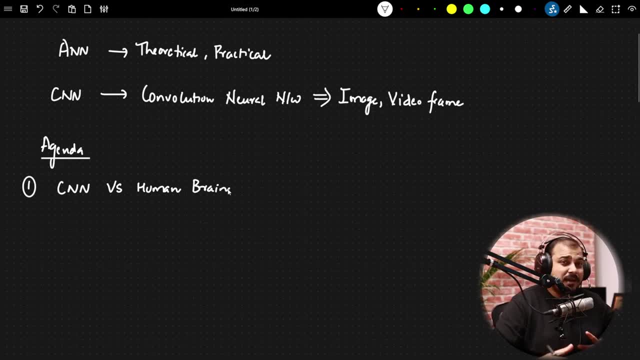 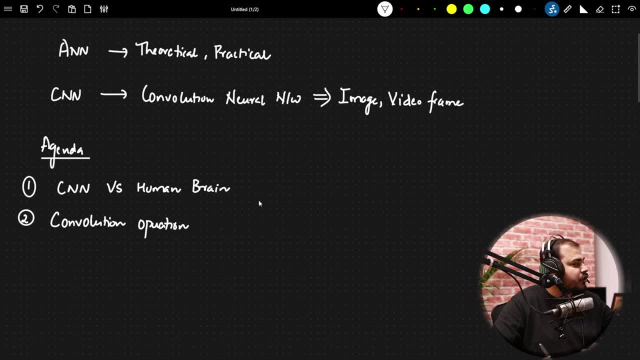 convolution operation, convolution operation. in this convolution operation, we are going to discuss about various, various words, uh, that i'm going to bring up over here, like, uh, what is convolution, okay. what is padding? what is strides, right? uh, we will be discussing this, you know. and how do we determine that? how the output of a 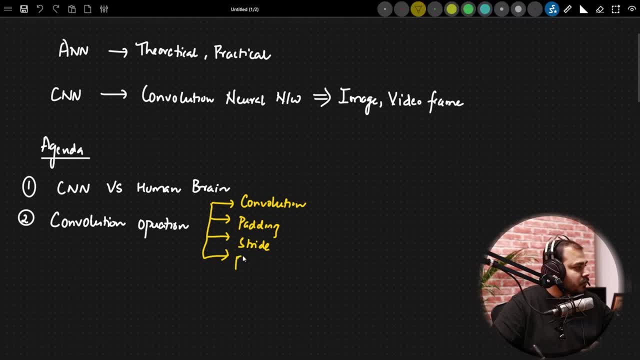 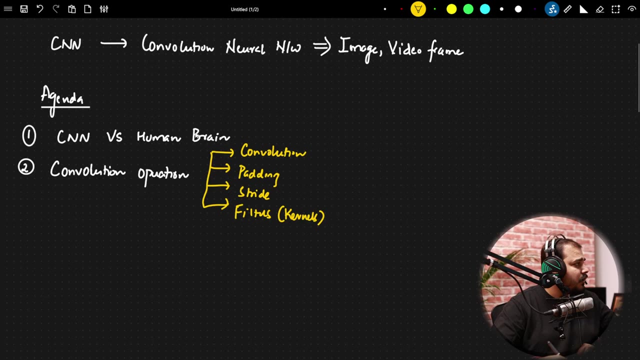 specific image will look like after we pass through this: filters, filters, filters- the filters are also called something called as kernels. okay, so we'll also be discussing about this specific thing as we go ahead. once we complete this two uh, then, uh, we will be discussing about the third part, which is called as max pooling, and in max pooling, uh, we will try to understand what. 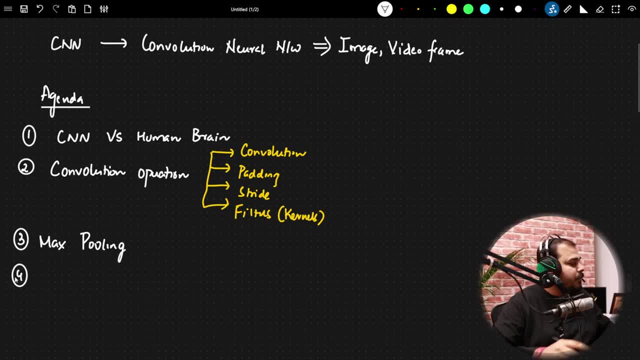 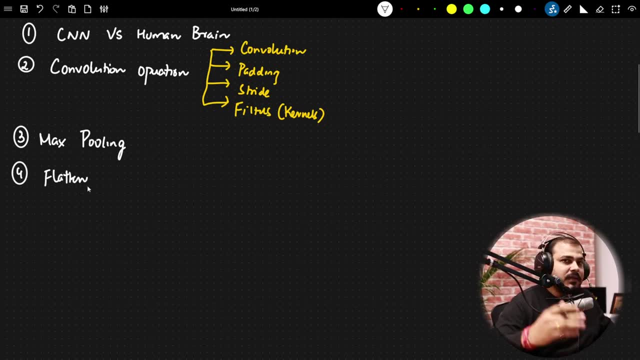 is the importance of max pooling itself. and the fourth topic will understand about the flattened layer, which is again a function of kernel, because we cannot control it. but we can control it by one amazing thing that happens in the final layer of the cnn itself. so we specifically call it as: 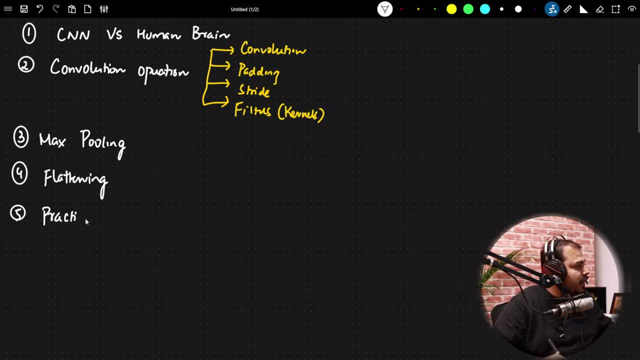 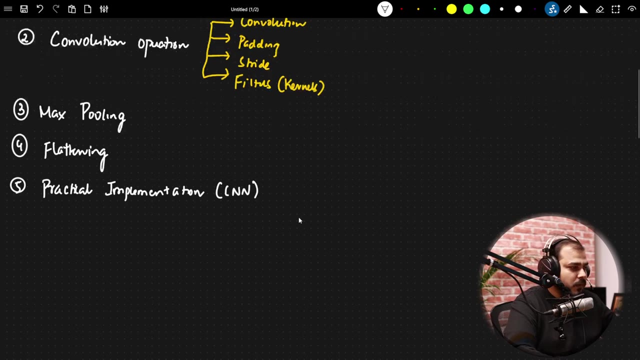 flattening. and in the fifth part we are going to see the practical implementation. okay, how do we implement the cnn? okay, practical implementation. so these all things we are going to cover and we are going to cover and make sure that we understand each and everything. okay, now this. 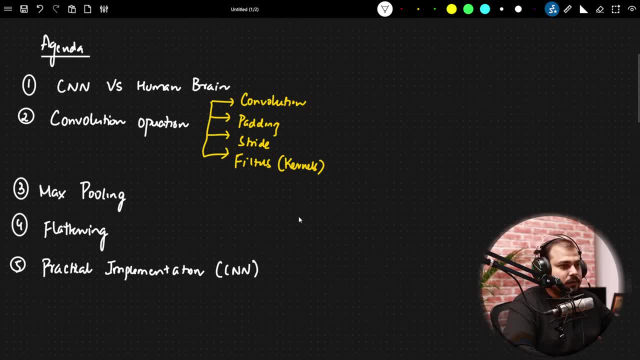 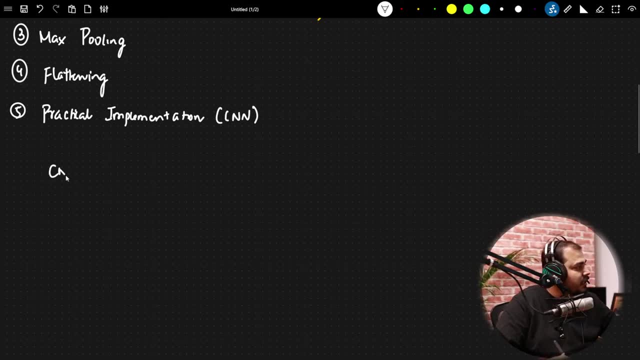 is the entire agenda of this session and we'll try to cover up all of these things. okay, and again, let's start with understanding cnn versus human brain, right versus human brain. now human brain always understand. how does it work? you know, like suppose i am seeing a specific. 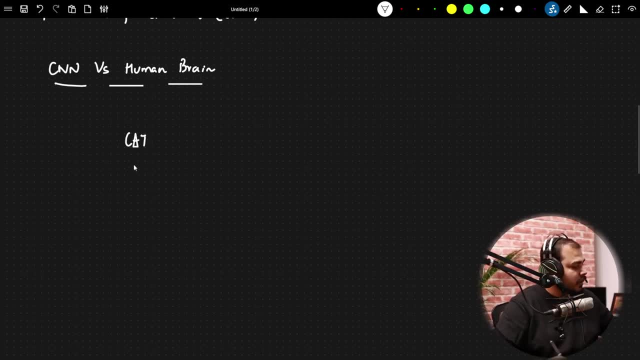 object. okay, suppose let's say that i'm seeing a cat, okay, i'm seeing a cat. or let's say in a specific image, right, i may have various objects. i may have cat, i may have dog. okay, i may have a bicycle. okay, i may bicycle. i may have a car and i may have a human being. okay, now, in this specific. 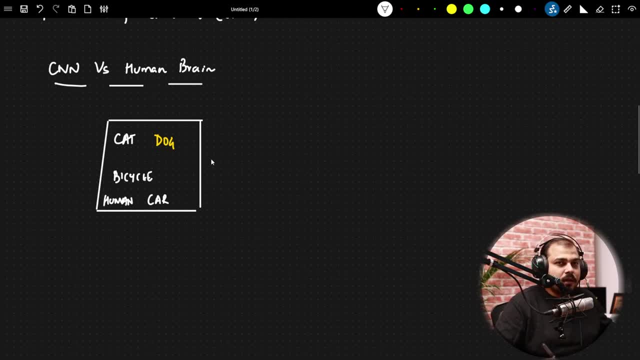 image. let's say that we have so many things over here right now specifically as a human being. right when i am specifically seeing a object, i may have a car, and i may have a human being right when i am specifically seeing a person, or i may just be seeing a human object right, let's say i. 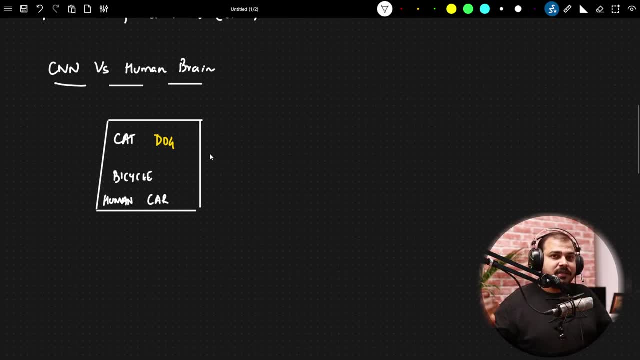 may find out many things right. i may see a person moving, i may see an animal over there, i may see a bird flying. so many details is getting processed in my brain itself, right, and because of that, because of that processing, i'm able to understand a lot of things. the major part of the brain which 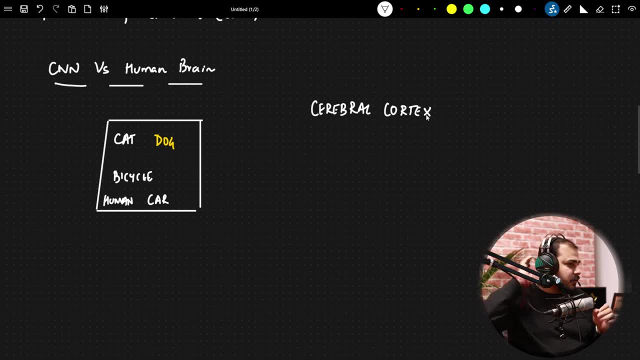 we specifically call as cerebral cortex right, the cerebral cortex which is in the backside of this, And in this part only, you know, there is a place, there is a part of the specific brain which we call it as visual cortex. okay, Visual cortex, which is specifically responsible for seeing any items that are there, any objects that are there in a specific image or in a video. okay, 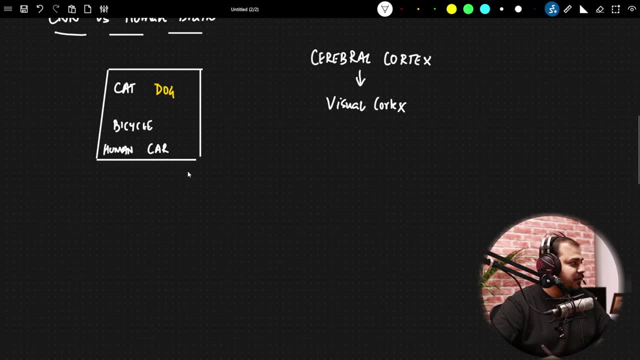 Now, this visual cortex, it may have many layers. okay, Suppose let's say that if I probably talk about this visual cortex, it may have layers like- let me name this layer at V1,, V2,, V3,, V4,, V5,, V6, and let's say V7.. 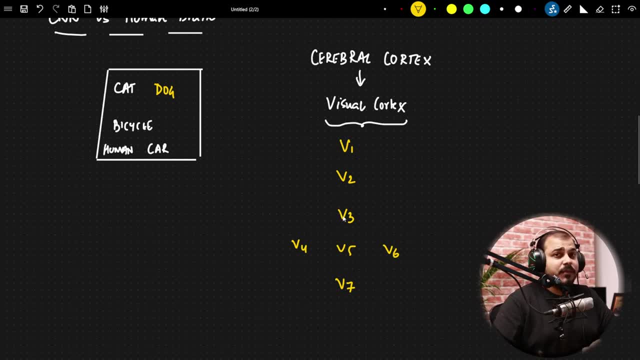 I'm just creating some layers, you know, like this, There may be many layers, but I'm just going to define some of the layers, like this. Now, as soon as this input passes through each and every layer, you know, let's say, this layer is responsible in understanding. 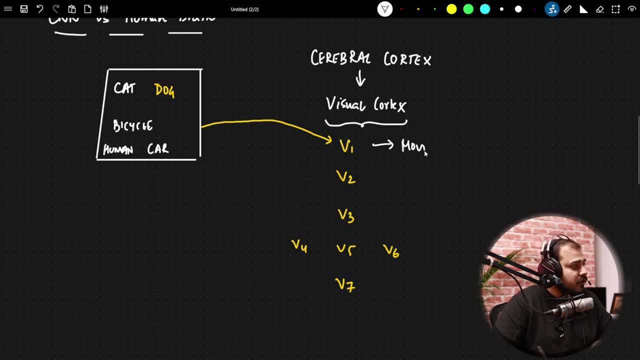 or in basically seeing the moving objects. So when it passes through this layer, we will be able to determine that, okay, fine, there is some moving object that is going up. Then when we go to the next layer over here, right, 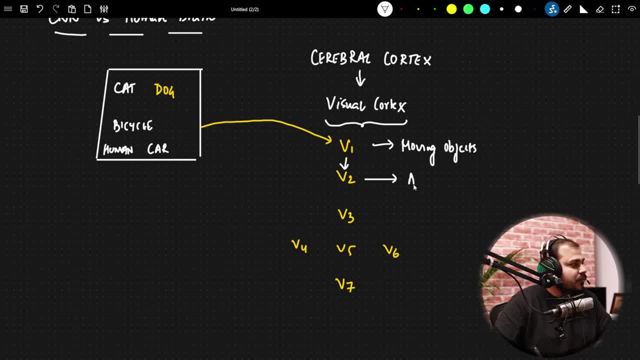 Let's say, over here we are able to understand some of the animals right, Like cat, dog or something right. So over here we'll be able to understand some of the animals you know. Then, as it passes through this layer, 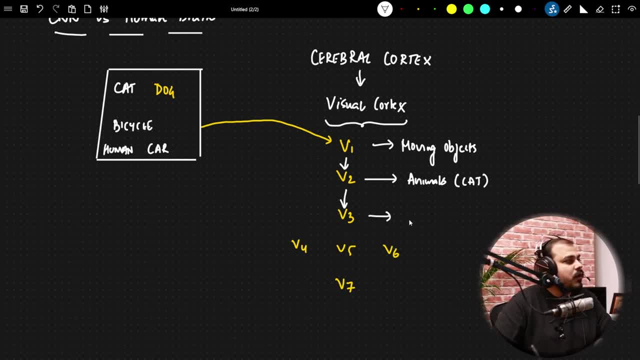 And goes to the V3 layer. let's say, And this is responsible for doing some other task, You know, here we are able to map the environment. Let's say some functionalities. map the environment. right, You are able to visualize the entire environment. 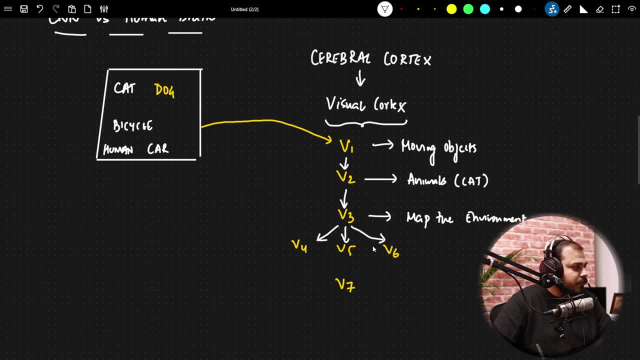 So something is happening in each and every layer, you know. And finally, all this information, when it is passed, we will be able to visualize this specific image over here in this V7 layer, which is a part of Visual Cortex. Okay, 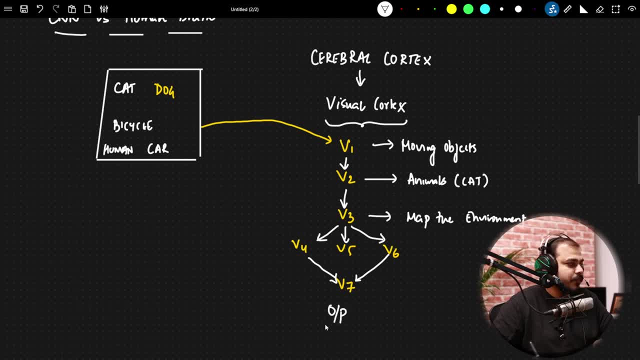 this, you are able to finally find out the output over here after so many processing, right? similarly, if i talk about convolution neural network, right, it should be also able to do this many number of different kind of processing. but now the thing rises: is that how we can make sure that? probably? 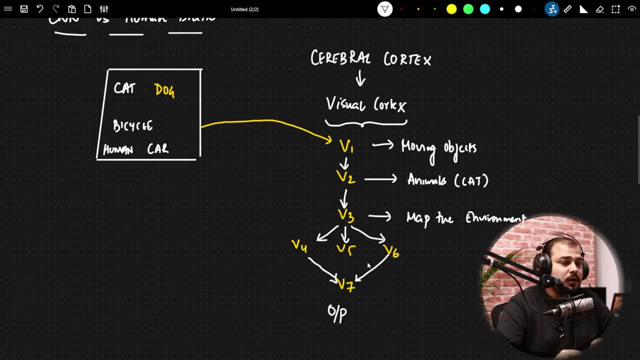 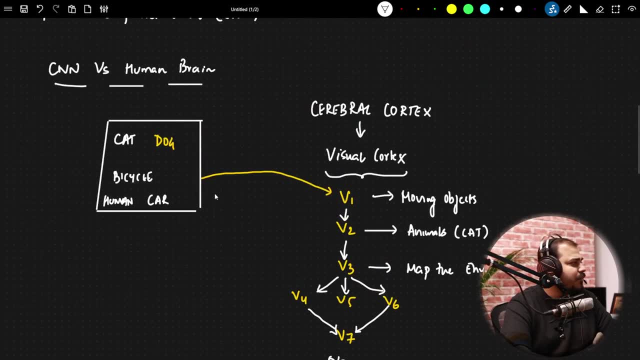 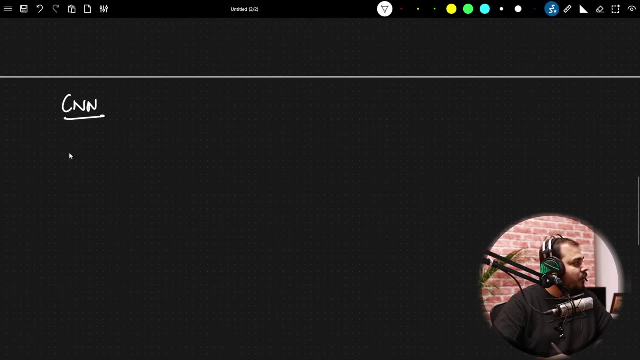 whatever cnn we are trying to develop, it should also be able to do all this kind of task. okay, so let's go ahead and understand. so, the first thing with respect to cnn. when, when i probably discuss about cnn, we will divide this into multiple steps. the first step of operation. 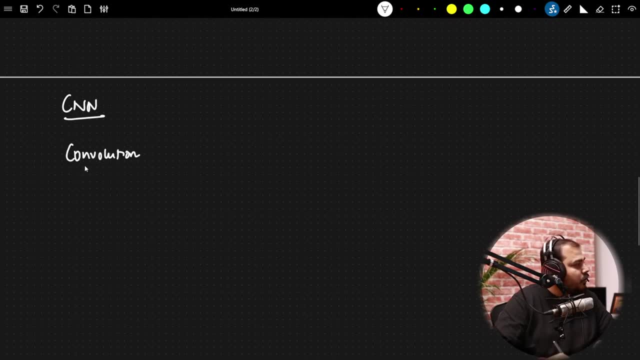 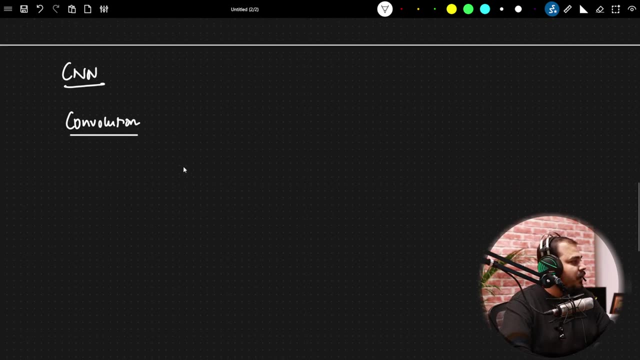 which is called as convolution. now, what exactly is convolution? before we go ahead and understand about convolution, we need to understand some of the basic information about the images, right? so what are specifically images? right? what are images? suppose you click your keyboard and you click right picture and you tick the image and you click your 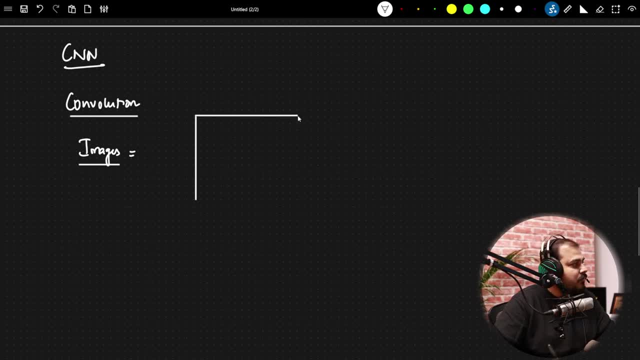 computer. you tick the image and you click your computer. and you tick the image and you click photo, right, let's say: this is your photo, okay, and it has specific, some kind of pixels. let's say, let's say that this is a photo. and whenever you have a photo, there are two types of focus. one is 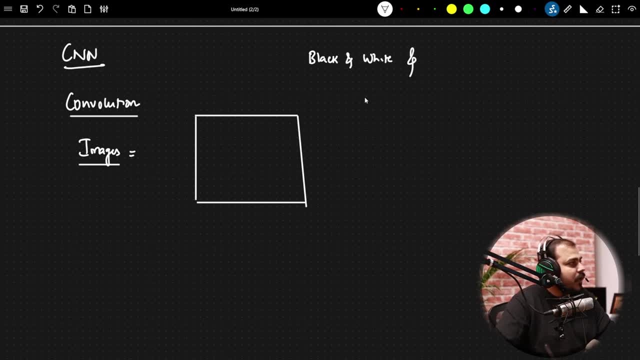 black and white, and one is rgb type and the other one is something called as rgb type. in black and white, you just have a single channel, okay? that basically means your, your entire photo will either be mostly the component of a black color or white color, something like that. okay, so here in in black. 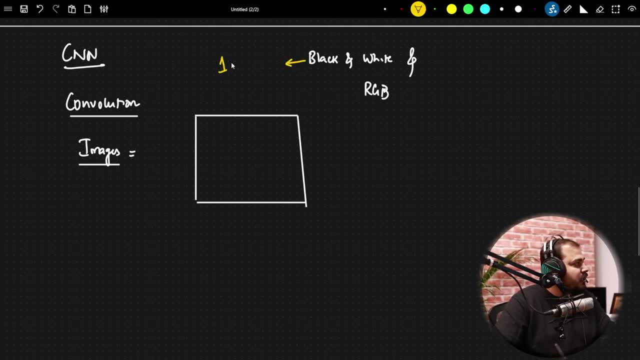 and white. in this right, you just have a single channel, one channel, okay. and whenever we divide these images, we divide by some kind of pixels. let's say, if i probably create this kind of line right, so over here let's say one, two, three, four, five. so in the width and height, let's say there. 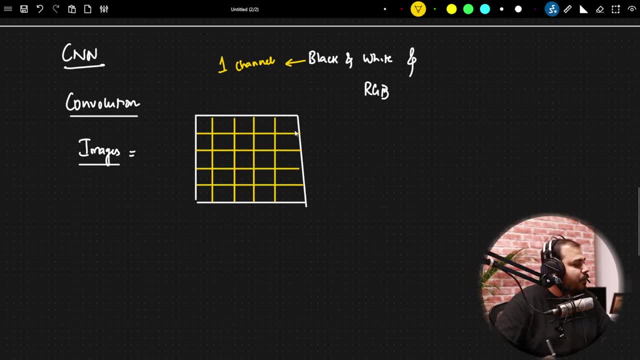 are five different different pixels. okay, so let's say, if i want to probably call this image, it will be five cross five pixel image, okay, and here each and every pixel will be ranging between zero to 255. right, if i specifically talk about mostly, zero is nothing, but it is a black color. okay, so let's say zero is a black color and 255 is actually a. 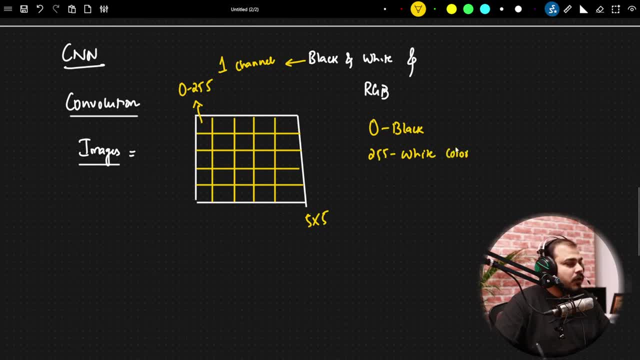 white color, let's say, okay, white color, so all these values, if your value is ranging between zero to 255, so every pixel will be a black color, so you will see white in each pixel. okay, so let's say, if i want to probably call this image, it will be 5 x 5 pixel, okay, and here each and every pixel. 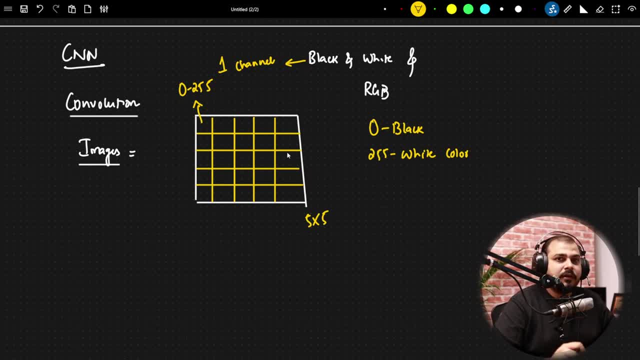 may have different, different values based on the image composition. right over here you may probably have 40, over here you may have 0. here you may have 255. here you may have 240. here you may have 17, like this. each and every values are there right, so this is basically called as a 5. 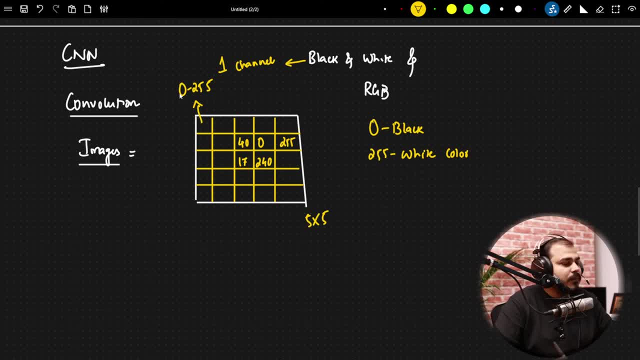 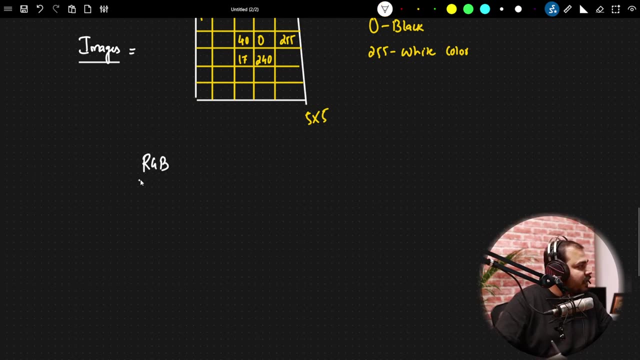 cross 5 pixel image and in each pixel your value will be ranging between 0 to 255 in a single channel. now, with respect to a RGB image, which is a colored image, okay, so suppose if I probably consider an RGB image now, how does an RGB image look like here? let's say we will be having three. 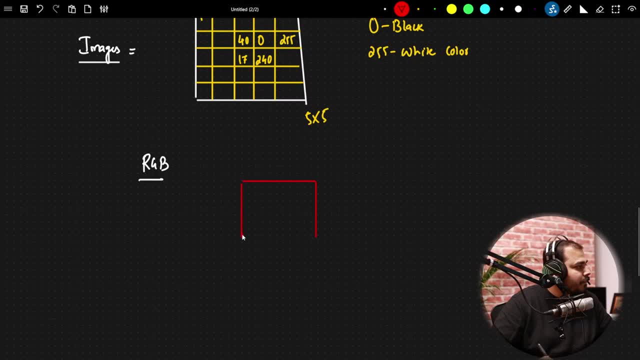 channels. one is the R channel. the R channel and this is basically the colored image. you know, whenever probably you click from your mobile phone or from some DSLR camera, you know you always get that specific image in the form of RGB format, because every color combination can be created with the help of this RGB image, that is. 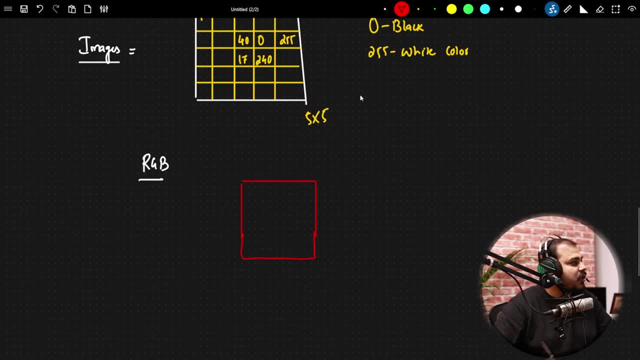 red, green, blue, right. so suppose let's say this is my R channel and with respect to the other thing, I may also have green channels. suppose this is my green channel, so I may create something like this: this is my green channel, okay, this is my green channel, okay. 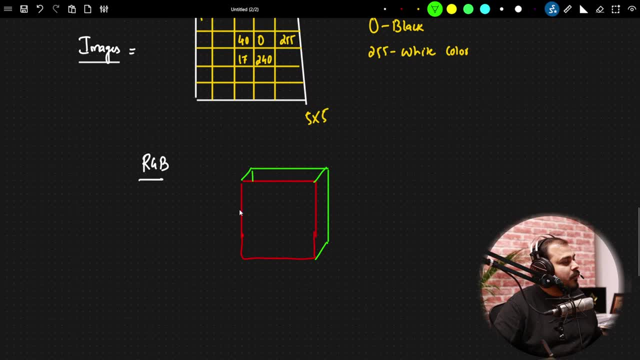 so this is my green channel. let's say, okay, and on top of it you may also have another channel which is like a blue channel. so suppose I go and pick up blue color. let's see where is blue color somewhere like this, right? so this is my blue color, so this blue will be another channel, right? 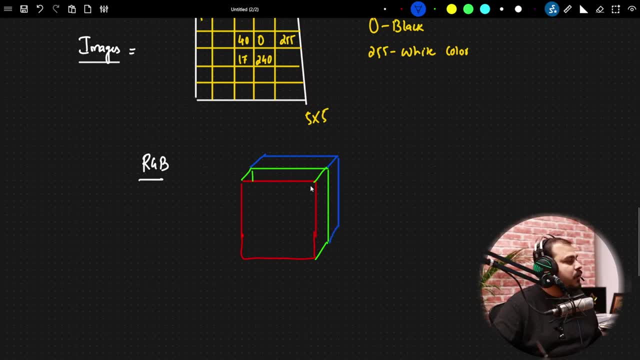 so whenever I have this kind of combination, then what will happen over here? let's say this is 5 cross 5. let's say this is 5 cross 5: 1, 2, 3, 4, 5. let's say this is 5 cross 5: 1, 2, 3, 4, 5. let's say this is 5 cross 5: 1, 2, 3, 4. 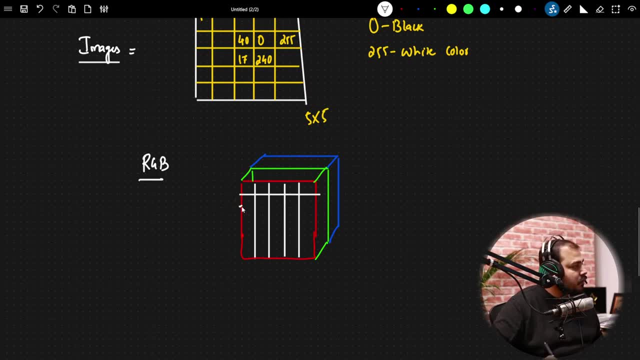 5 right, and similarly I have 1, 2, 3, 4, 5 right. so whenever you have this 5 cross 5 pixels, here also it will be 5 cross 5 right. so any image that you are going to take is that you're going to combine. 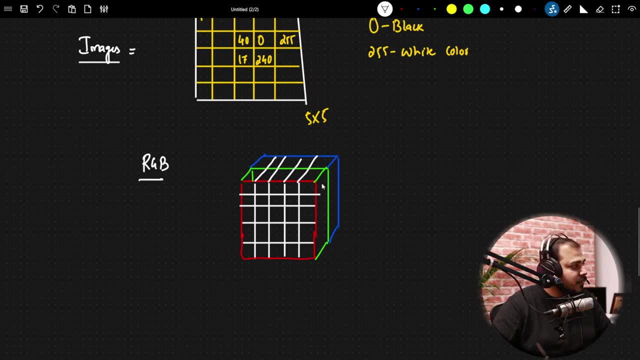 this RGB. right, this will be our channel, that is red channel, this will be a green channel, this will be a blue channel, and when it combines, it can basically come up with some kind of format. okay, and here also, your values will again be ranging between 0 to 255 with respect to each and every channel, and when you combine them, 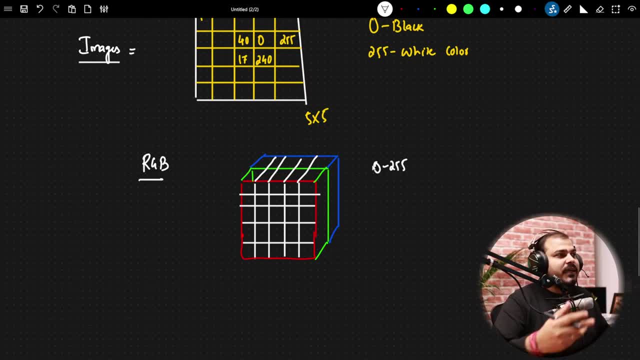 then the combination that you are actually going to get, you will be getting it in different colors, okay, so this is with respect to RGB format, and suppose, if I want to represent this in the form of pixel format, I will basically write 5 cross, 5 cross, 3 channel. okay, because they are three. 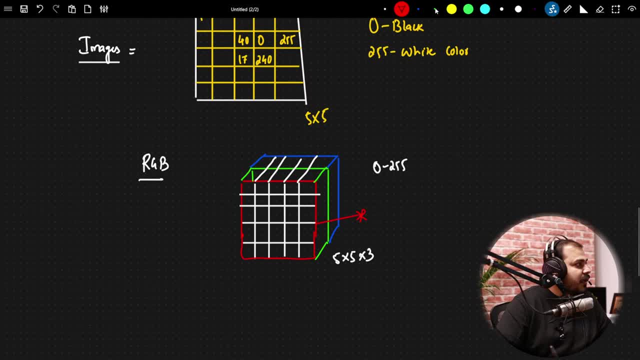 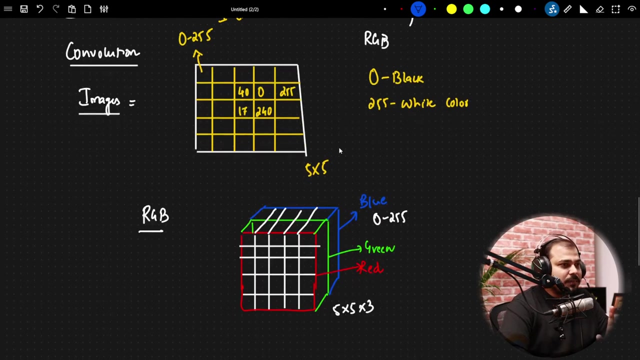 channel, this is my R channel, this is my green channel and this is my blue channel. right, so red green, blue, red green, green and blue channel. okay, so these are my red, green, blue channel. so I hope I I you got the difference in understanding the black and white image versus the RGB image. okay, so this is the basic information you really 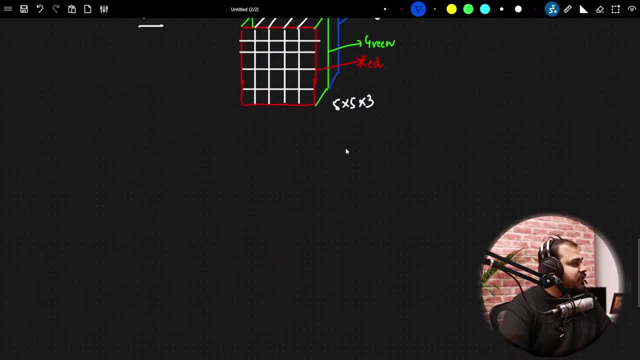 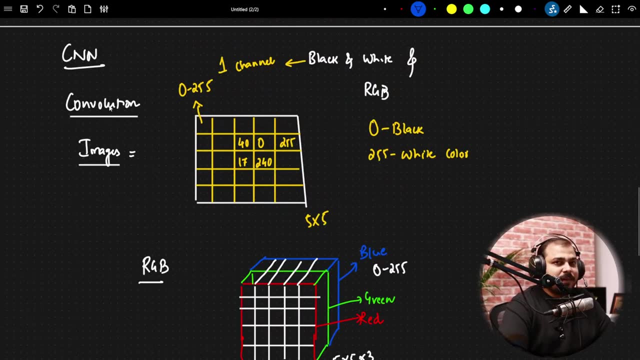 need to understand. okay, now, if I go to the next step, let's let's talk about this convolutional layer. so what exactly happens in a convolution layer? and later on I'll show you an example with respect to a single black and white image and also with respect to a RGB image. so if I go over 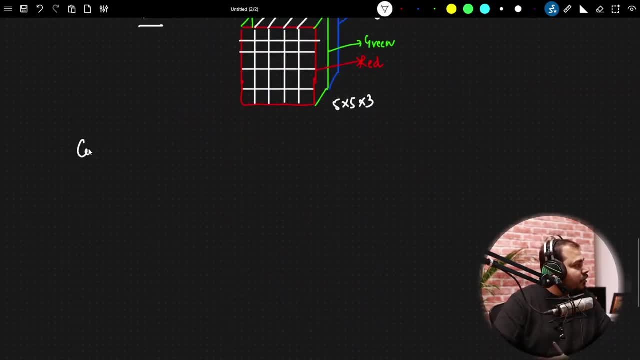 here and probably take up this convolution operation. now, in convolution operation, what happens is that- and this is the first step with respect to a convolution neural network, let's say you have an image, and this is my specific image, and here I have values. let's say how many number of channels I have. okay, so let me just create this three, four, five, six, right? 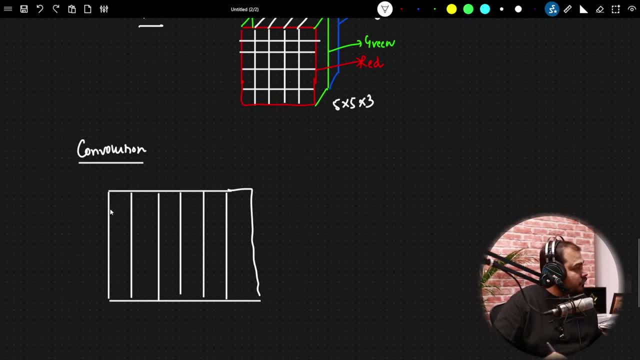 so here also, you have one, two, three, four, five, six, right? so this is my six cross six image. okay, six cross six image. now, when this is basically a six cross six game age, what we are actually going to do is that we are going to pass it through a filter, okay. 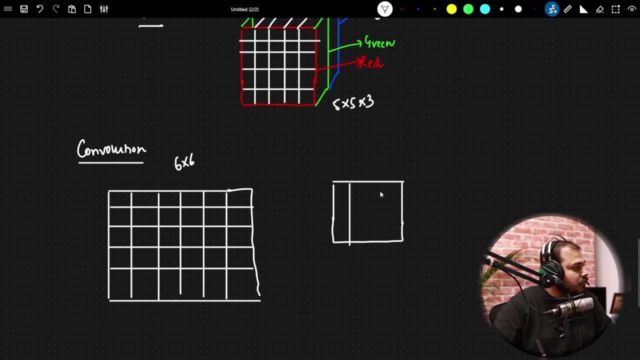 we are going to pass it through a filter and this filter will be 3 cross 3. let's say 1, 2, 3. right, let's say that this is my Strix 3 cross 3 filter. here you can see this as filter also, or this s: 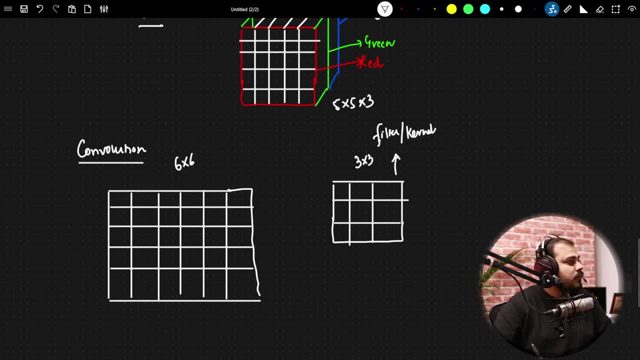 kernel also. okay, this has filter on, this can schedule also and finally you get some kind of Output and let's say that this is a 4 cross 4 output. I'll tell you why we are getting a 4 cross 4 output, Why you are getting a 6 cross 6 output and all. 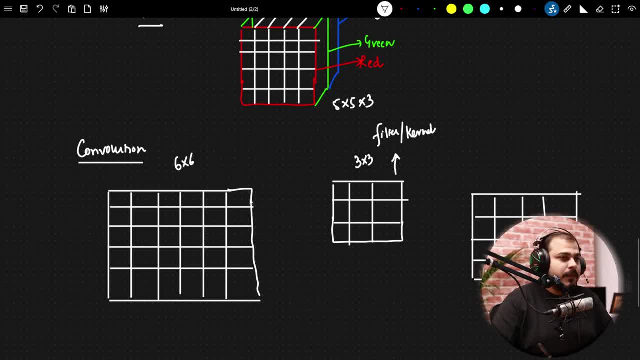 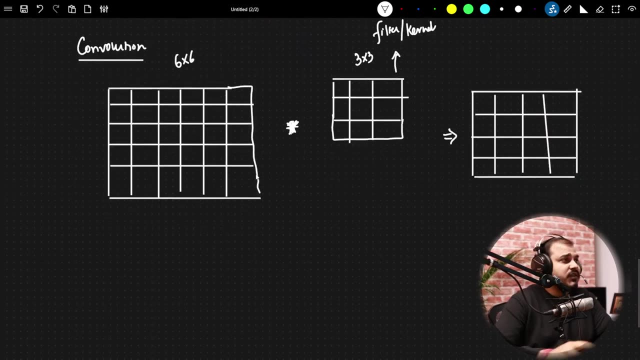 2, 3, 4,. okay Now, whenever you do this convolution operation, convolution, let's say we are doing this kind of symbol, We are getting and we are getting this specific as an output. Okay now, Let's say This is my 6 cross 6 image and let me put some values. you know that. 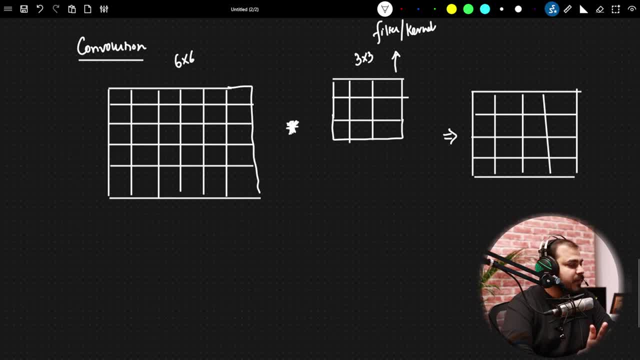 Whenever we try to put some values with respect to the image pixels, you know that it will be ranging between 0 to 255,. right Now, in convolution, what we do is that if I really want to convert this into 0 to, let's say that this is my values. 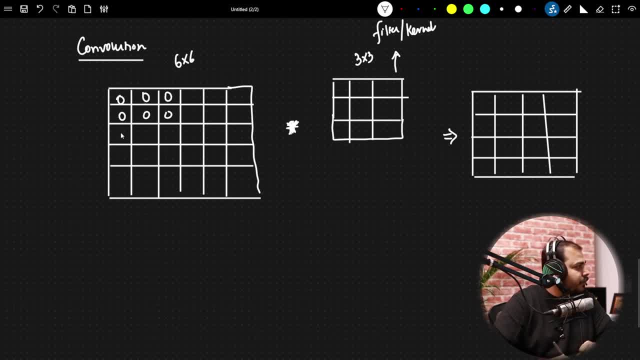 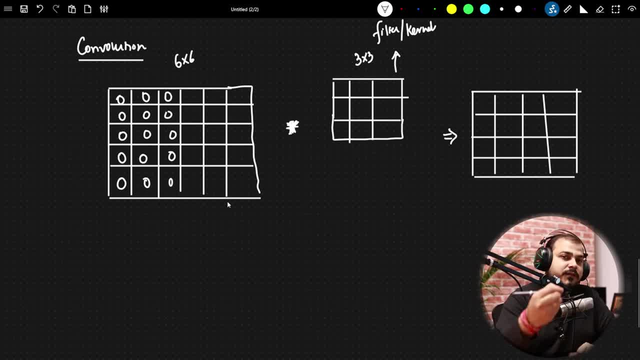 Let's say, and these all are 255. Okay, always remember, the first step that we do in a convolution is that we try to bring this all values between 0 to 1. Okay, if I'm trying to bring this values between 0 to 1, then what it will happen. 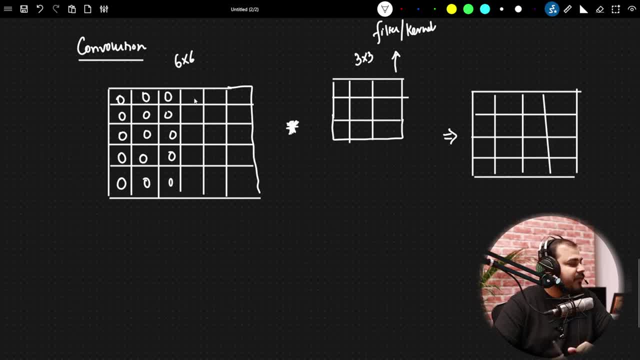 I will divide each number by 255.. So over here, if 255 is there, I'll make sure that this all will get converted to 1. This we basically say it as min max scaling. Okay, min max scaling. So this process is actually called as min max. 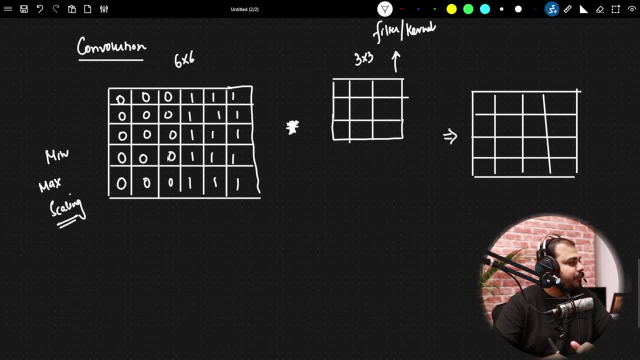 scale: Okay, min max scaling. now, in min max scaling, what we are doing is that we are just trying to convert all the values of the pixels Between 0 to 1.. Okay, super important, and this is the step that we are also going to see. 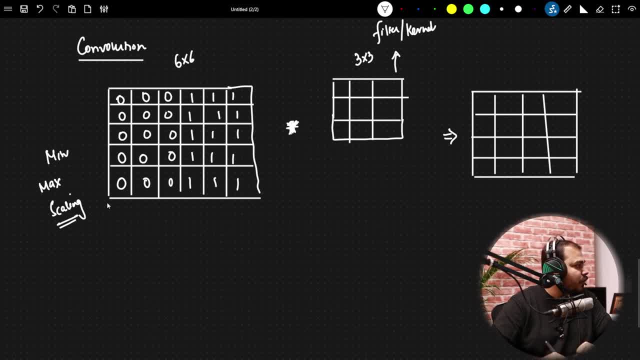 Okay. so here you can see: 1, 2, 3, 4, 5.. Okay, one more value. I will just have one more row. I will just try to put it over here, So this will be my lines: Okay, 0, 0, 0, 1, 1. so 1, 2, 3, 4, 5, 6, okay. 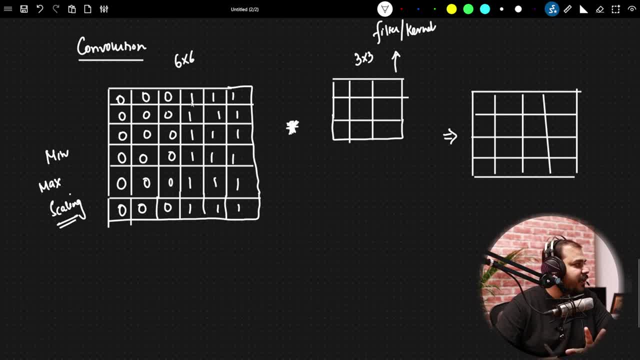 and So you have actually got this much idea that what I have done is that my first step. I've done a min max scaling, So whatever pixels are there, I'm going to basically convert this into 0 to 1.. Okay, Let's say that I have a specific filter over here, and this filter what I am actually going to. 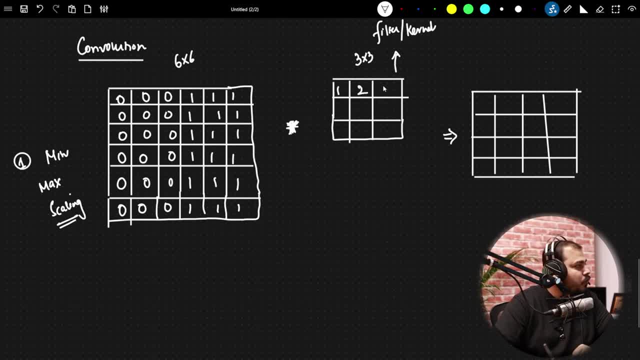 Put the values like is that I will just write 1, 2, 1.. I'll talk about it. Why I am putting this passive filter like this: 000 minus 1 minus 2 minus. Let's say that I have put this specific filter. This filter is actually called as something called as horizontal. 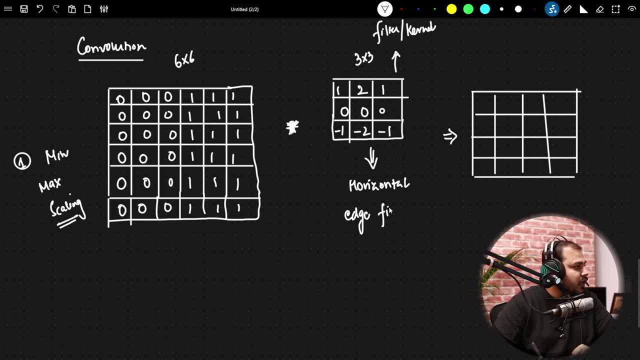 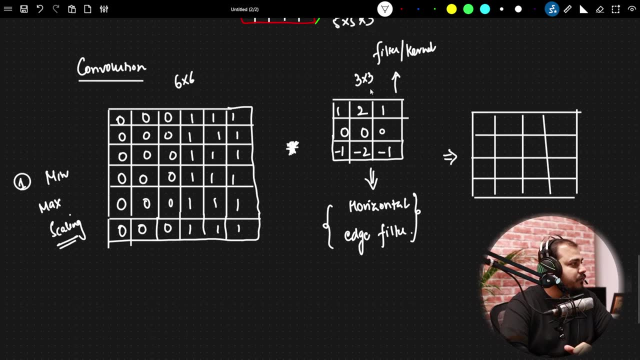 edge detector, a Horizontal edge filter. Let's say I'm just saying this as horizontal edge filter. Now, I hope you have got an idea with respect to this. So what I have done is that I have given 6 cross 6, I image, have passed it through a convolution filter. Sorry, I passed it through a filter which is 3 cross 3 with this values. 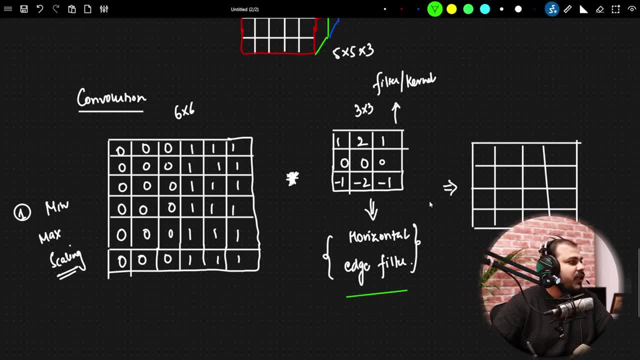 Which I specifically say this as my Horizontal edge filter, and finally, the output that I am actually getting. I'm getting it over here and this is actually 4 cross 4, Okay, and this is specifically my output. Okay, and What kind of output we will get, that I'll try to discuss. Okay now, 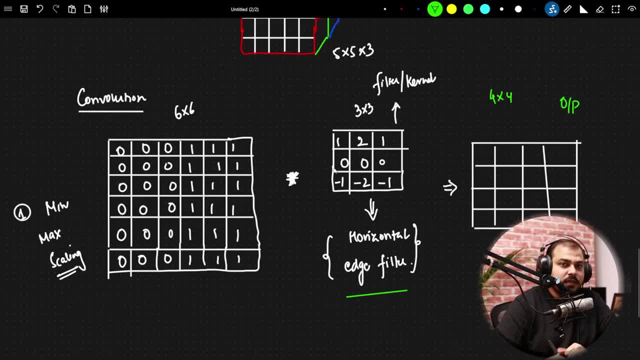 Let's try to understand how this convolution operation happens. Convolution operation: what it says is that I will take this filter and I will just place it in top of top of this Specific image from left. from the starting, let's say that I have taken this filter and I am placing it over here. 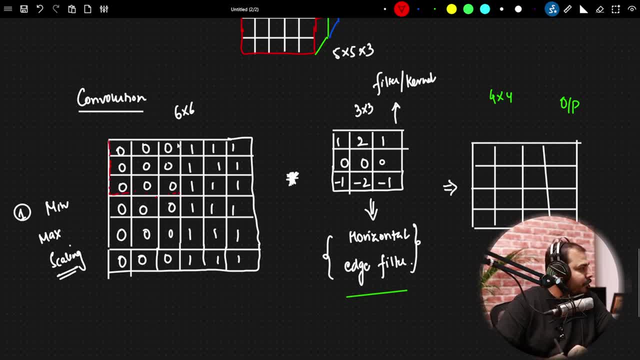 So I am placing it like this, I'm placing it like this on top of it, I'm placing it over here and top of it. now, when I place it over here, When I place it over here, what will happen? what will happen? the first operation that I am actually going to do- 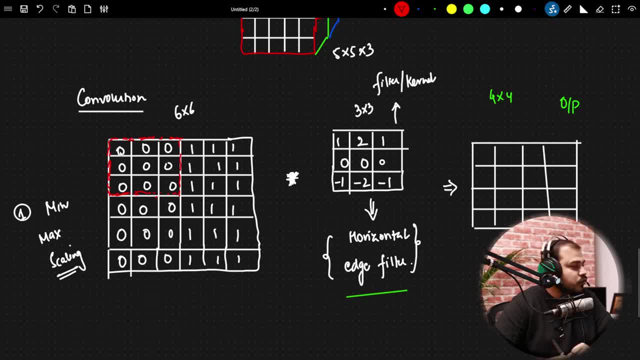 I will take this value and wherever it is placed to that same same row or Same cell. right, suppose this cell is there and I've actually put this 3 cross, 3 filter over here. So over here, this value and this value will get multiplied. So if it gets multiplied it is like 1 multiplied by 0. 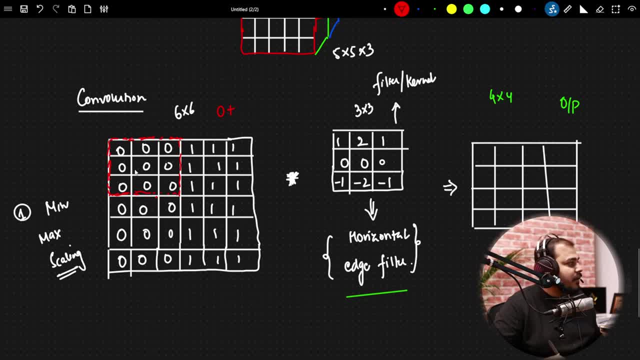 So I'm going to get 0. okay, Then I am going to add the next value, So this value will get multiplied with this, so this will also become 0 and similarly, 1 will also become 0 and like this, all the values will become 0 in the first instance, when I am placing this specific filter and 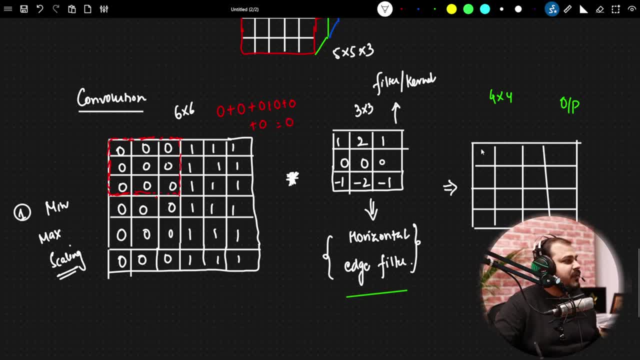 And whenever we add up this value, whatever is the final output, we will place it over here. okay, So this is the first operation. So I hope you are getting a clear idea about it. okay, So what we are doing over here, we are just place this convolution filter, this filter or kernel, on top of it. 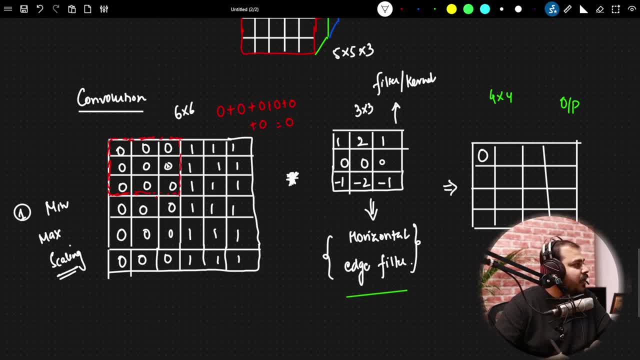 We are multiplying each cell with that cell, and then we are adding up all the values right Now. after this, what we do is that we move one step to the right. We move one step to the right. Whenever we move one step to the right, there is a variable which is called as stride. 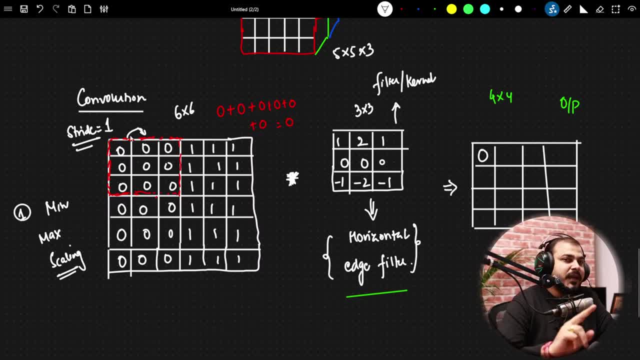 We specify the stride variable as 1.. If you are jumping two steps to the right, then we will basically make stride is equal to 2.. But here we are jumping just one position to the right, So one position to the right, the stride will be 1.. 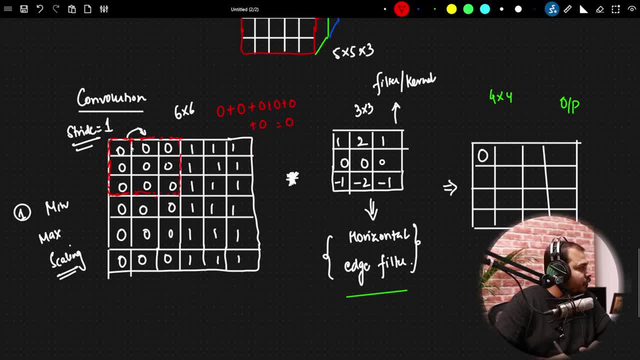 Now what will happen? My filter, this filter will start moving from here to here right Now. when it moves from here to here, then what will happen? Again, Do the calculation. My calculation will start. 1 multiplied by, let's say, my calculation will start for the second instance. okay, 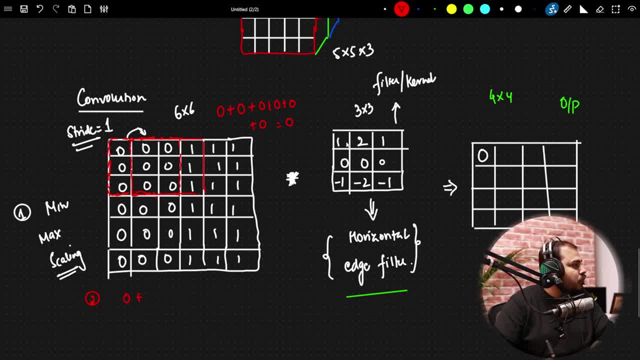 1 multiplied by 0.. So it will be 0 plus 2 multiplied by 0.. It will be 0.. 1 multiplied by 1. So it will be 1 plus 0 multiplied by 0.. It will be 0.. 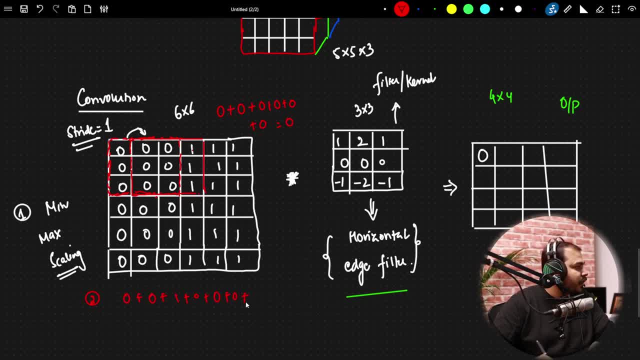 Then again 0, 0. Then over here. if we go over here it will be minus 1, minus 2.. This both will get multiplied and to this also It will be 0, 0. And finally I will have minus 1 multiplied by 1.. 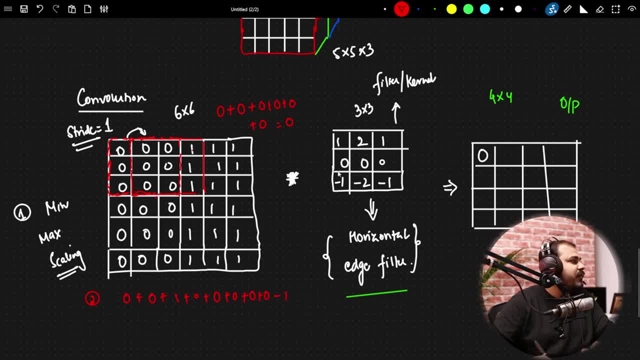 It will be minus 1, right, So here also what I will be getting. My total value will actually be 0, okay, So I hope you are getting an idea about it, Then, what we will do. We will again jump one step to the right after this, because I have to go and take the next pixel of the information over here. 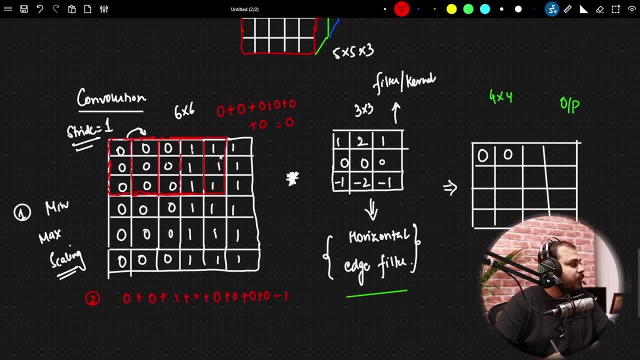 And here we go with respect to this. Now, when I jump one step to the right, then what will happen Over here? like I will be jumping at this position to this position And again the same operation will happen. The third operation: again, if you try to see, everything should be equal to 0, most probably, because, see, if I multiply this so 0, then this will be 2, then this will be 1, then all will be 0 over here. 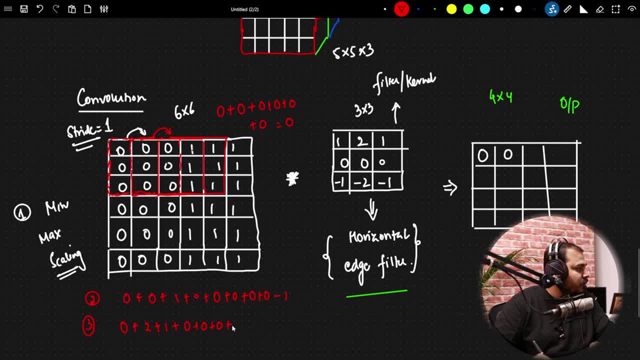 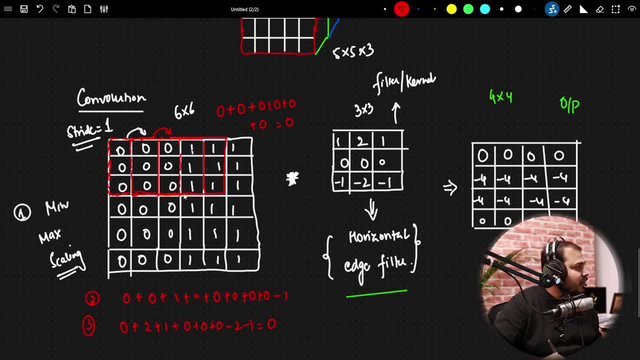 So that basically means, after we finally go to the next step, then my next trade will move towards this position and again it will do the calculation, again I will get jump. It will become 0 over here. and after this, what we do? we go one step towards downwards. 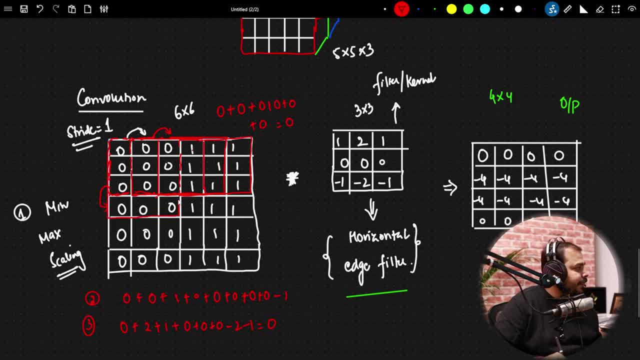 So from here to here will be my next step, and we will continue this particular step from here, and then we will do the calculation Here. you will be able to see that I will be able to get minus 4 for the same thing. 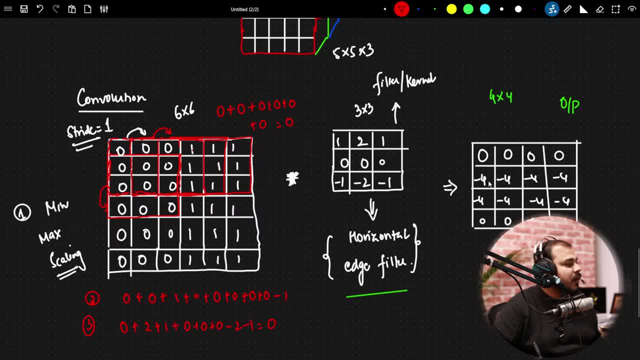 Okay, So I hope you are getting an idea about it and you are able to understand some kind of calculation that we have actually done over here. Okay, So this is very much clear till here, I guess, And you are able to understand things. 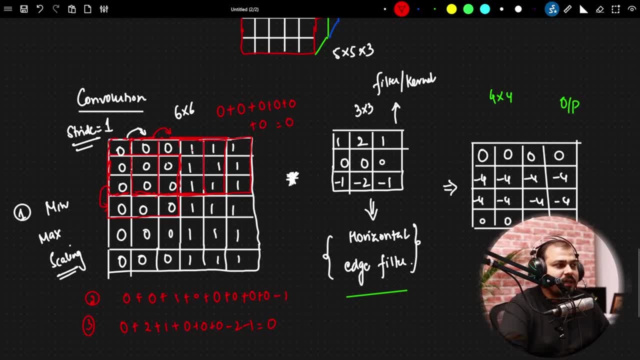 Okay, And definitely you can do this entire calculation and you can try to find out. Okay, So if you move one step towards down, then again one more step. if you move towards down and if you do the calculation, you will be getting some values like this: 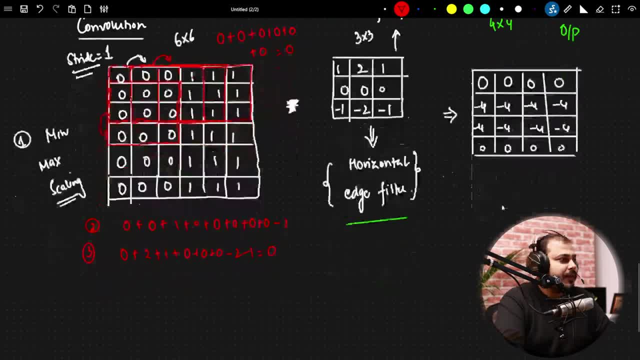 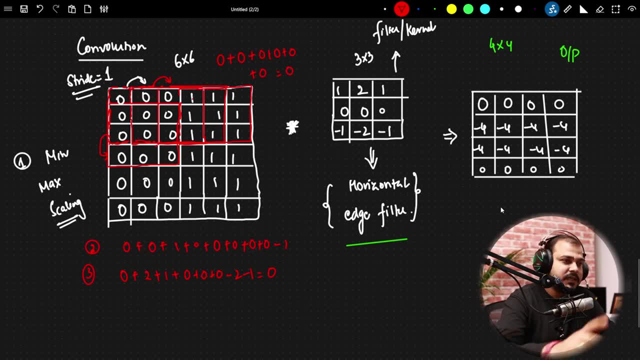 Let's say that I have got the output, which looks like this: Okay, So I hope everybody is clear with respect to this specific output and you are able to understand. Is it clear? everyone? Yes, still here. Can I get a quick yes, if you are able to understand till here? 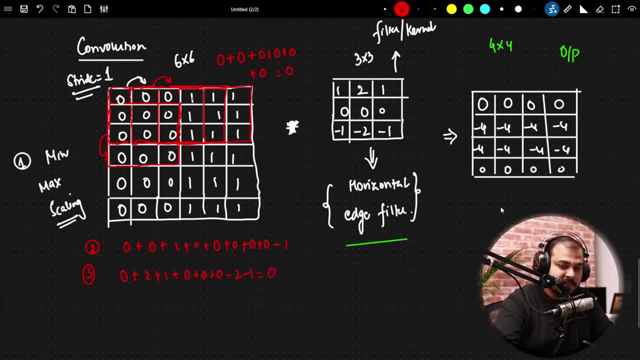 Okay, Yeah, You are able to understand guys. Just give me a quick yes, Yeah, Everyone, Yes, Okay, Perfect. Let's say that I have got this specific output. Okay, Now this operation is specifically called As convolution. 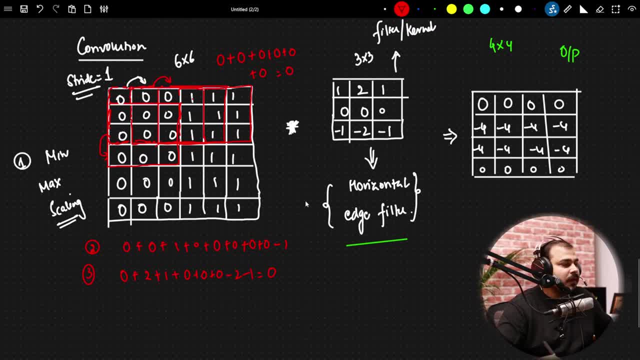 Okay, This operation is specifically called as convolution. Now, whenever we are giving filter can be one more thing, guys, filter will talk about it. Right, I have just initialized a horizontal edge filter. Okay, Now, let's say that when we got this specific output, one thing that you see over here- I am just going to rub this. 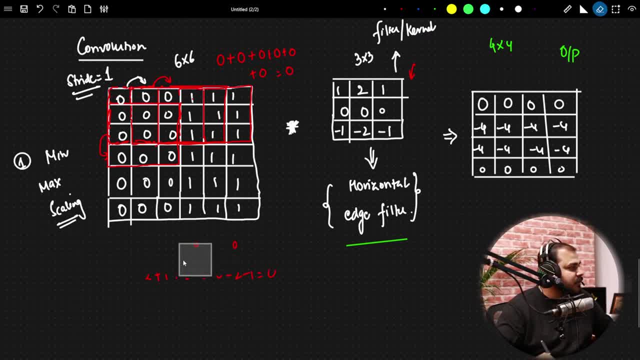 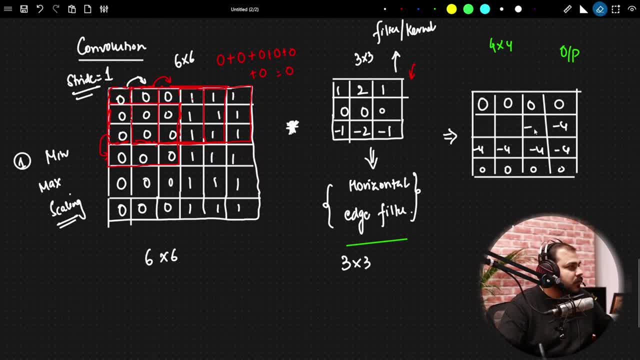 Okay, Let's say this also: I'm getting it as zero. Okay, Let's say that I'm getting this values, As if I do this operation, then automatically this will become zero. Uh, this will also become zero. Um, this will also become zero. 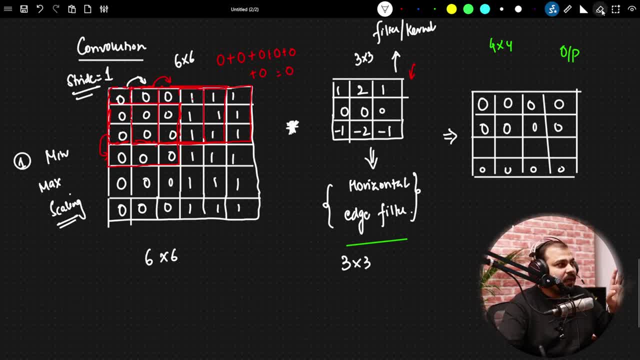 See, do the calculation. Okay, Whatever value you get, Okay, Let's consider- I'm just saying that- okay, let's consider over here that I'm getting this values. Let's, let's just imagine: Okay, I'm getting this values. 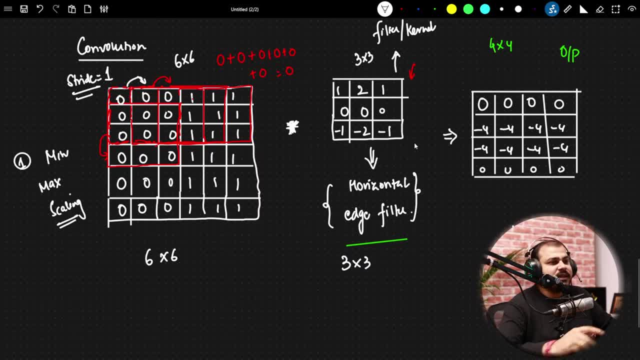 Okay, I'm getting this values by passing through this. Let's, let's just consider. Okay, I know this value will become zero or it can be anything else, you know, let's consider. I'm just saying that let's consider okay, because I want to give you a very important point by putting this: okay, uh, how, uh, we will be getting minus four or whatever values you may be getting. okay, or do one thing. if you don't want to do, go ahead with this. you know, change the filter. 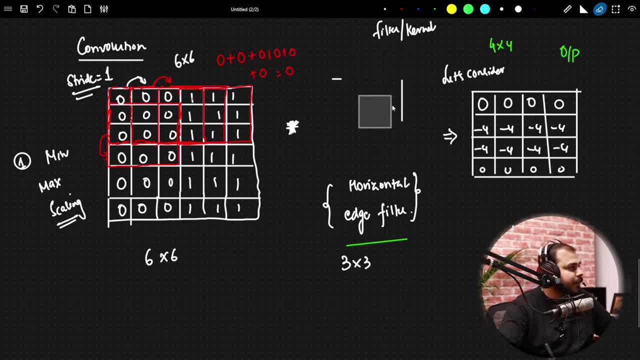 Okay, What I will do is that I will try to make a new filter over here. Okay, Let's say that I've got this new filter. okay, and let's say this is my three cross three matrix, okay, and uh, let's me see they say that, okay, I have this specific filter, minus one. minus two. minus one. okay. so let's say I have this specific. 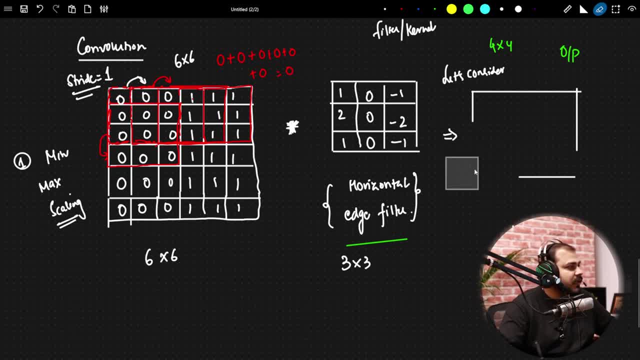 filter and let's start the operation from again. Okay, Let's say, and this filter is basically called as vertical edge detector, Let me just drop it. Okay, And let me pass this filter. Now, when I pass this specific filter, and I will be getting a four cross, four output. 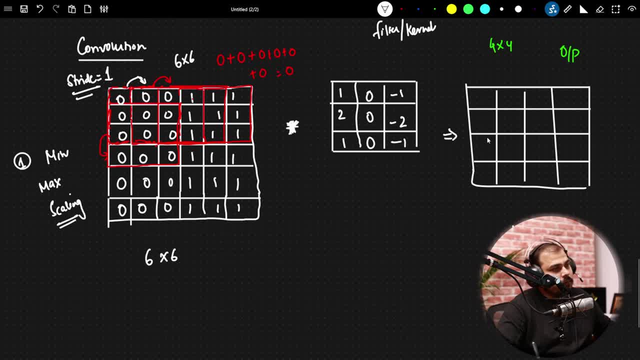 Okay, One, two, three, four. Okay, Now do the calculation: Everyone. What will happen? first time? Everything, Okay, Okay, Okay, Okay. So this will become zero, Right? Second time: Uh, if I go one step to the right, then it will become minus four minus one, minus two minus one. 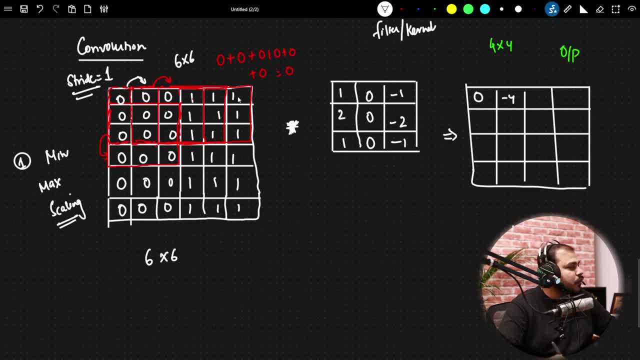 When I add this up, it will become minus four. Then again, when we go to the one step to the right- Okay, Then then again I'll be getting minus four, and then this will become zero, And similarly, this will happen for every row. 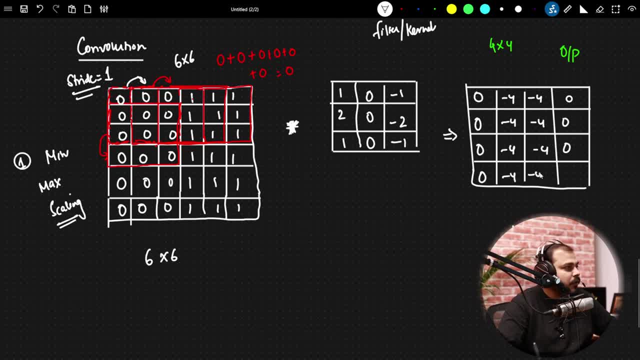 Just do the calculation and let me know whether you are able to get it or not. Okay, So this kind of values we are actually getting, Okay, Okay, Okay, Very simple. When I place from here, I go one step towards the right. 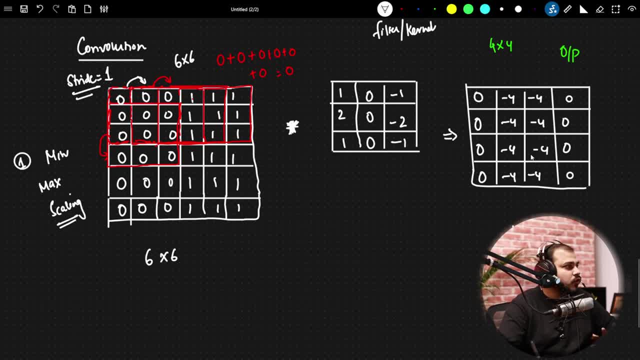 Similarly, I go one step towards the right and I do the convolution operation, You'll be able to get this. Okay, So this is basically called us vertical edge filter, edge filter or kernel. Okay, So this is my vertical edge filter occur. 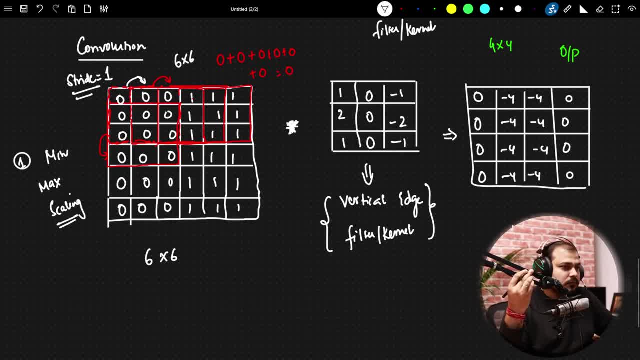 Okay, So I hope everybody's able to get this. Okay, How to choose a filter, values and all. I'll just explain. Let's say that there is This specific filter, which is already defined, and whenever I pass this filter to this, I'm 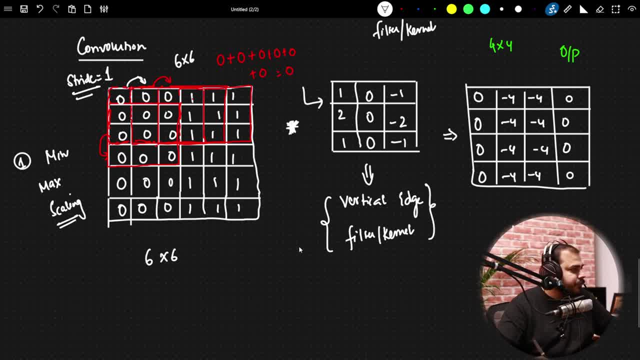 going to get vertical edges some or the other way. Now one very important thing with respect to the output. you know that if I again rechanges values- because you know that we had done feature scaling over here- right, If I do back I, if, if I revert back the feature scaling, then what will happen? 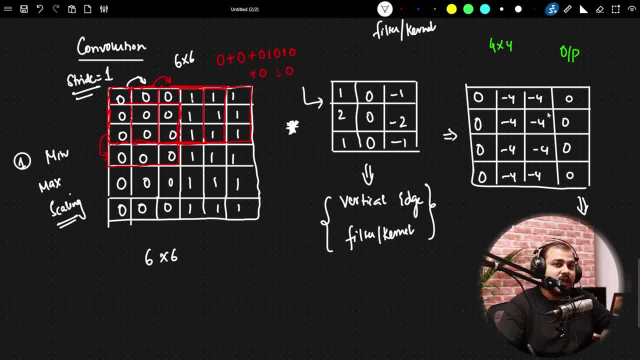 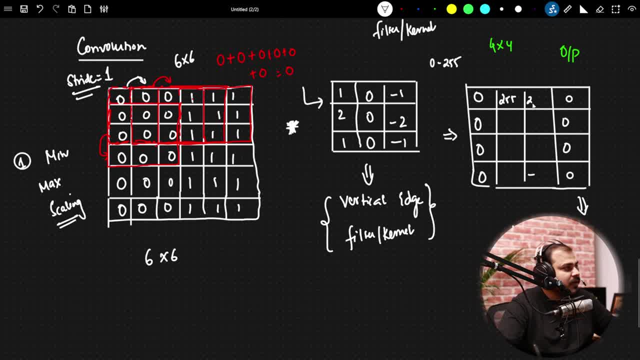 We'll actually become two: 55.. I hope everybody agrees that. right, This will become two: 55.. Sorry, This will become zero. right, This will become zero. Why? Because this was minus four. The lowest value will get converted to zero. 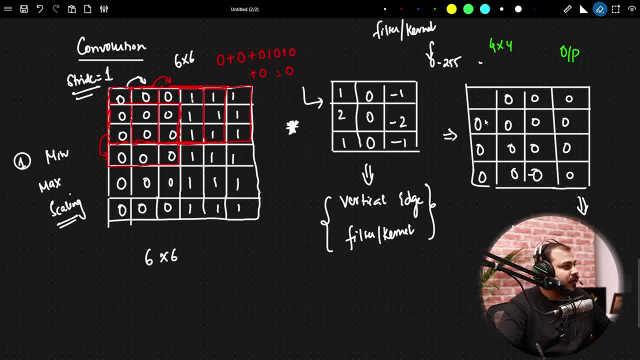 And the highest value will get converted to two 55.. I hope everybody remembers this, how we did feature scaling right? So this will entirely become this will entirely become two 55.. Okay, So if I do back the feature scaling, this all will become zero and this will become two 55, because the highest value was zero and the lowest value was minus four. 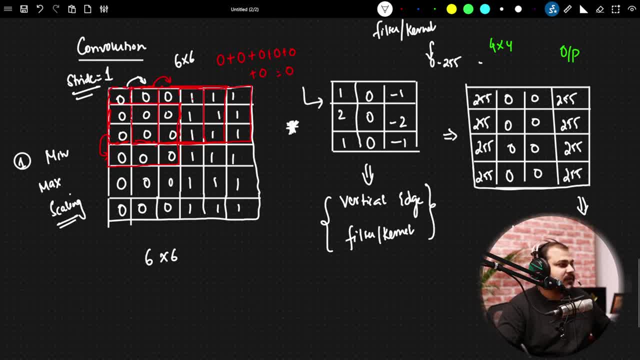 So if we bring back the min max scalar, if we apply the min max scalar again, what is going to happen? The smaller value will become zero and the larger value will become two- 55. Now, two 55 is nothing, but it is a white color. 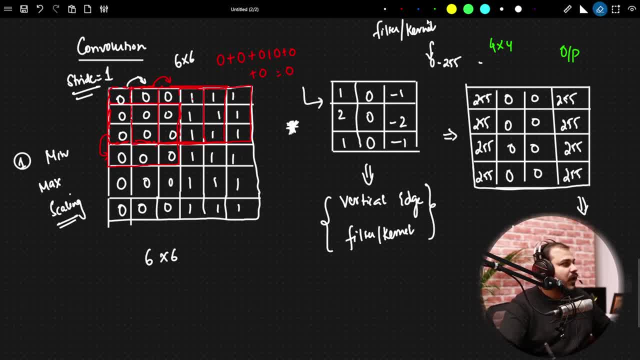 Two 55 is nothing, but it is a white color, right. So I hope everybody knows about it. So two 55 is nothing but white color, right. And zero is nothing but black color, Right. So two 55 is nothing but white color. 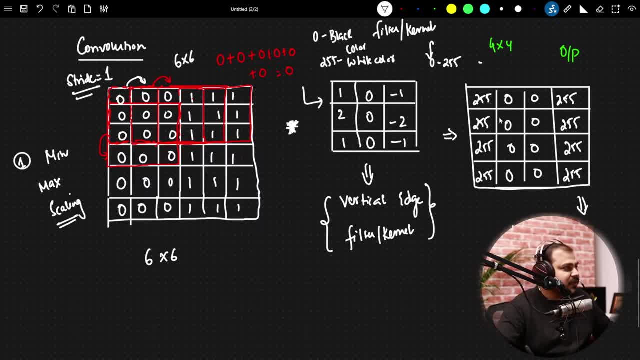 So I hope everybody knows about it Now, when I have this, that basically means this entire thing is black color, right Zero, and two, 55 is white color. So how do I get this If I probably try to draw this in the form of a diagram, right? 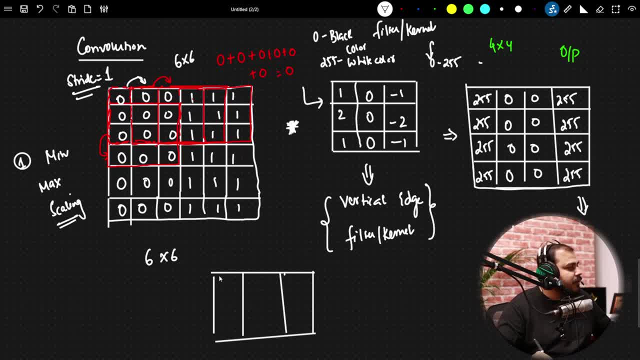 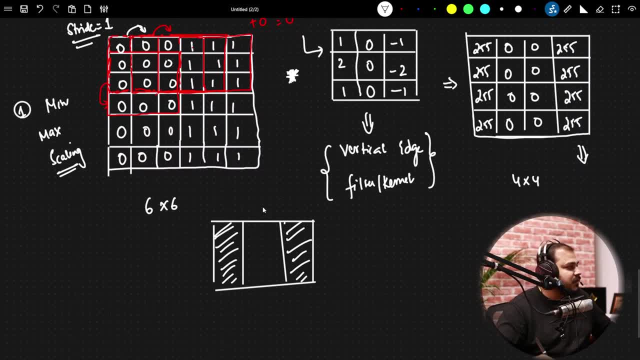 It will look something like this: So this will be my white color and this remaining all will be my black color. So this will be my white color and this will all be my black color, right? So this is nothing, but this is my vertical edge. 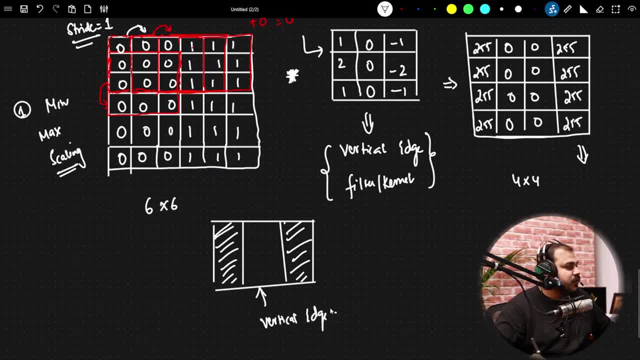 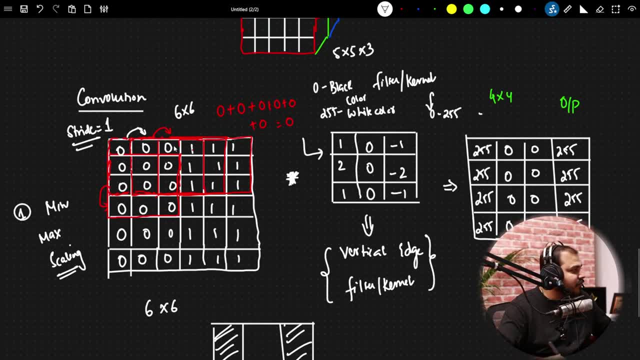 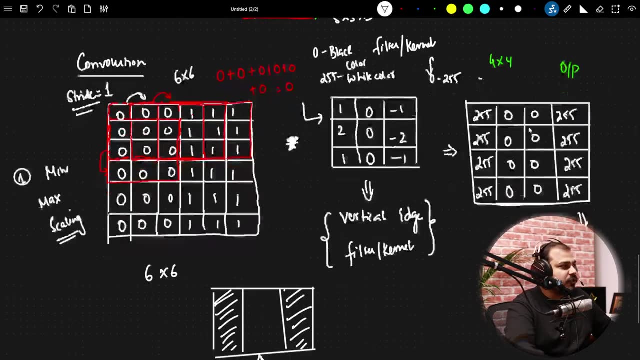 Vertical edge. So in this specific image, so in this specific image, you know that zeros and ones are there. Obviously, I should be getting a vertical, I should be getting a vertical edge. in between that and after passing this filter, I am able to get a vertical edge that you can see from. 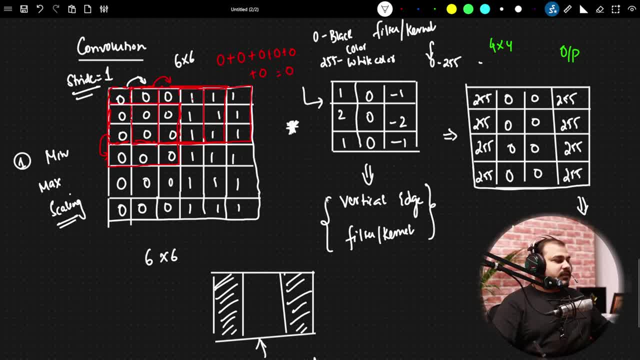 here, right From this specific example, And this filter is responsible for doing that. It is responsible for getting the vertical edges right. So from here you can see, As soon as I pass this filter, I'm able to get the vertical edges. 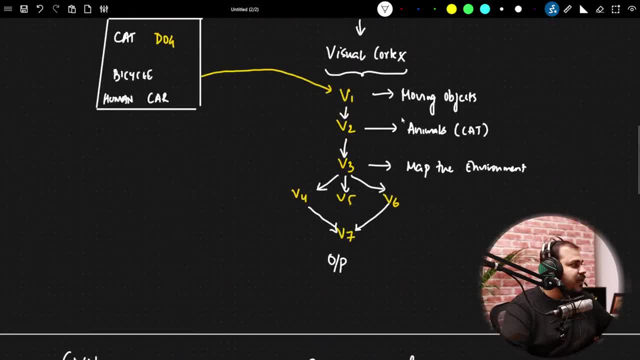 So what does this basically mean? Here I discussed about my various layers right: V1,, V2,, V3,, V4,, V5,, V6, V7.. Similarly, we have created a layer over here which is able to extract some information. 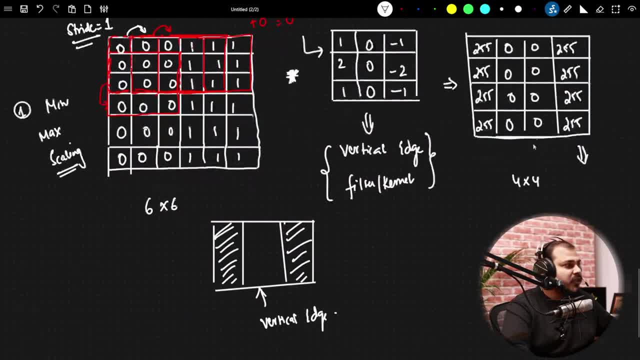 Now, in this particular case, with the help of this filter, I'm able to extract where are my vertical edges right. So this process is basically called as a convolution operation. Similarly, I may have- Let's say it's different- kind of filters. 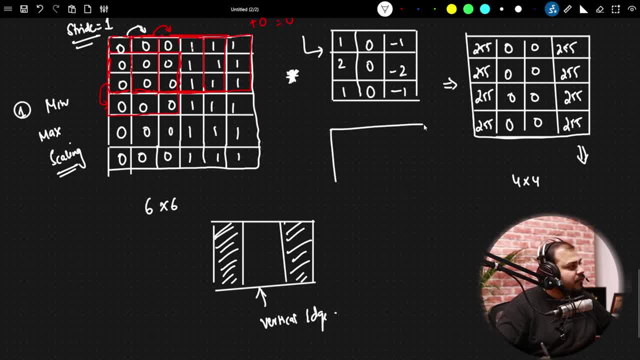 I may have a horizontal filter. I may have another filter like this, And this filter will be also 3 cross 3,, let's say, And this will be able to determine my horizontal edge. There will be one more filter, let's say, which will be able to determine my round objects. 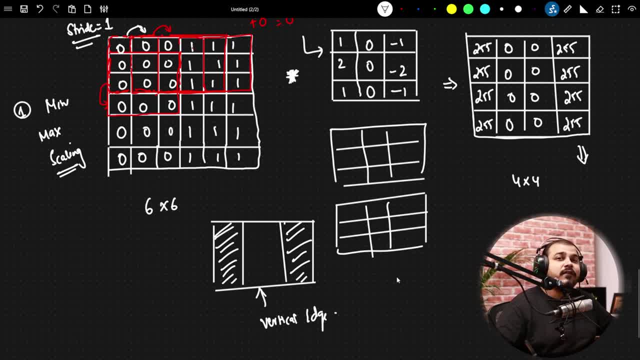 let's say: Okay, So I may have multiple kind of filters over here. you know, And this filters. you know, this filters is basically like what we are doing. It's just like This information: we are trying to extract it from the image. 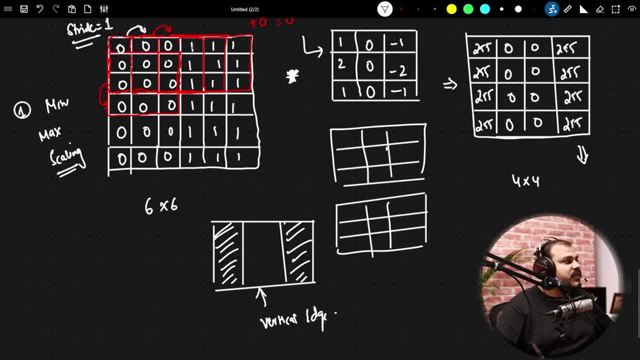 With the help of this filters, we are just trying to extract the information of this specific image, right? So I hope you are able to understand till here, right Now, in a specific image. whenever we are performing convolution neural network, we can have multiple. 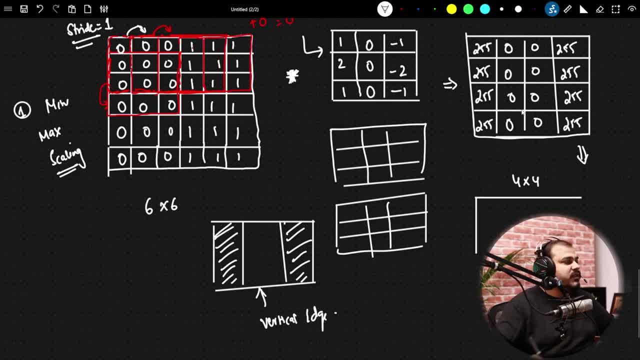 filters like this And we will also be getting multiple outputs like this. Okay, So, like this, multiple outputs we will be getting. Okay, Like how we got over here. For horizontal filter, We may get a different output. For round shape filter, we may get a different outputs from a specific image. 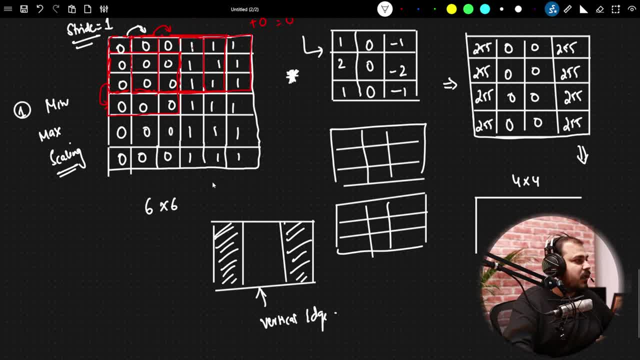 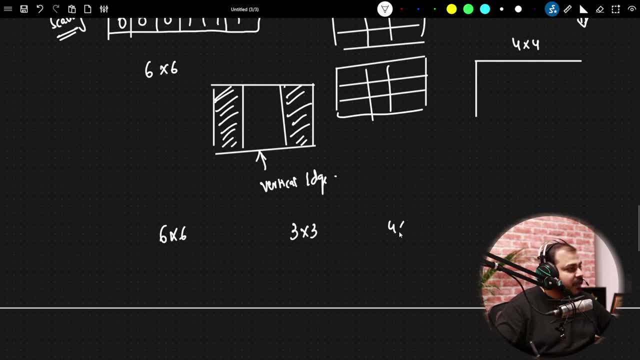 Okay, Now you need to understand some very important things. Whenever I pass a 6x6 image in a 3x3 filter, I am getting an output as 4x4.. Right, Whenever I take a 6x6 image, I pass it through a 3x3 filter, I get an output as 4x4.. 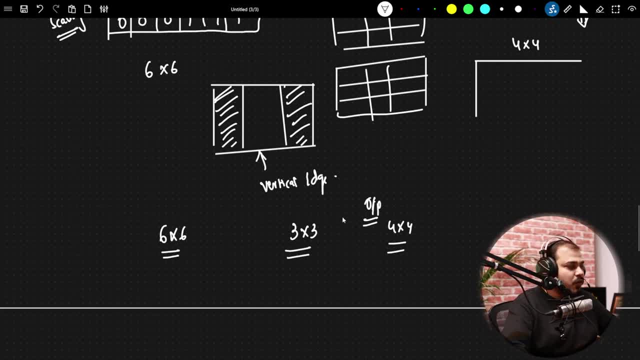 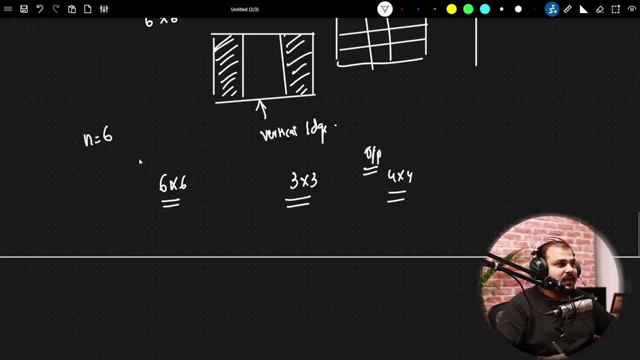 Right, How this is basically happening, Right? So over here, let's say the size of the image is given by n, So n is equal to 6.. Okay, n is equal to 6.. Let's say the filter is nothing but 3.. 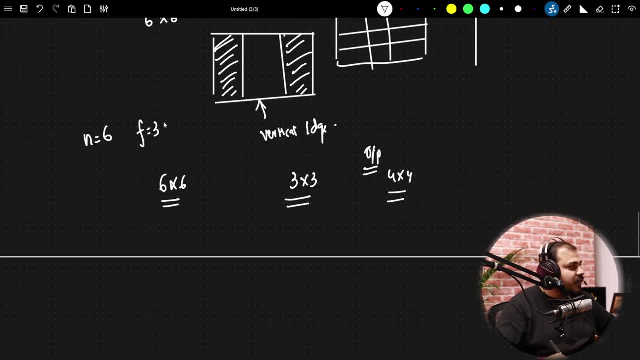 Right. So if my n size is 6 and filter is 3, what will be my output image? So here you can use a mathematical formula. The mathematical formula will be n minus f plus 1.. So when you use this n minus f plus 1, it is nothing but 6 minus 3 plus 1.. 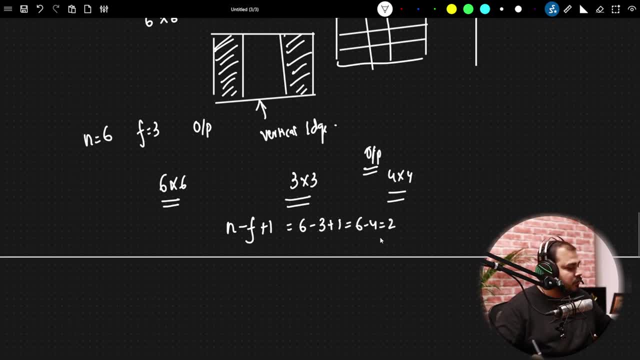 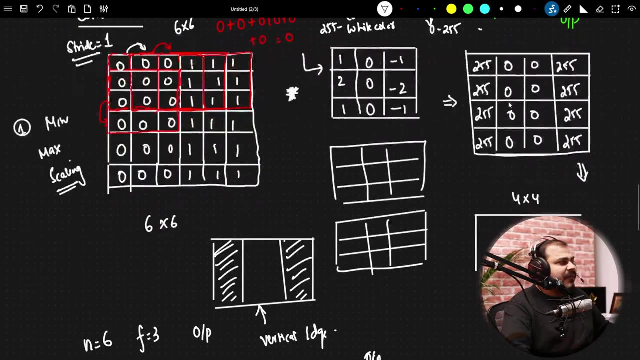 Which is nothing but 6 minus 4, which is nothing but sorry, which is nothing but 3 plus 1,, which is nothing but 4.. So, finally, you are getting a 4x4 output. Okay, Now you may be having a confusion, Krish. how do we define this filters? 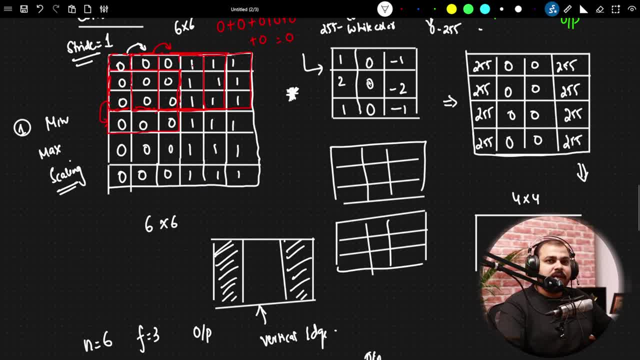 You don't have to define it, guys. I'll talk about it just in some time Here. you don't have to even do any kind of hard coding. I'm here. I'm just giving an example. Let's see what filters can actually do. 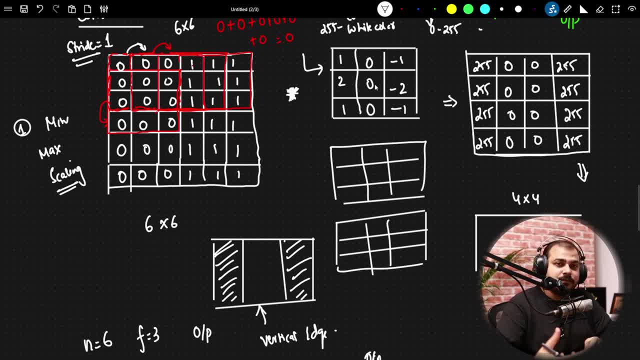 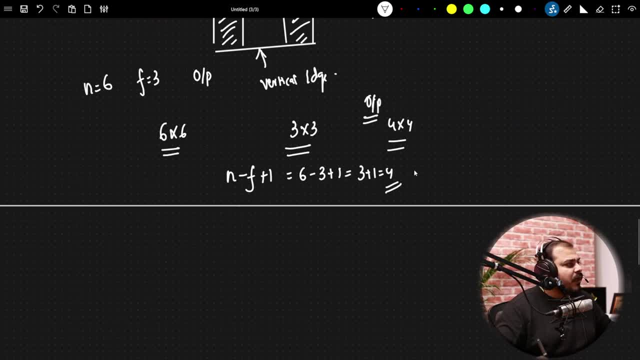 Filters can actually take out the information from the specific image. Okay, How do we define this filter? I'll just say in some time. Okay, But here you understand that you have applied this formula and I have got: 3 plus 1 is equal. 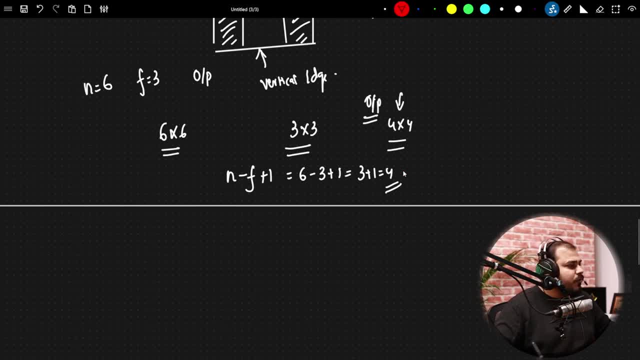 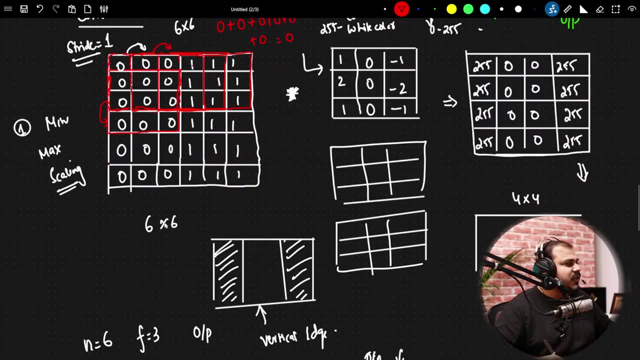 to 4, and that is what my output is Right. That is what my output is Right. Now, a very important question: What is happening? See, if I give a 6x6 image to a convolution operation, I'm getting a 4x4 value output. 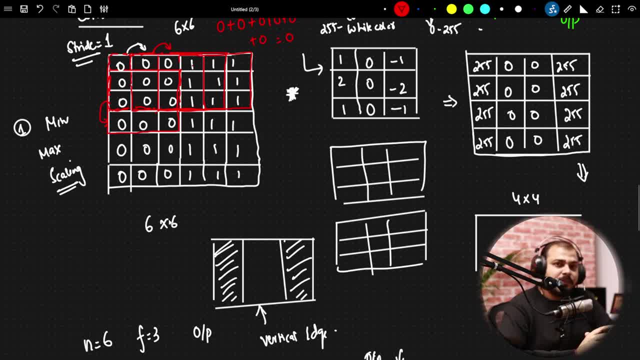 Okay Here, my image size is decreasing, and this should not happen. If my image size decreases, that basically means we are losing some kind of information. Now, in order to prevent this loss, what we can actually do? We can come up with something called as padding. 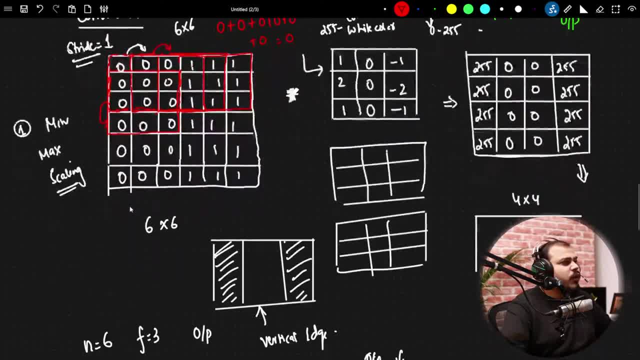 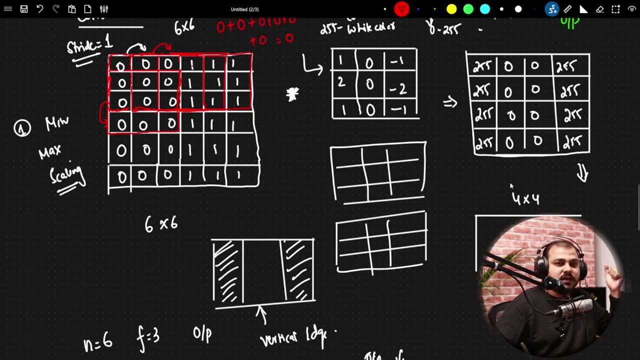 Now, what exactly is padding? Padding says that do not do anything If my image size is 6x6, I want to get the same output over here like 6x6, all you have to do is that apply padding on top of it. 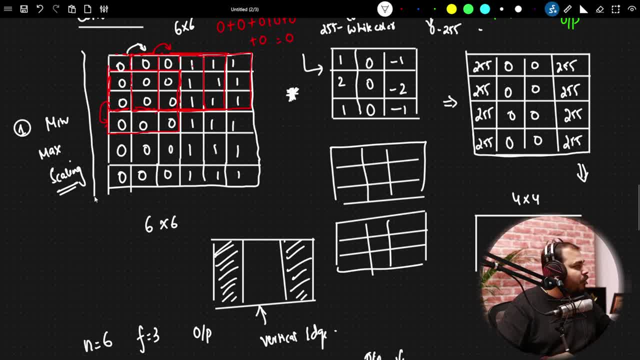 So how do I apply padding? Padding is just like building a compound, building a compound around the images. Let's say, I'm building one more additional compound on this specific image, on this specific image, on this specific image, like this: Now, when I build this compound, when I build this specific compound, then what will happen? 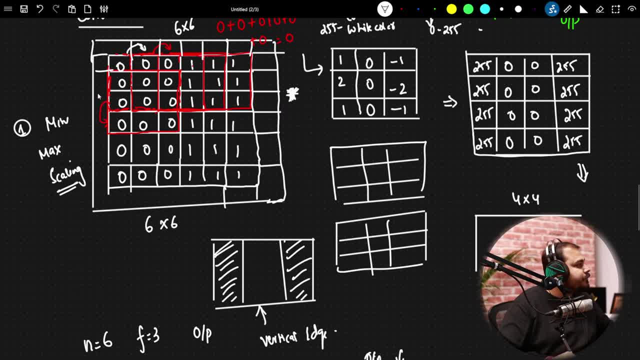 When I build this specific compound, what will happen? So if I build this compound here, you will be able to see that I'm actually getting a 8x8 image. My image size is 6x6 only, But now it becomes an 8x8 image. 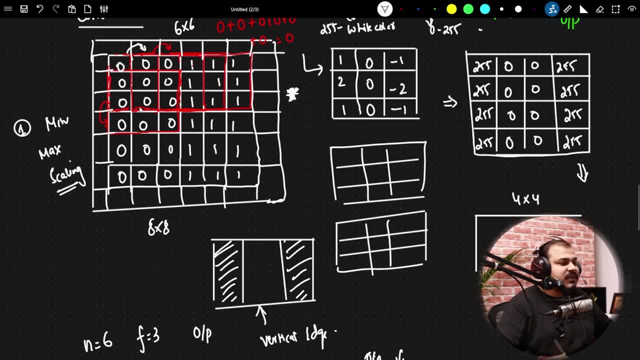 Okay, Now it becomes an 8x8 image, But my image size is anyhow, 6x6.. Okay, But since I'm applying padding, this concept of applying a layer on top of the image- I'm applying a layer on top of the image- is called as padding. 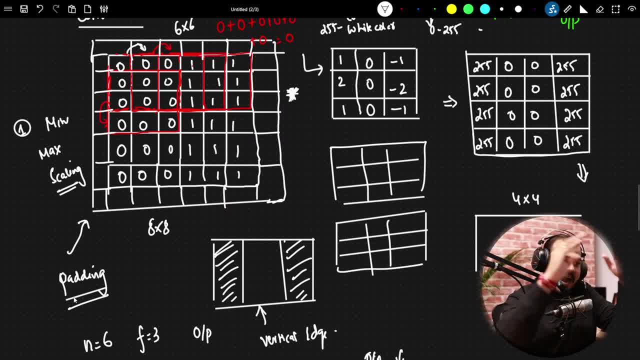 Padding basically means that I am protecting the image by adding another layer on top of it. Okay, Now you may be thinking what values can come inside this specific cell. This is a question that many people may have. For this, you can have different kind of paddings. 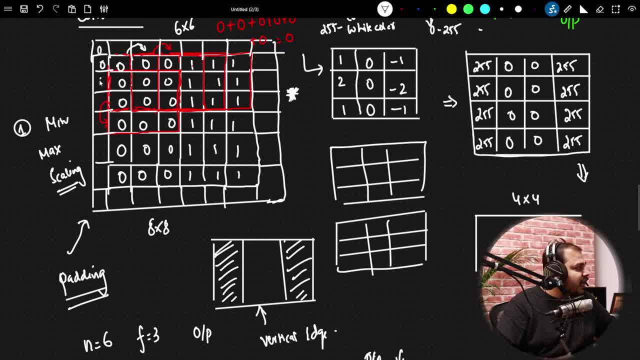 One kind of padding is that zero padding. Just go ahead and fill this cell by zeros. Okay, Just go ahead and fill this cell by zeros. The other kind of padding is that zero padding- Okay. The other kind of padding is that whatever is the nearest value, you try to put that. 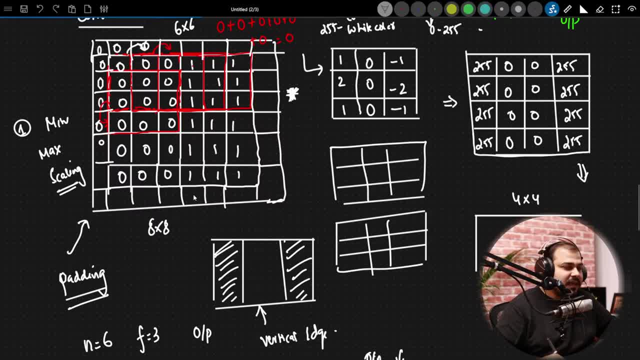 Okay, Like suppose I'm trying to pad or put some values over here. The nearest value is 1.. So I'll try to put 1 over here. Okay, I may put also 1 over here. 1 over here. Now, if I apply the same operation, what will happen? 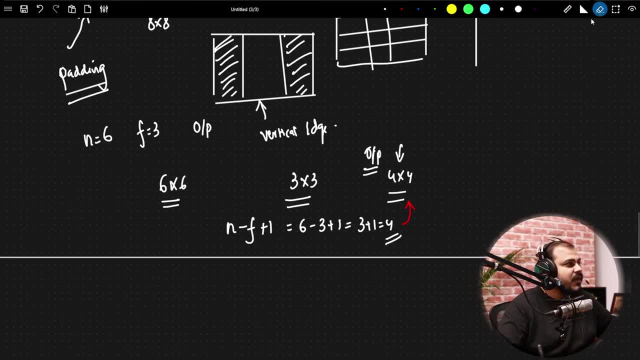 See My image size. initially was 6. But after applying padding it became 8.. Right, It became 8 now. So 8 minus. this is after padding. 8 minus 3 plus 1 is equal to What is this value? 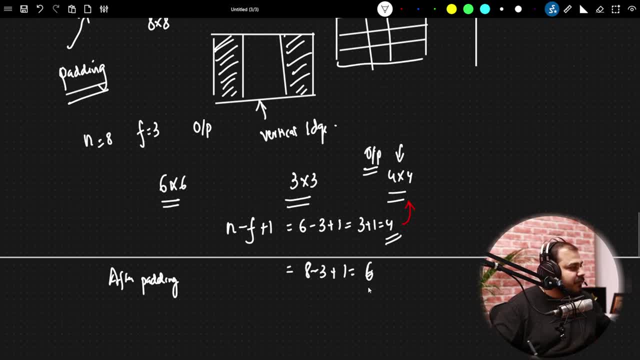 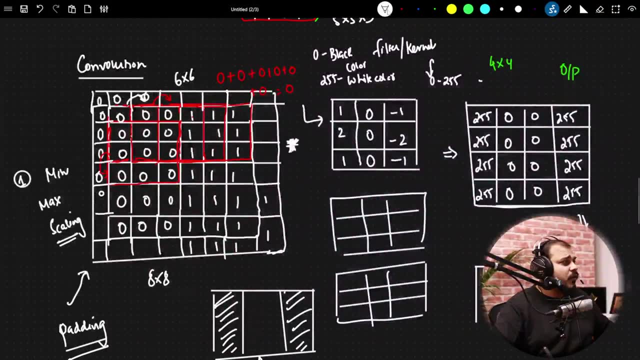 This is nothing but 8 minus 3 is nothing but 5.. 5 is nothing but output. It will be 6.. So, finally, you'll be seeing that I will be able to get one more additional layer, and this additional layer will actually create a 6 cross 6 image. 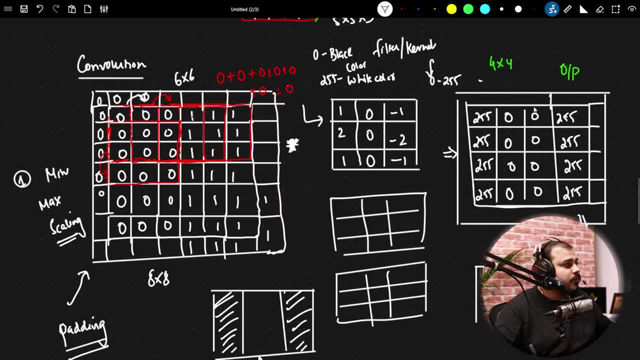 It'll create a 6 cross 6 image. Okay, it will create a six cross six image. okay, so this will actually now become a six cross six image. this is what we wanted, right? this is what we wanted and what will be this values that will. 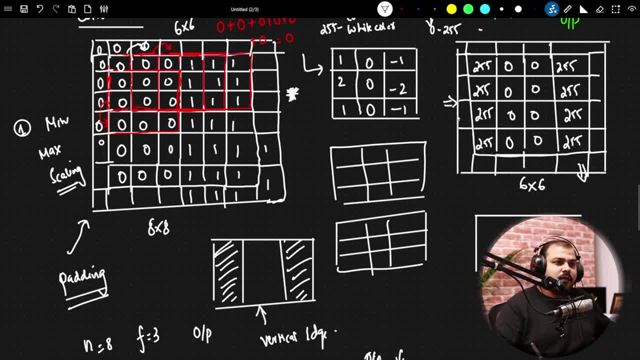 be coming up based on the calculation. whatever we get through these filters, we are going to get that and remember, we will be starting our again filtering operation from here, convolution operation from here, and then we will be crossing this entirely and finally i'll be getting a six. 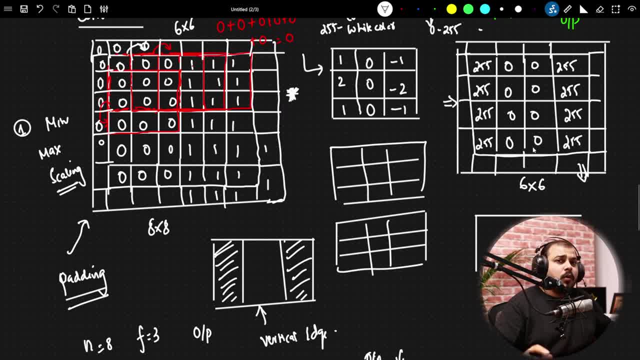 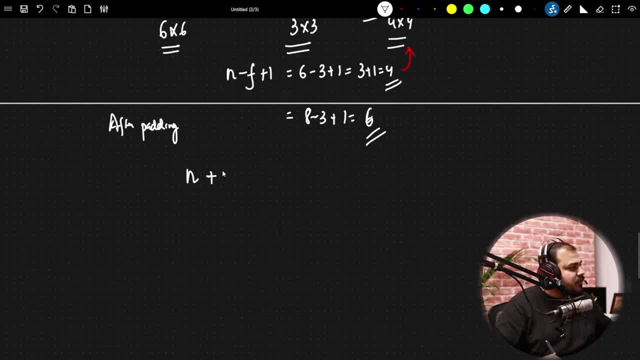 cross six output. okay, so what will be now my updated formula? my updated formula will be now like this: n plus 2p minus f plus 1. so what will be my initial size of the image? six, right? how much layer of padding? i am actually doing one padding, right? i did one padding for this, one padding for. 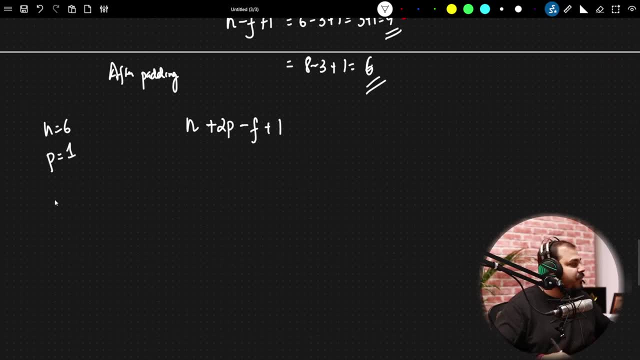 this. so i i'm writing: p is equal to one. what is my filter size? it is nothing but three. and here, if i try to put all these values so it will become six plus two minus three plus one, it is nothing but six plus two is eight. eight minus three is five. five plus one is nothing but six. so finally i'm. 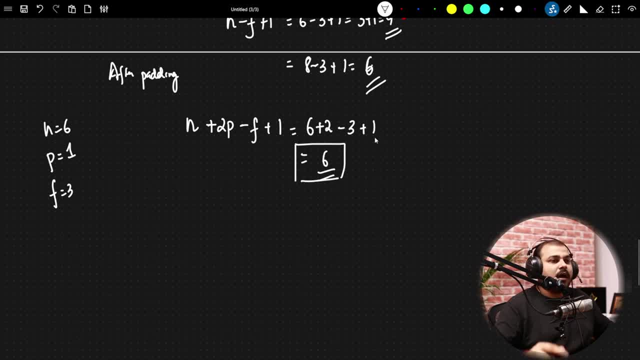 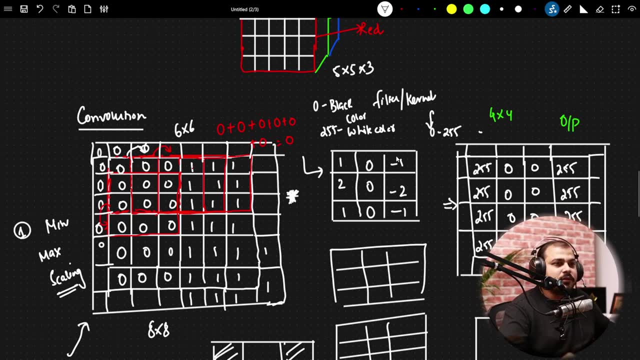 actually getting six as my output and this will be the output of the specific image. okay, so a very important interview question: what is the importance of padding to prevent the information from being lost in the image? we basically apply different kind of padding techniques. okay, so this is with. 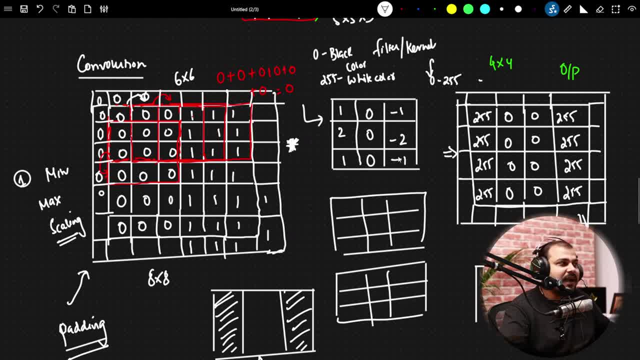 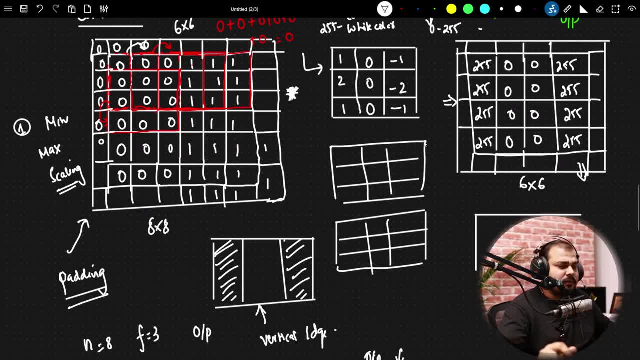 respect to convolution operation. i hope everybody is clear. the main thing is that i'm just trying to extract some information now. a very important thing again, very, very, very important. as many people said, or many people may have a confusion saying that thresh, why did you hard code these? 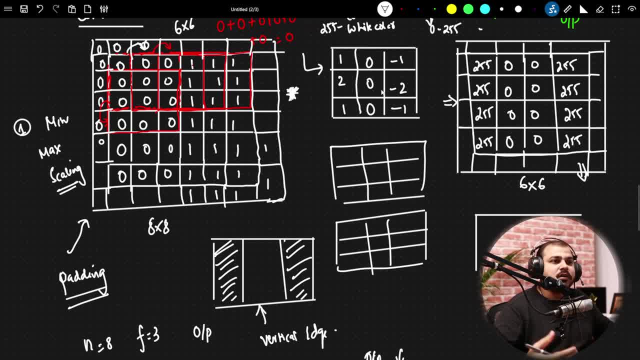 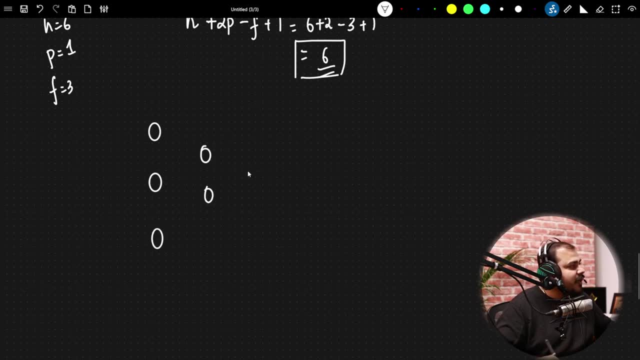 values and in a real world problem statement, do we need to hard code this? specific values. okay, the answer is no. you don't need to hard code this like how in ann, how in ann, let's say how in ann, we create a neural network like this. i have my hidden layer and i have my output layer. right, i have my output. 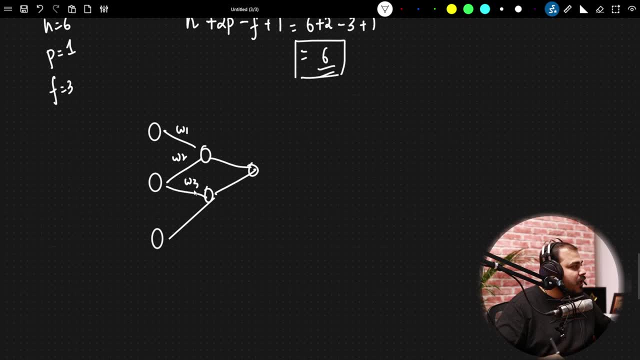 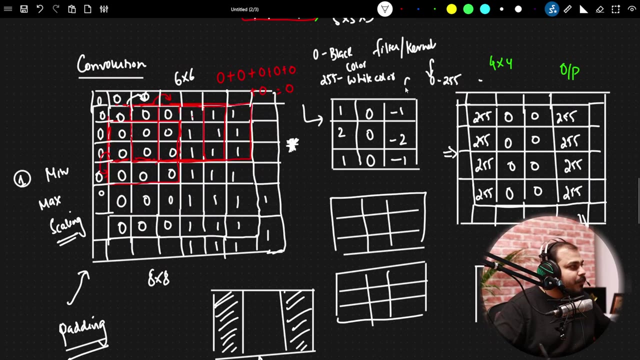 layer right. in this we assign weights right and in the back propagation we we update this weights. so in cnn also, you also have to make sure that you update the filters based on the input. so we need to update this filter values. okay, initially, let's say that we have initialized. 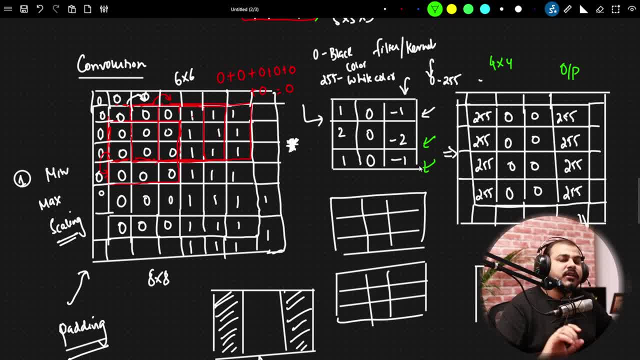 some filter randomly. okay, initially we have initialized some filter randomly, but through back propagation again, like how we did in the case of ann. we also have to update this: filters based on the input image, because every image will be different. right, every image can be a black and 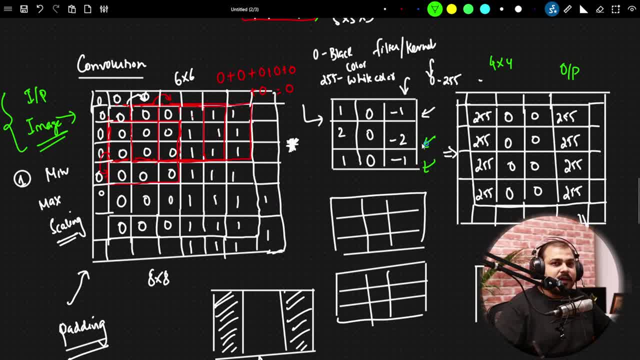 white, it can be. rgb, it can be of different, different types. right, so, with the help of back propagation, i need to update these filters. but now still, the question comes that how back propagation will actually happen. we have still not used any kind of activation function, so where do we? 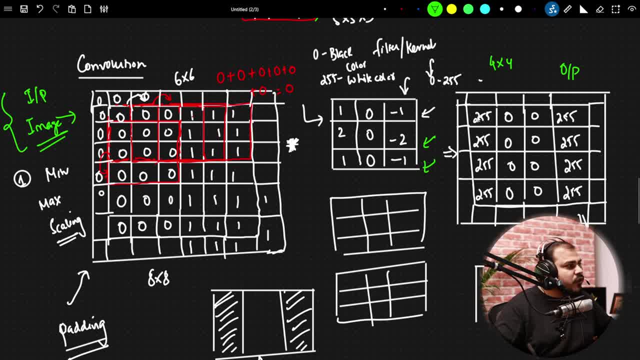 specifically use the activation function after this convolution operation. guys, whenever we get the output on top of this, for each and every value we apply a relu activation function. i hope everybody knows the importance of relu activation function. relu activation function is nothing but max, comma, zero, comma, x, right. so i hope everybody remembers this. so, on each and, 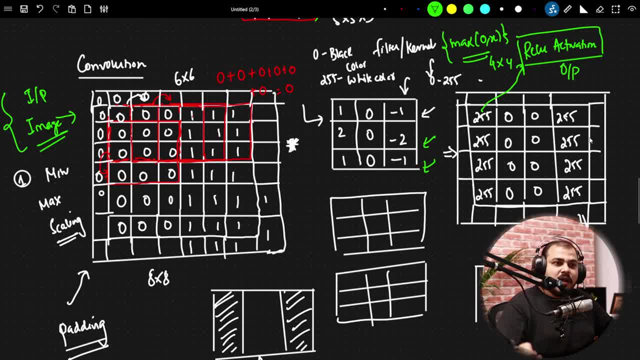 every value, we apply a relu activation function. now the question is that: why do we, why are we applying relu activation function? because you know that relu activation function during the back propagation. the derivative can not be applied to the back propagation function. so should the filter be applied to the filter alpha value, the derivative can be found out. 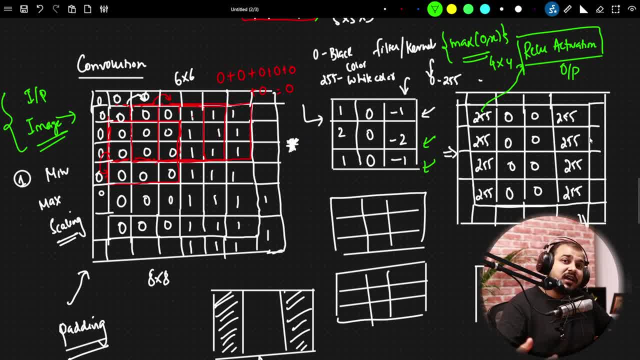 now, since we can find out, the derivative relu activation function or other activation function like pre-rew can definitely get applied over here, because in the back propagation we will be updating this- all kind of filter values. when we have all the values over here and we apply relu activation function on top of it, you will be able to do the back propagation. 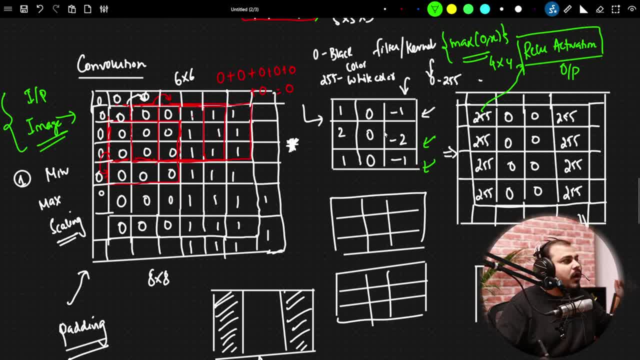 and you will be able to find out the derivatives and, similarly, you'll be able to update this filter values. I hope I'm super clear with respect to this. One important thing: I told you about stride right Now, what if my stride becomes two? 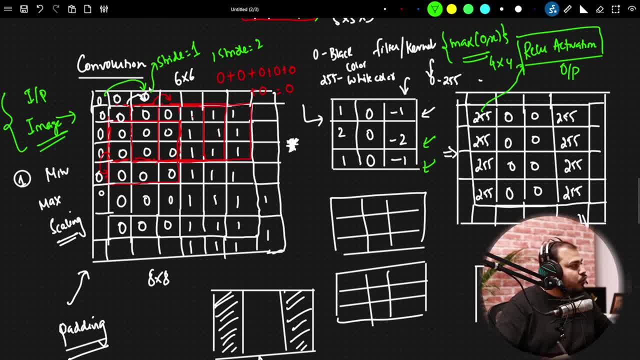 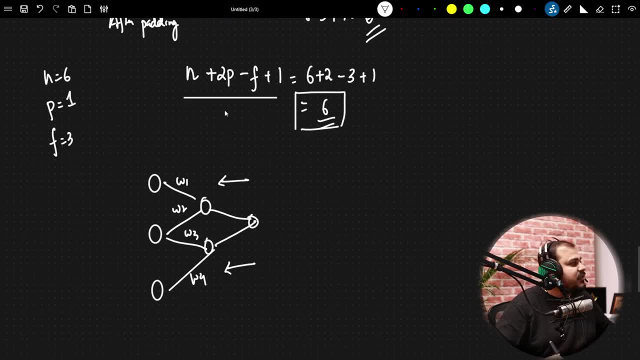 Your stride can also become two right, I can jump two steps. I can also jump two steps while doing the convolution operation. Will this create an impact in my output? Yes, definitely, it can create an impact in your output. So now my updated formula. it will not be just like this. 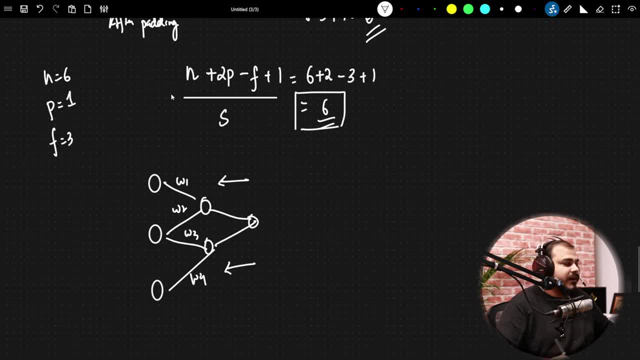 but it will be divided by S. S basically means stride. okay, So if my S is one, I did not write this, but if my S is two, this will definitely create an impact with respect to my output. okay, So is it clear, guys. with respect to convolution operation, 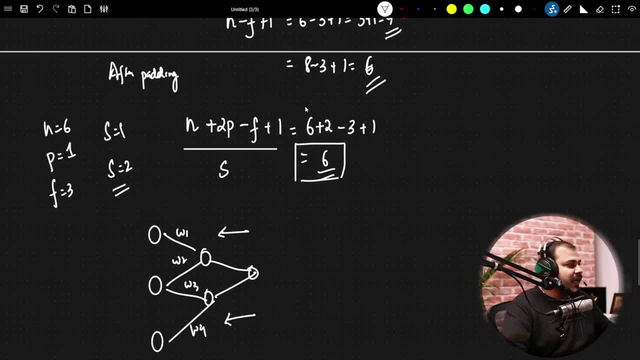 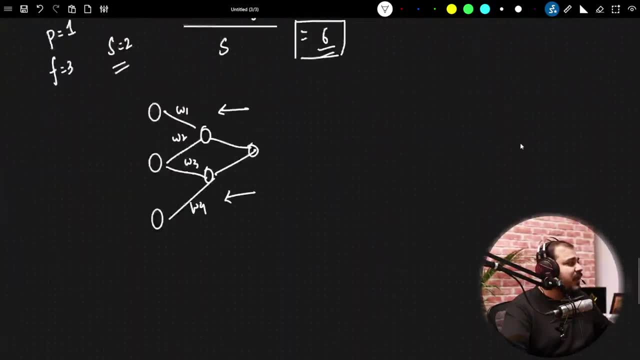 I've covered convolution, padding, stride, everything and the formula. What is the use of this ReLU activation function? Everything? Is it clear? everyone? Can I get a quick? yes, I hope you are able to understand till here, Okay. 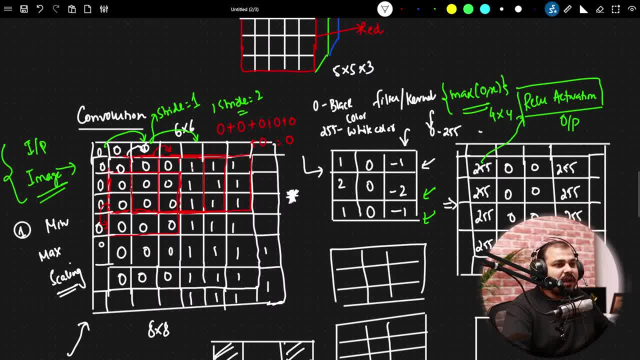 So this was with respect to convolution operation. Now let's go ahead and understand the next operation, which is called as max pooling. So like this, this convolution, we can have horizontally stacked right. So what are things we have in the convolution neural network? 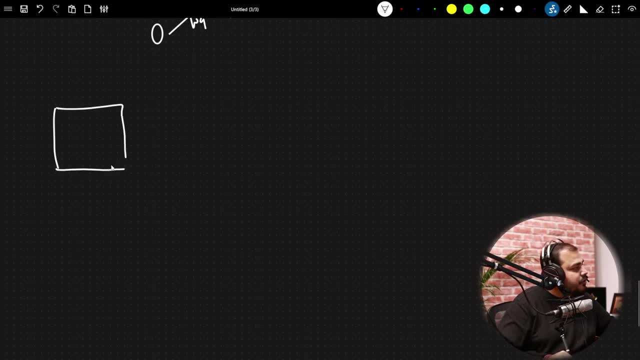 Quickly, let me just write it down. So I have a specific image, Let's say some image over here: four cross four. one, two, three, four. This will also be four cross four. This will get passed. This will get passed to another filter. 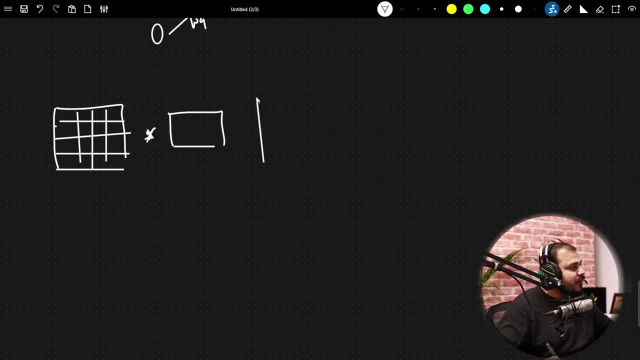 Okay, And based on this, any filter it can be, I will be getting an output right. So this entire thing, along with the ReLU activation function, is basically my convolution operation. Convolution operation And this entire thing can be stacked together. 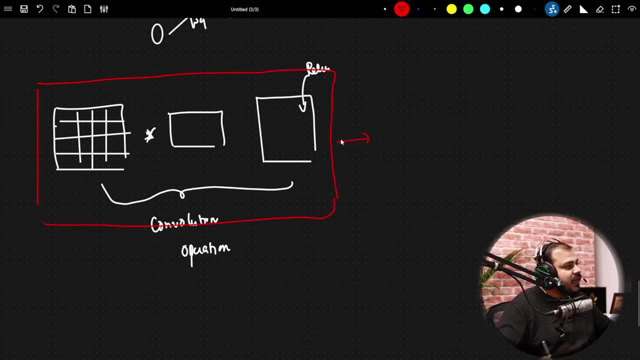 So this will be my one convolution operation And after that in my CNN I may have another convolution convolution operation, similarly like this right and over here, i can have any number of filters. i can have any number of filters i like. okay, this you need to understand and our main aim in the 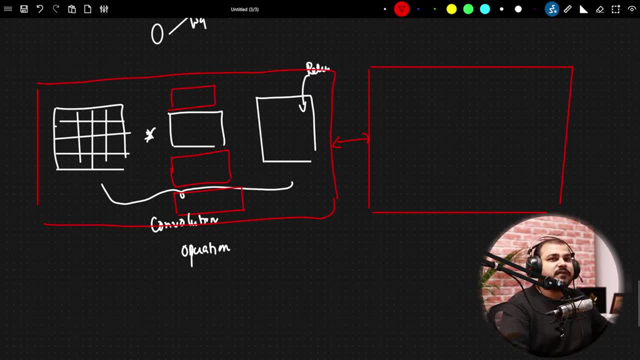 convolution operation is that we need to learn from this. filters, we need to learn and update based on the input images. based on the input images. we need to learn from it. okay, so i hope you are able to get the idea about it and you are able to understand over here, okay, okay, now let's go. 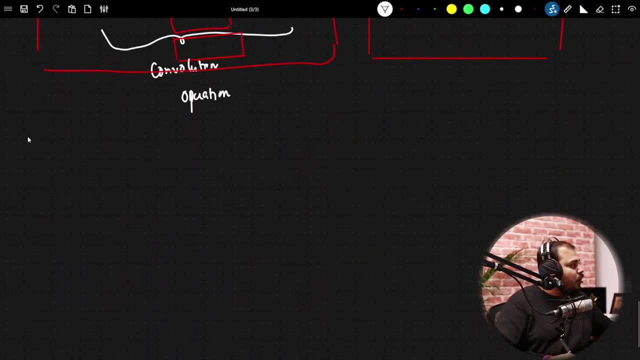 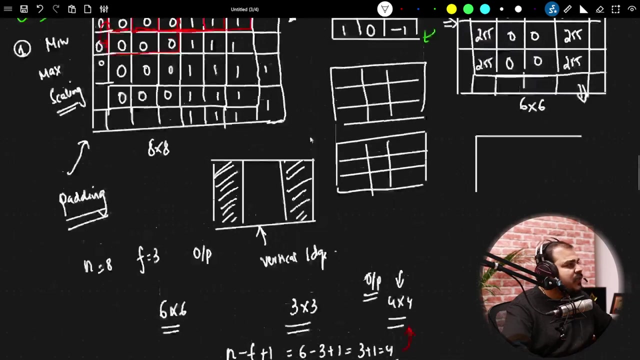 to the second one, which is called as max pooling. now, what exactly is max pooling? max pooling- okay, after a convolution operation, there is something called as max pooling layer. okay, and i will show you in images also how it will look like over here. just try to understand the crux, understand the keywords that i'm 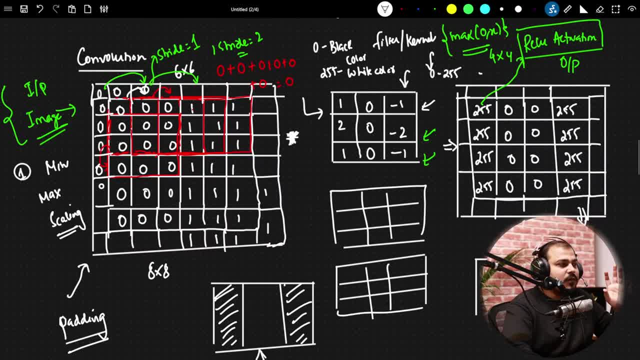 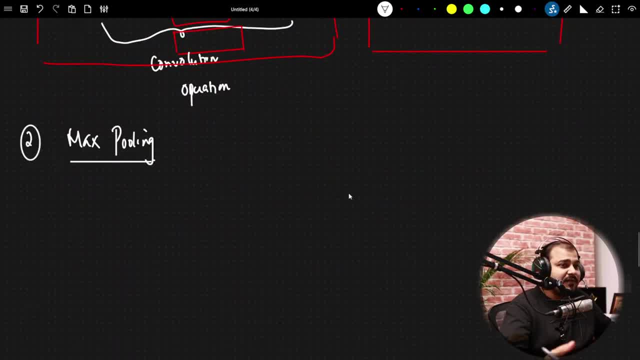 specifically using right. this will all actually help you to understand in a better way. okay, now filters can be selected in different, different ways. you can have a 5 cross 5 filter. you can have a 7 cross 7 filter. you know. you can have a 3 cross 3 filter. this is all like a hyper parameter tuning. 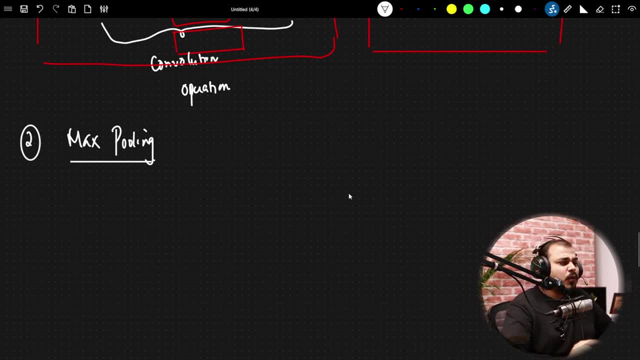 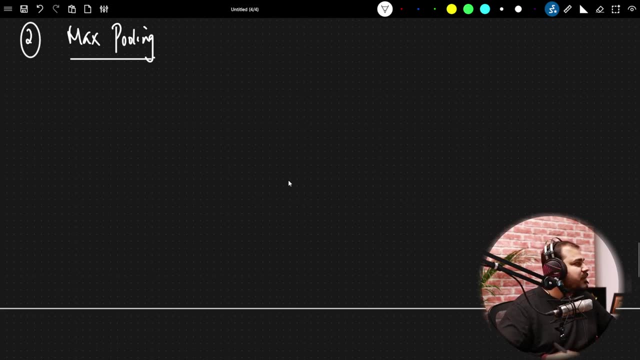 later on in the upcoming classes i will probably take one more live session there. i'll discuss about transfer learning. okay, now in the max pooling layer, what happens in a specific max pooling layer? let's say this is my input. let's say i have three cats, so this is my cat one, this is my cat two. 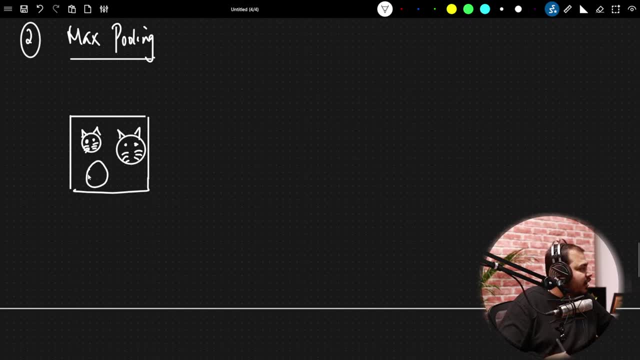 okay, i hope you like my diagram, and this is my cat three. okay, let's say this is my cat one and this is my cat two. okay, let's say this is my cat three. okay, let's say this is my cat two. okay, i hope you like my diagram and this is my cat three. okay, let's say this is my cat three. okay. 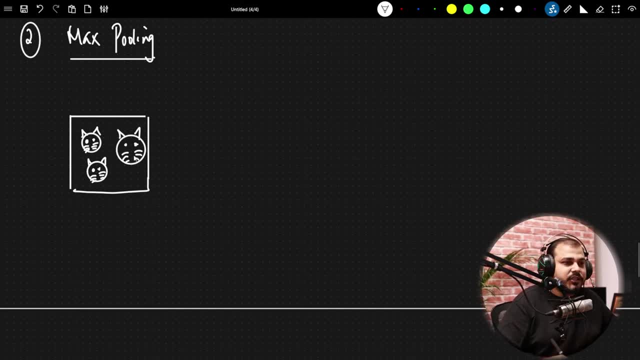 Let's say this is my image with respect to a cat. and then my first operation is basically my convolution operation, where I pass through a filter or kernel. I get my output over here. let's say I am getting an output over here, This output, and after the output we apply a relu activation function. 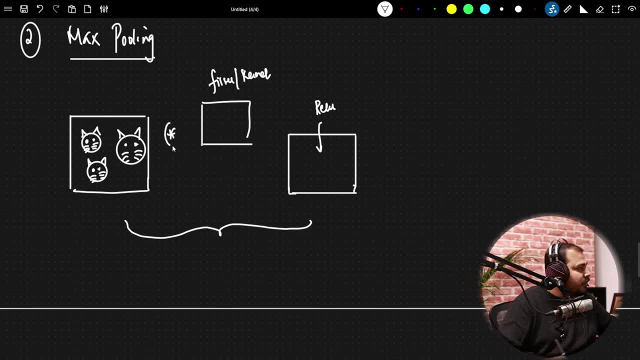 So this entire operation is my convolution. so that basically means I am applying this and I am getting this. So this is my convolution operation. Now, after this, what can we have? we can have multiple convolution layer also, but again, I have seen lot of transfer learning techniques where they have used another layer which is 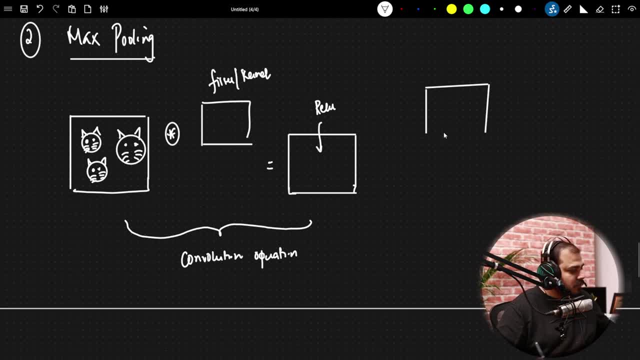 called as maxplot. So here I am just going to define something like this And this layer is basically called as max pooling layer. I will talk about max pooling layer. Let's say, after this convolution operation I applied the relu and I probably got a 3x3. 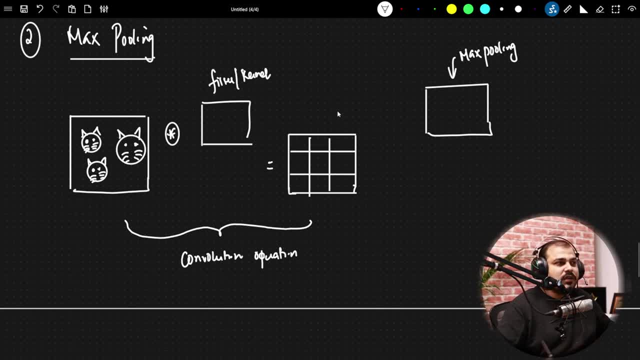 output with some values. I am just going to initialize values, so don't worry that. how did I take up? Let's say that this is a 3x3 and I have got some values, Some pixel values like this: 1,2,3,4,5,7,0,3,5.. 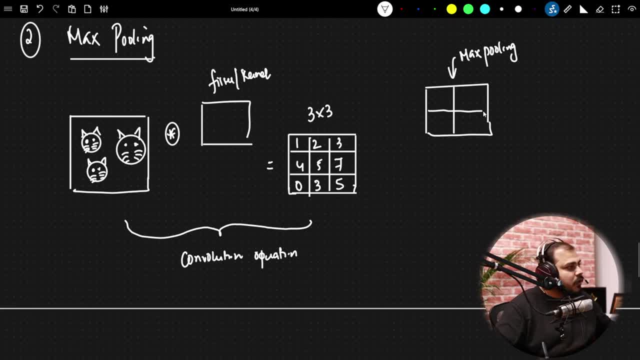 So let's say this is my this. Let's say I am using a max pooling of 2x3.. Now why exactly max pooling is used? Now, see guys, here I have 3 cats, Here I have 3 cats. And when I apply a filter operation, let's say, from these images I am able to see the. 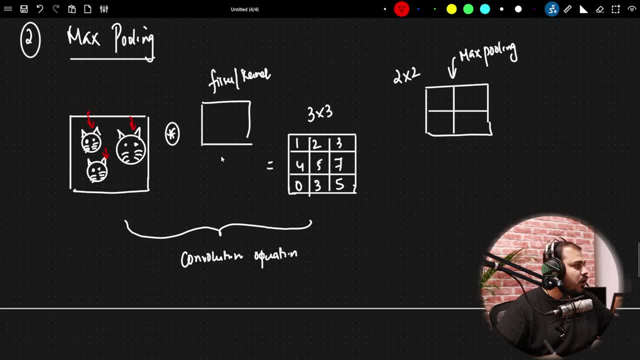 rounded eyes. Probably I will be having another filters also for vertical edges, horizontal edges and all Now some information I am able to extract from this particular filter. Let's say, I may have any number of filters as we go ahead, But I am just focusing over here. 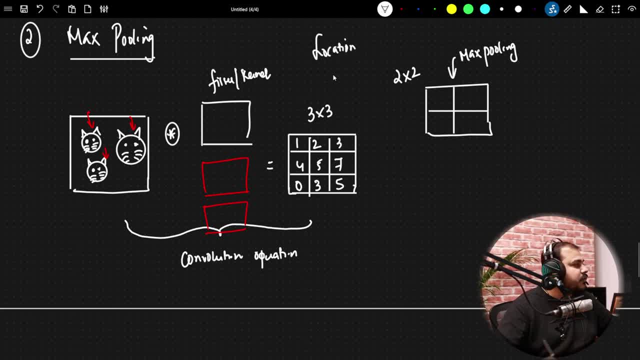 Now there is a concept which is called as location invariant. Now, what does location invariant say? Location invariant says that, let's say there are multiple objects in the images, My convolution neural network, till it goes ahead towards the next layer itself, it should. 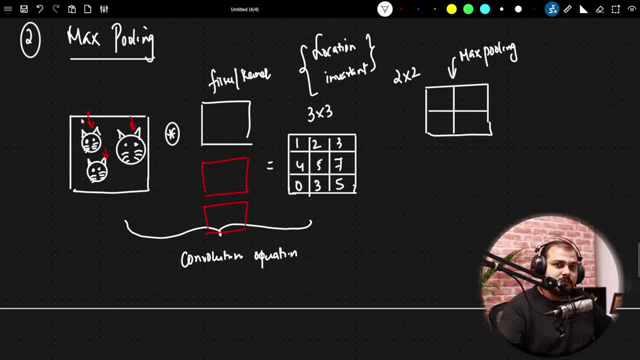 be able to extract more and more clear information, More and more clear information. So location invariant basically says that my objects may be present anywhere, But as we pass from many convolution layers, I should be able to extract the information more in a better, in a clear way. 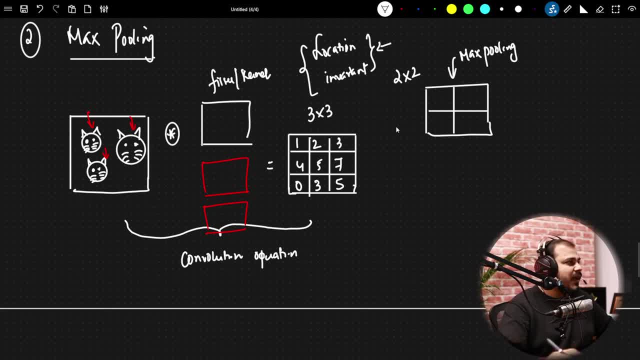 Right. So in fact, we specifically use something called as max pooling. Now, in max pooling, what it does is that let's say, how do I extract much more clear information? How does this information look like When I apply max pooling? max pooling says that: okay, I am just going to place on top. 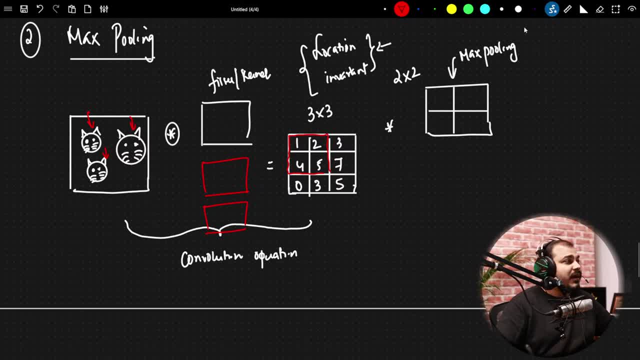 of it. And let's say: and there are different types of max pooling layer, There is something called as average max pooling. Let's say there is something called as average max pooling. So let's say there is something called as average max pooling. 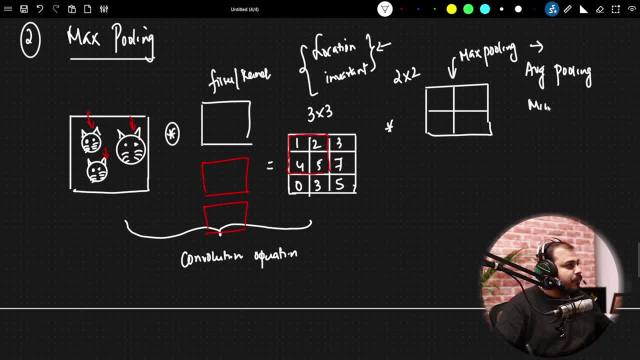 Let's say there is something called as average max pooling, There is something called as average pooling, There is something called as min pooling And this is my third type, which is called as max pooling. Okay, Let's say, in this particular scenario, I am using this max pooling. 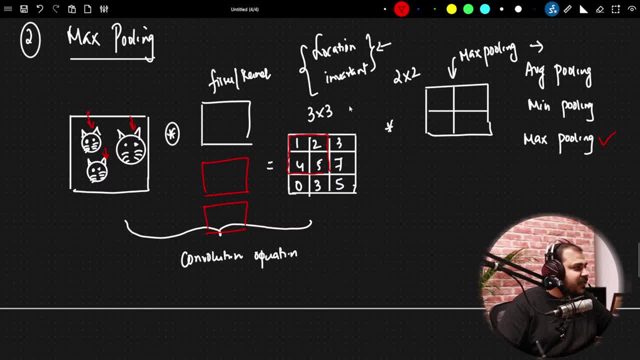 Now max pooling. what it says is that I am just going to place this on top of the output over here, And what I am actually going to do, I am going to basically get an output, And this output will only be focusing on the biggest number. 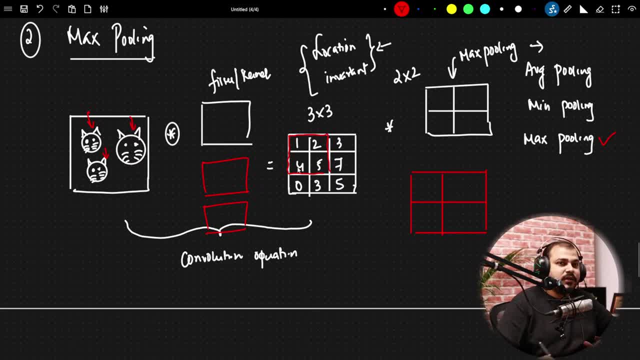 The most clear or the highest number over here. Which is the highest number over here? Clearly, you can see that 5 is the highest number, So I am going to take this information only and update it over here. That basically means one of the cat eyes is clearly visible. 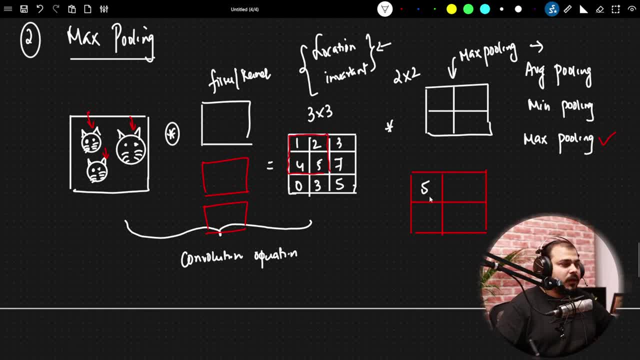 So I am just going to pick up that information and put it over here. Okay, Then I am just going to jump to the next stride, Right In the next stride. what I am actually going to do, I am going to basically jump like this: 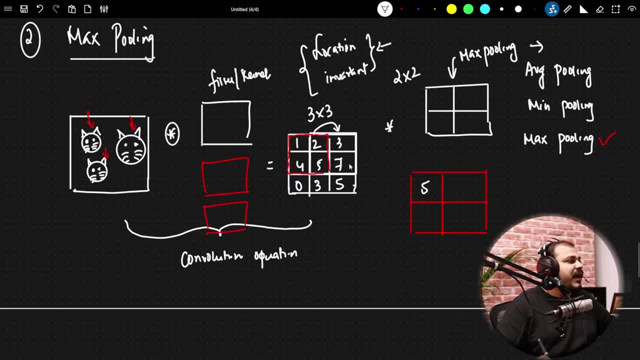 and basically take up the next one. Okay, So from this, the highest value that I am actually going to get is 7,. let's say Then I am going to jump next downwards in this direction, let's say in this direction and this direction. 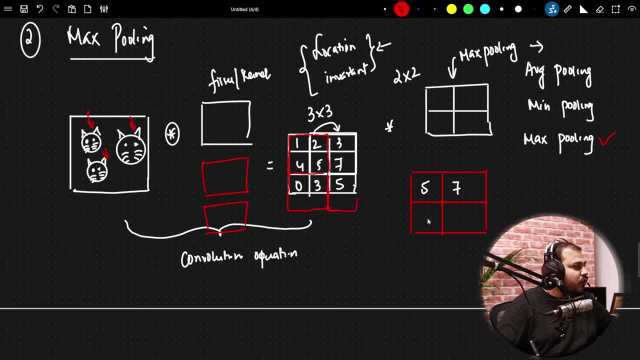 And I am going to basically see that which is the highest value. So over here also, I am going to get probably 3, and over here I am going to get 5.. So the most specific and the clear information, I definitely want it from this. 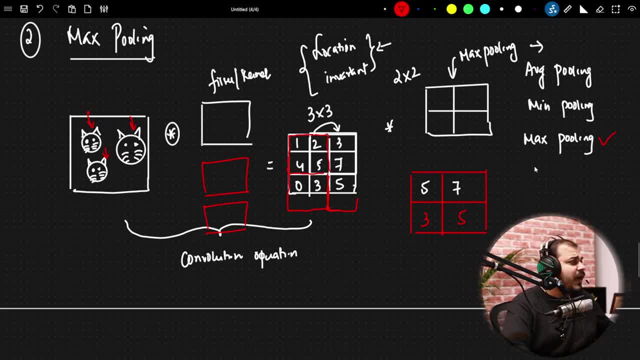 Okay, So what I am actually specifically doing And over here, guys, one more thing that you need to really understand is that here I will make a stride of jump 2.. Okay, Stride of jump 2, not stride of jump 1.. 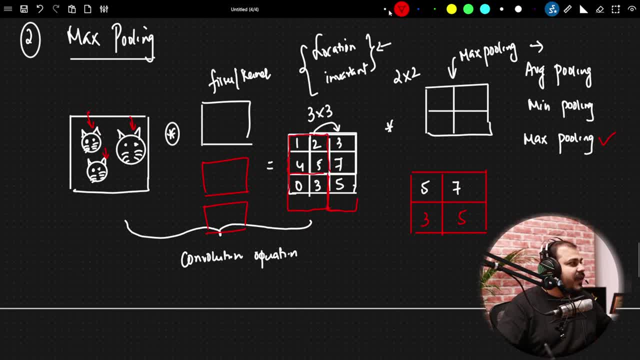 Let's say, initially, stride was here, I got the value as 5.. My next jump will be a 2 step jump, So my next one will be starting from here and it will be ending like this, And out of this I have my highest value as 7.. 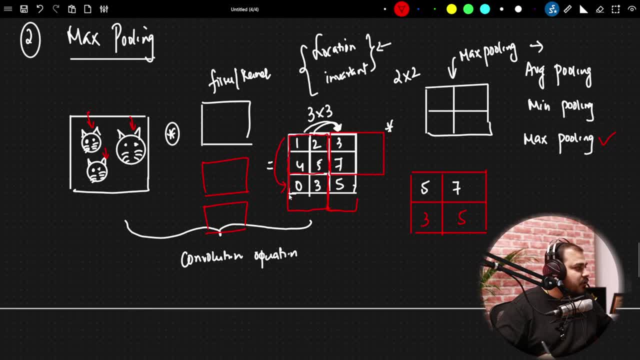 Then, similarly, I will make a stride 2 jump downwards. So this will be my next one. From this, I know which is my highest value: 3.. And then I will again make a stride jump of 2.. And when it comes over here, whatever value is highest, I will be getting it. 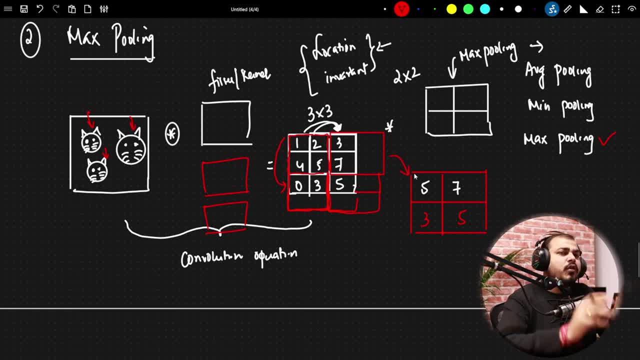 So here I am actually trying to specifically take up the most important information out of the output that I have got from this specific filter. Okay, And this basically solves the problem of location invariance. That basically means if I have multiple objects also and if one of my filters is able to determine 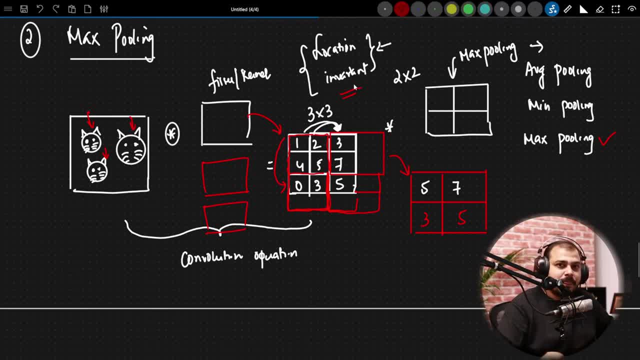 that particular object, It will be able to clear it. Okay, Pick up from there, Okay. So I hope everybody is able to understand till here And I hope everybody is understood about the max pooling Right Now suppose I want to use some other pooling. 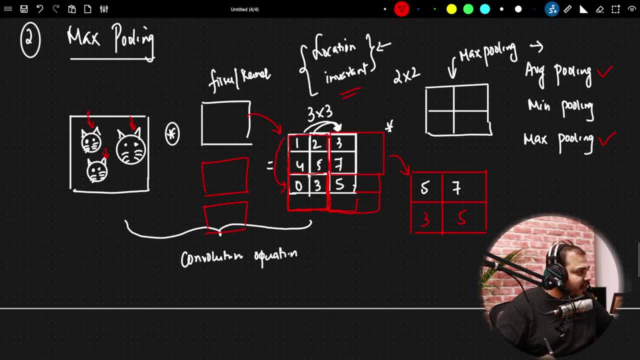 Let's say average pooling. In average pooling, nothing will happen. We will just try to find out the average of all these values And, similarly, in min pooling, what we are going to find out? We are going to find out the minimum values. Now, based on different, different problem statement, we can play with either of this pooling layer. 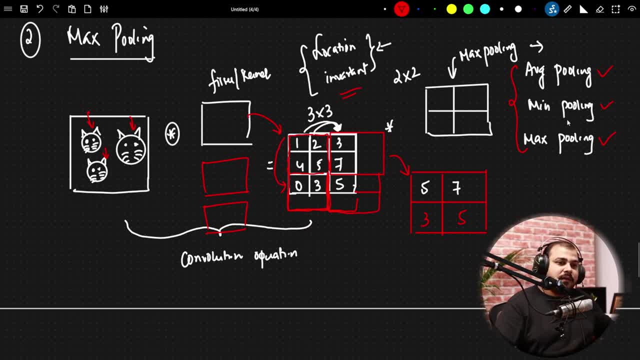 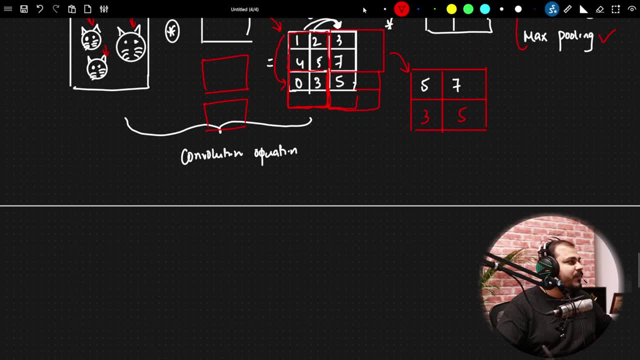 Okay, We can either use max pooling, we can either use min pooling, we can either use average pooling. Okay, So finally you get this. and with respect to different, different filter operation, again I may get another 2 cross 2 over here with some values, let's say like 7, 9,, 2, 1.. 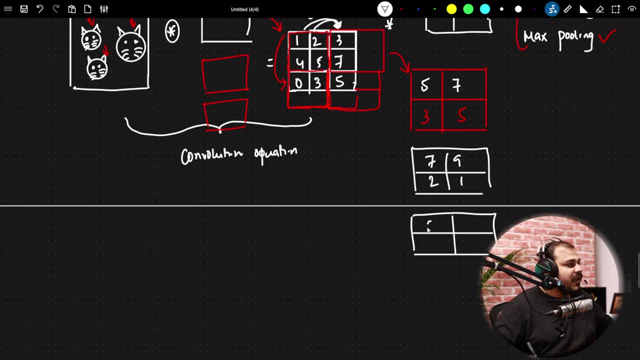 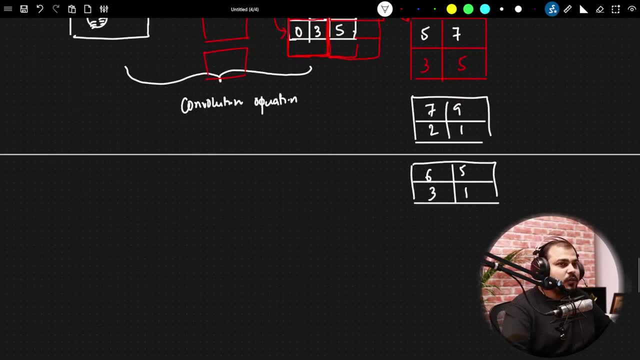 Then another filter will actually able to give me some other values, like 6,, 5,, 3, 1.. Right, So all these values that I am actually getting, like this, Okay, What I am actually going to do now. This is the end of the max pooling. 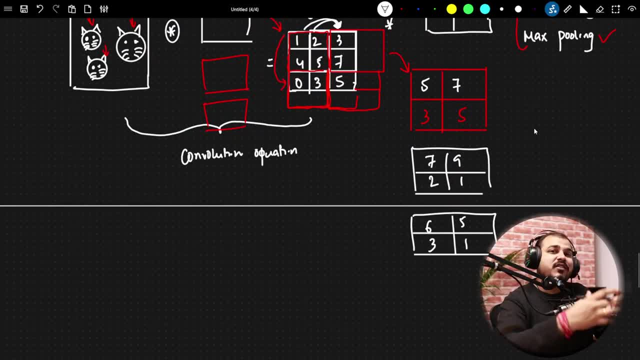 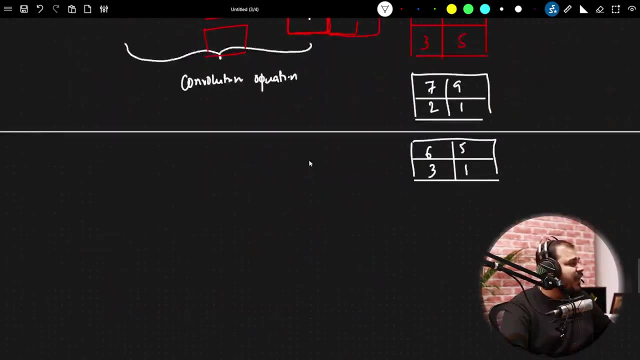 And again, convolution and max pooling layer is used as a combination. We can stack it horizontally any number of times based on different different neuron layer. Okay, Different different neuron layer. Now, what will happen after this? After this, there is an amazing layer because finally we get this output. 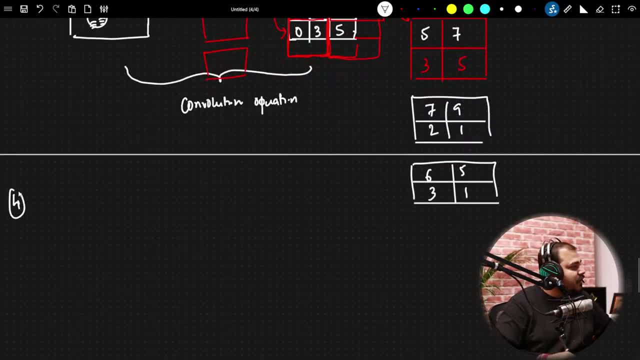 Right, Everyone. Then after this, we have something called as flattening layer. Now, flattening layer is pretty much simple, Because this will actually look like an ANN dense layer, only ANN dense layer. Now, whatever inputs, whatever outputs I get from this max pooling I am just going to make, 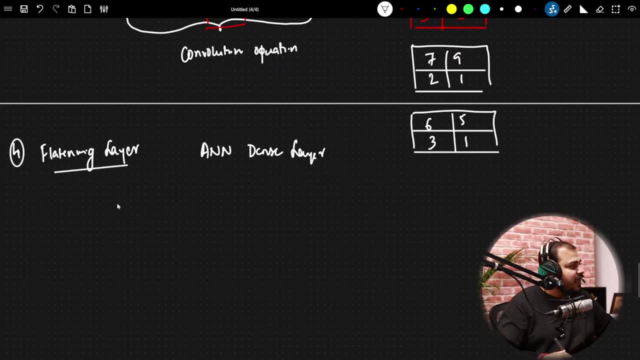 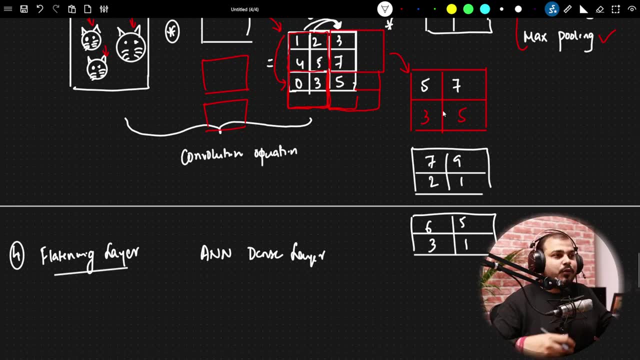 it straight forward: flattened. Flattened basically means I will just go, I will just pick up this entire filter and I am just going to elongate it like an input, like how we give input to a ANN Right, Like that we are going to flatten it. 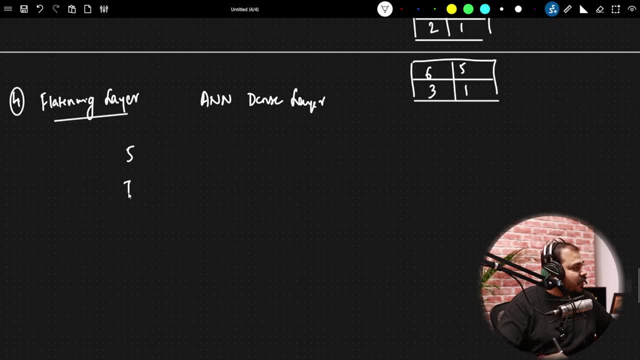 So my 5735 will get elongated. Okay, It will get elongated to something like this: It will become 5735 and this will basically get elongated, which looks like this: Okay, Then the next filter value that I am going to get: 7921. that will also get attached to. 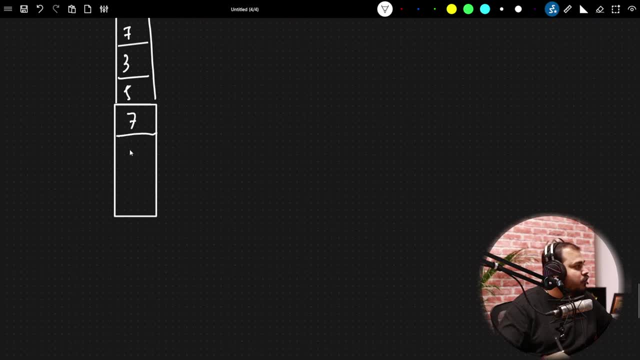 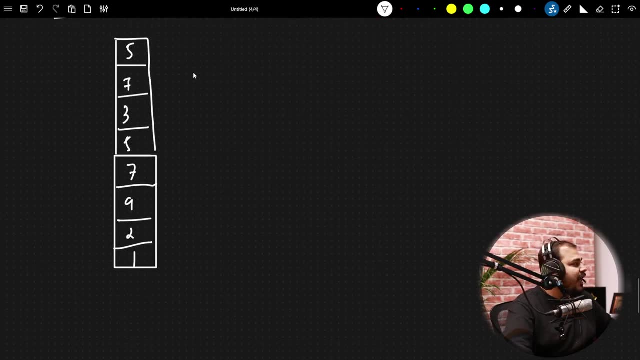 this. So now my 7921 will also get attached over here, Right? Similarly, I am going to flatten this entire, all the filter outputs, and I am going to combine it over here. Okay, This is basically called as a flattening layer. 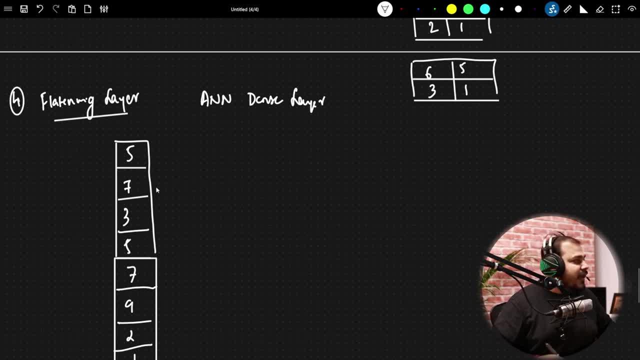 I am just flattening it, I am just elongating it, and now this becomes an input to my dense layer. Then you go and create a fully neural network connected layer, and how many number of outputs you have. suppose if I am doing image classification of cat or dog, this will get connected like 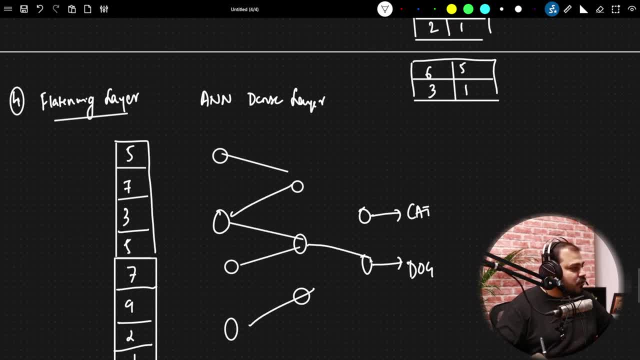 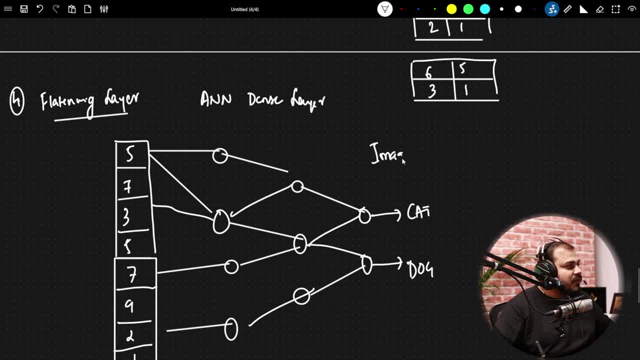 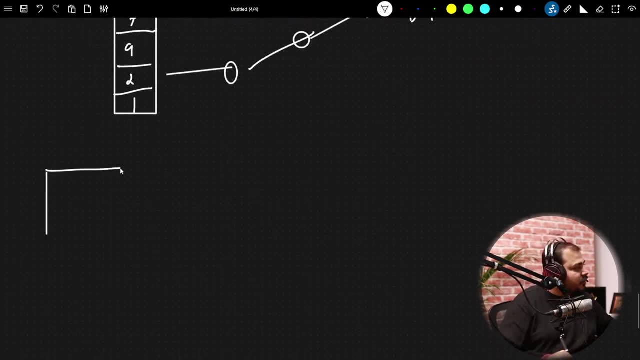 Okay, And finally, I will be able to do this image classification in this specific way. Everybody clear of the entire process. In short, what all things we did? let's say this is my convolution operation, convolution operation. then I went to my max pooling layer. 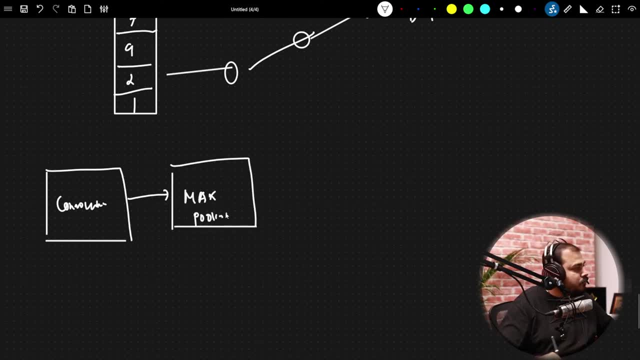 Okay, Max pooling, This convolution operation has what all things: convolution: padding, applying filters, everything happens inside this and after the max pooling layer, what we specifically do? we provide it to the next stage, which is called as flattening layer, and then we create a ANN or fully connected. 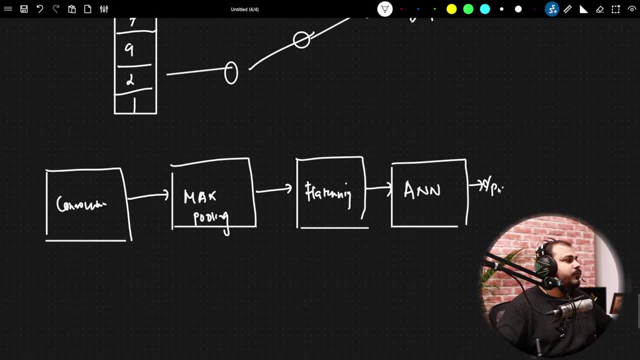 neural network and, finally, I get my output Right. So these are my entire steps. please do let me know whether you have understood or not. Till then, I am just going to go ahead and start the next step. Okay, I am just going to open some examples. okay, 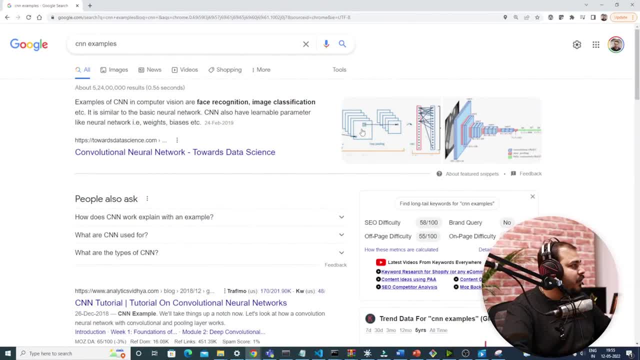 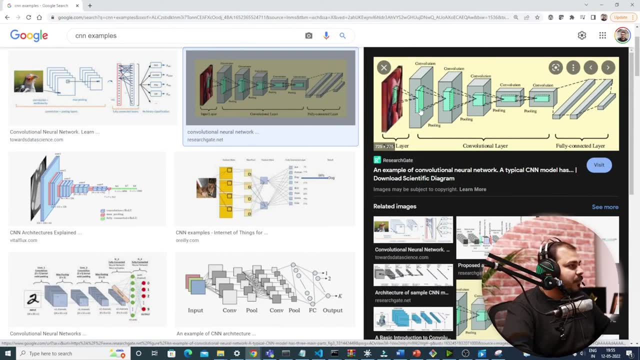 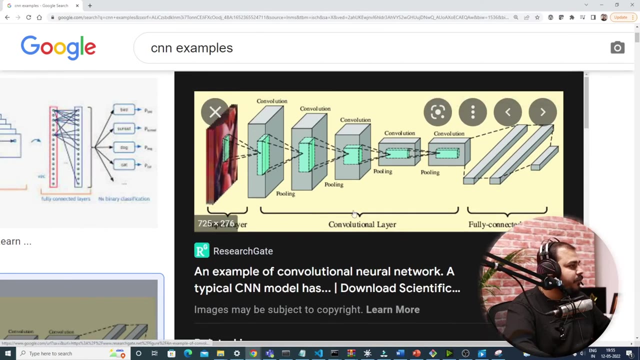 So I am just going to open this browser. everyone see over here if I probably try to go and click on images now. you see over here, right? this is my image. okay, probably you will be able to see over here very clearly. let's say again this: I have taken from Google, see this. 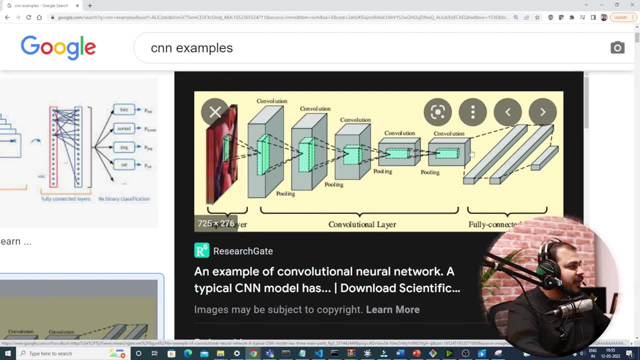 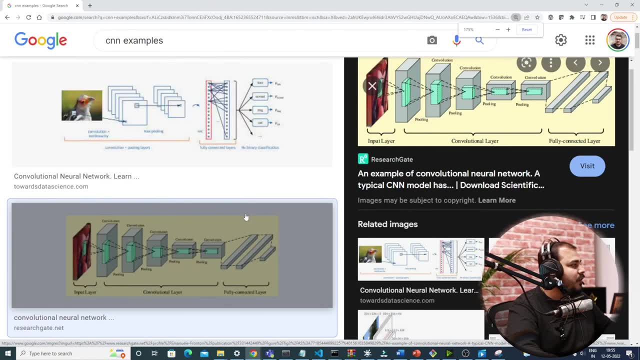 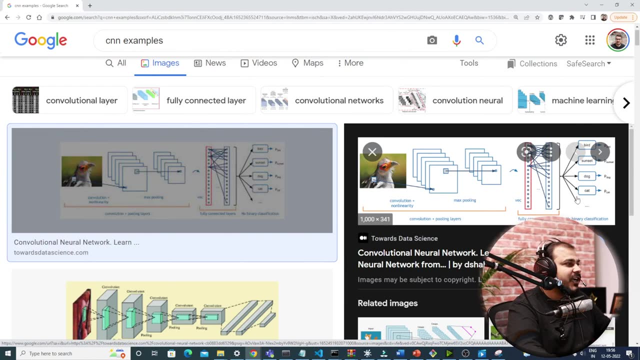 convolution pooling, convolution pooling, convolution pooling, then flattening, then fully connected layer. Okay, So this way you will be able to see. you can also see other other examples: convolution, nonlinearity, max pooling, fully connected layer and classification. right, So we give this image. each and every pixel gets passed. all the information is basically. 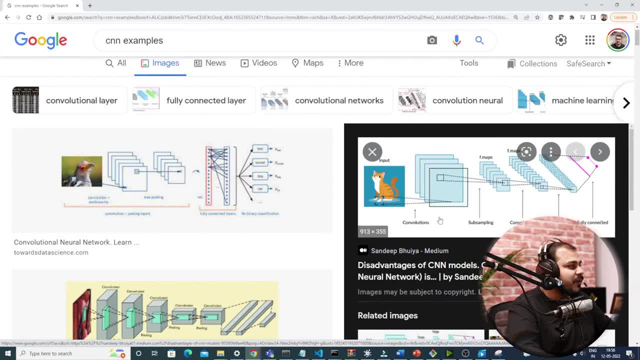 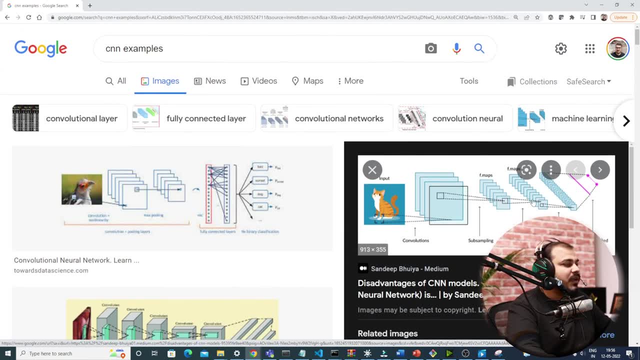 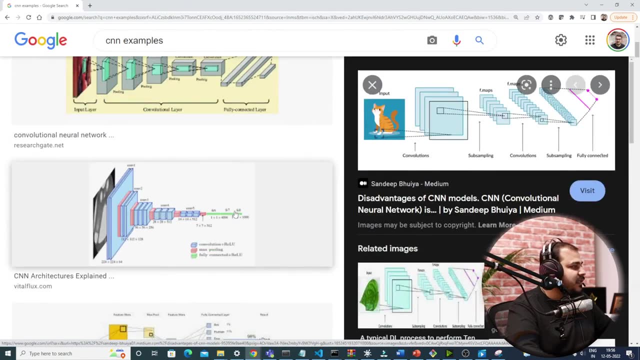 getting extracted. similarly. here also you can see this is my input image. I pass it through convolution, then I basically got the filters output. then what we did we did: applied another convolution layer, Okay, got a fully connected layer, you know, and then finally we got a output. so like this kind of 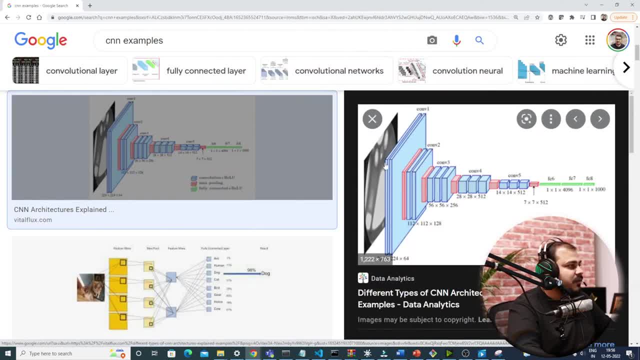 operations you will be able to see. see here also this image: we applied to convolution layer, then we applied a max pooling- red color is max pooling layer. then you can see that we have got another convolution layer. then again, we applied a max pooling, then we applied convolution layer three. 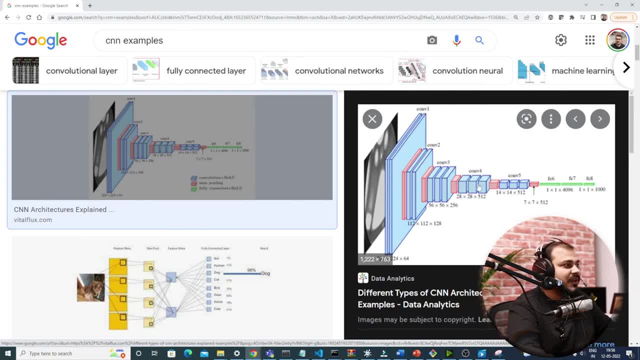 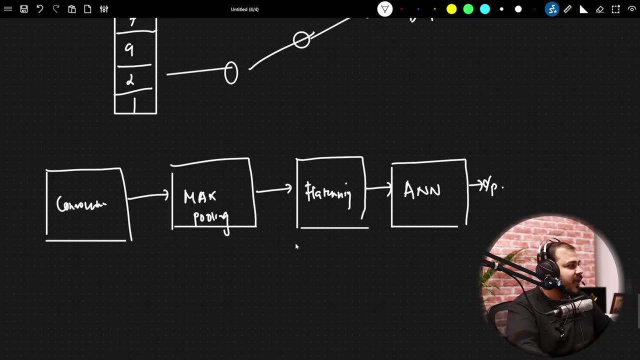 three times convolution layer. then we got a max pooling, then convolution, max pooling, convolution, then finally fully connected layer. fully connected layer and fully connected layer right by default. max pooling layer through the code is basically taking two. so, guys, did you understand whatever i explained with respect to all the cnn neural network? can i get a quick yes, if you are. 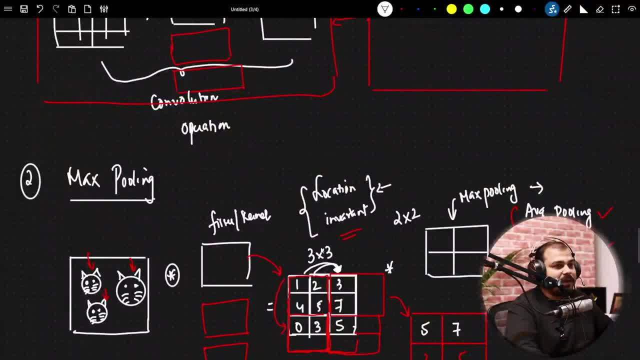 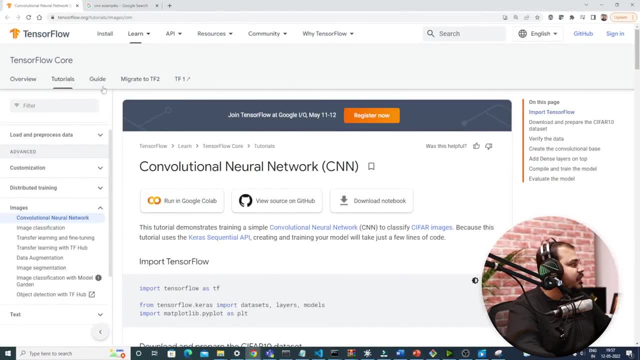 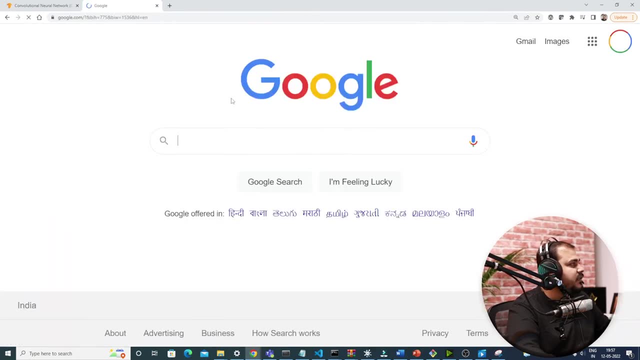 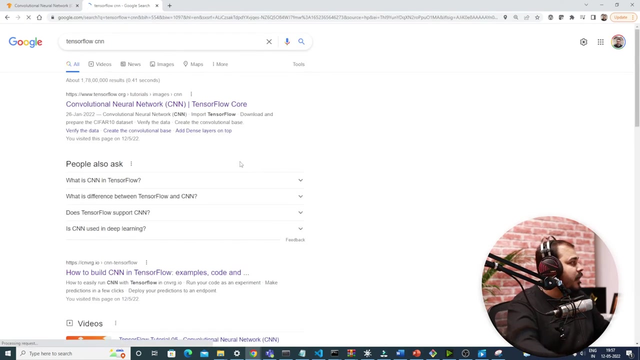 able to understand. now we will try to do one practical example. yes, so what i want you all to do is that just go and search for uh, tensorflow images cnn. just search for tensorflow cnn. like this: just go and search for tensorflow cnn, and here you will be able to see the first. 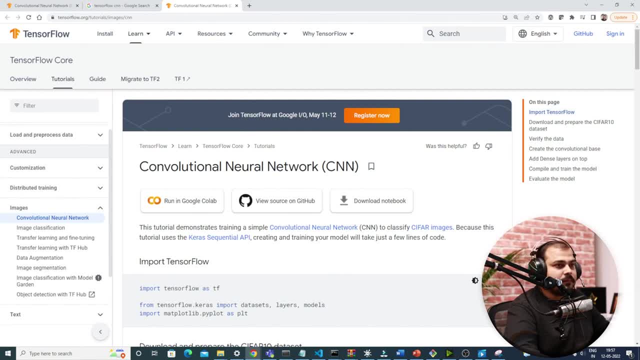 over here an example over here: okay, okay, now you cannot determine. one thing is that how many layers you can actually use. okay, so there you need to understand from the transfer learning. people play with different kind of layers. there is an image net competition where people focus on understanding that how many layers needs to. 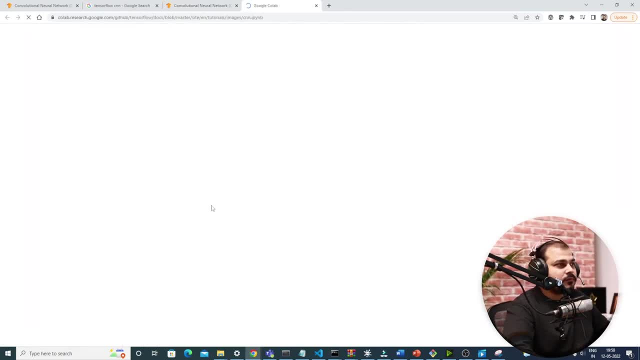 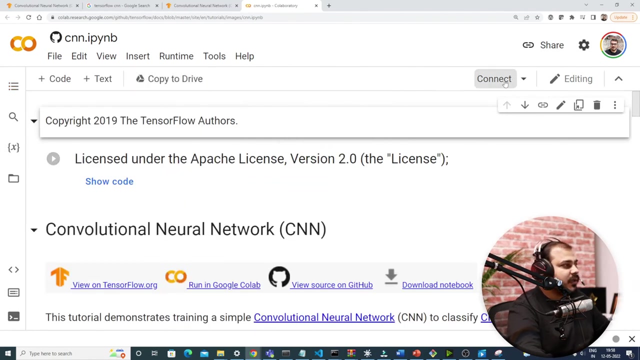 be used now. just go and click on run in google collab once you search this convolution neural network. go and click on run in google collab and here use your specific output automatically. when the traversing of the entire images will complete, you will get the image traversing will get complete. 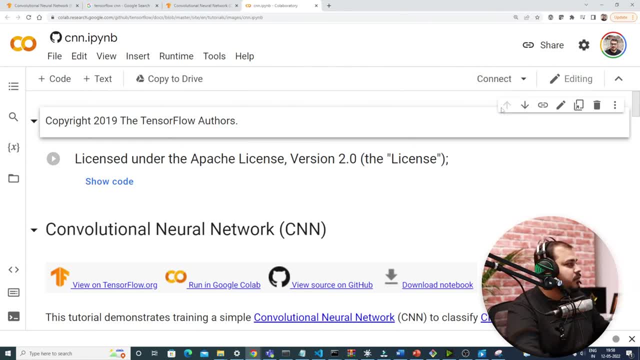 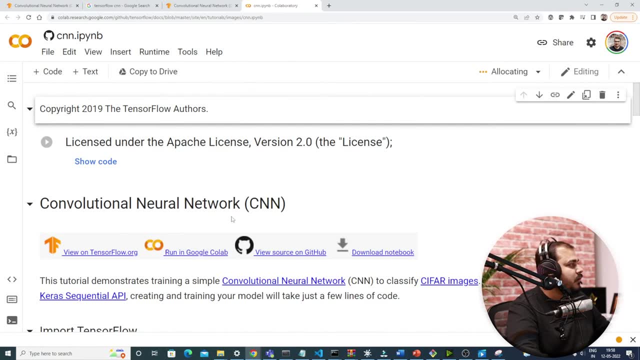 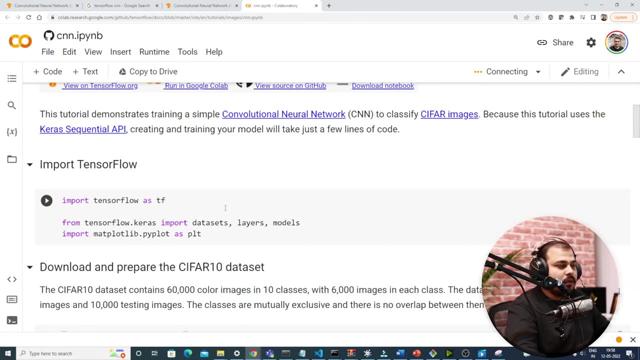 that time the stride stride will stop moving. okay, so here is my tensorflow connected and i'm going to change the runtime to gpu save, connect it. okay. so here you can see that what all things we have actually done. okay for this um. max pooling is specifically related to extracting more information. 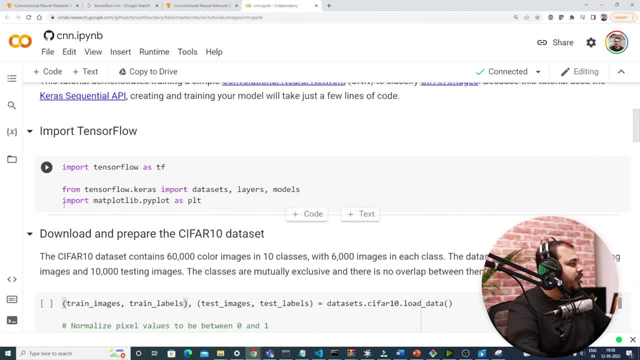 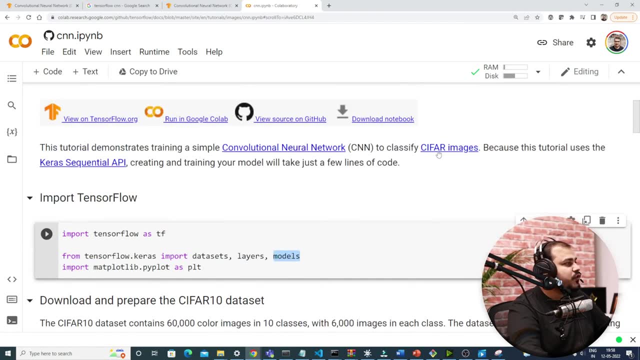 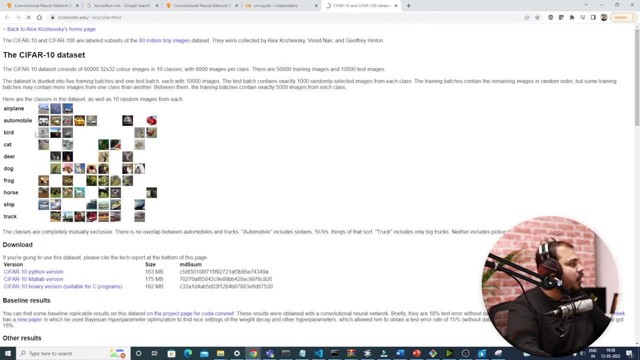 from a specific image. okay, so, as usual, i'm going to import tensorflow, tensorflow, keras. i'm going to use data set layers and models. what kind of data set we are going to use? we are going to use cifar images, data set. so if you click on this, cifar images has what? all things it has, this all. 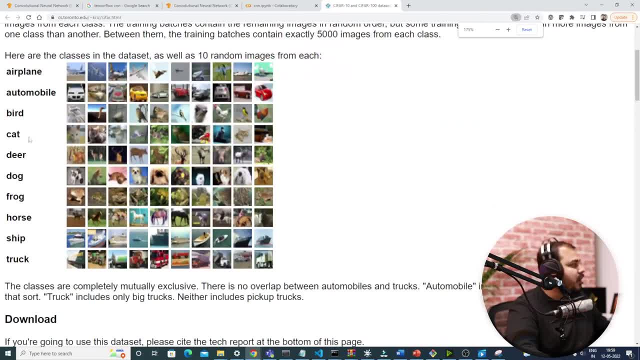 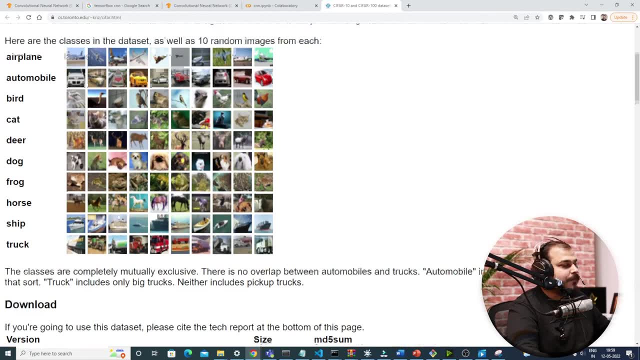 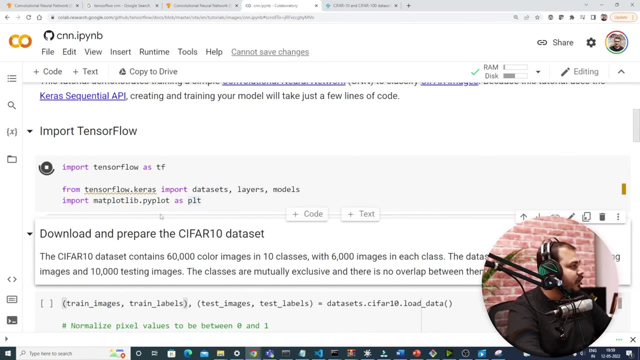 kind of images like airplane, automobile, bird, cat, deer dog. so we are going to classify. whenever we get this kind of images, we are going to classify them. okay, now let's go ahead and let's quickly execute. so here, first step, i'm just going to execute the tensorflow part. it will get a. 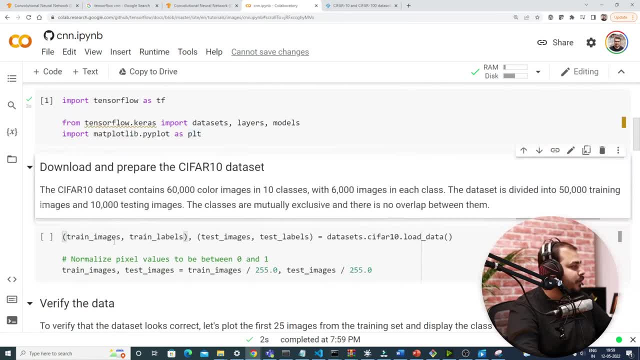 get executed. let's see how much time. yes, it has got executed. now let's download and prepare the cifar 10 disaster. this data set contains 60 000 color image in 10 classes, with 6 000 images in each class. the data set is dividing into 50 000 training and test, 10 000 as test image. 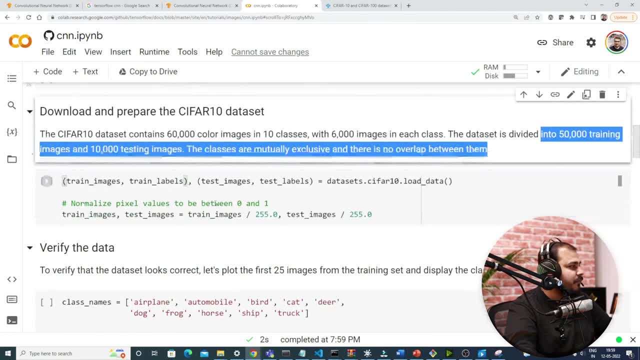 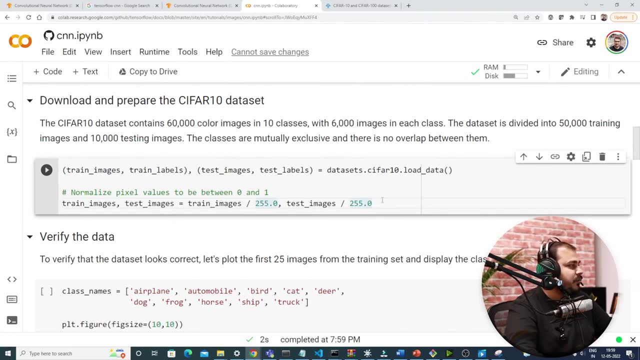 these classes are mutually exclusive and there is no overlap between them. fine, we know all these things, and then we are going to basically say: training images, training label, training test images and labels. okay, as i said, we need to normalize the values to between 0 to 1.. 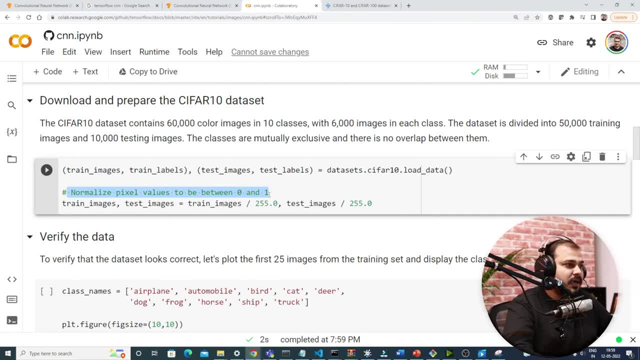 in the first stage. we have already discussed this while explaining the theoretical part. we will normalize it and we will always make it between 0 to 1.. so all we are doing is that the training and the test image. we are dividing it by 255.0. if the pixels are 255, it will become zero. 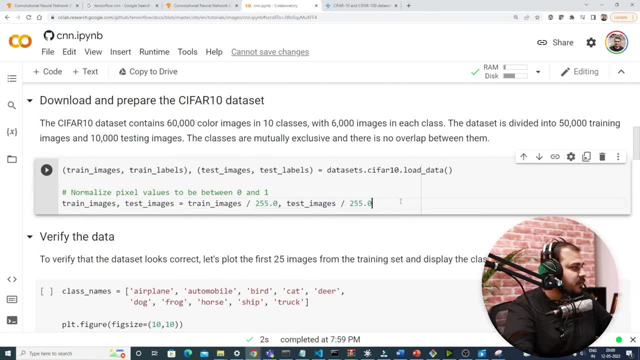 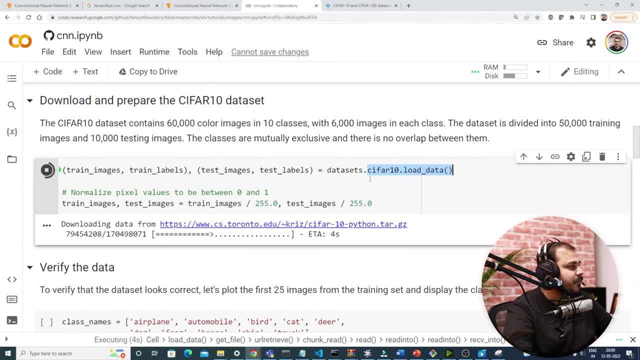 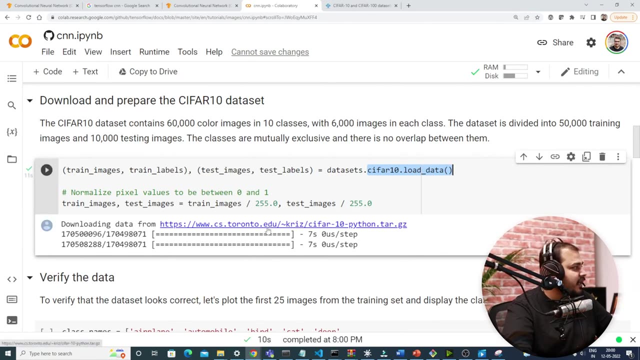 sorry one, otherwise it will become zero if the values are zero pixels. okay, so i'm just going to execute this and automatically this data set will be downloaded from this particular library. data sets: dot, cifar, 10, dot. load data. okay, so you can just execute this quickly, get it, and here you can see that i have downloaded. 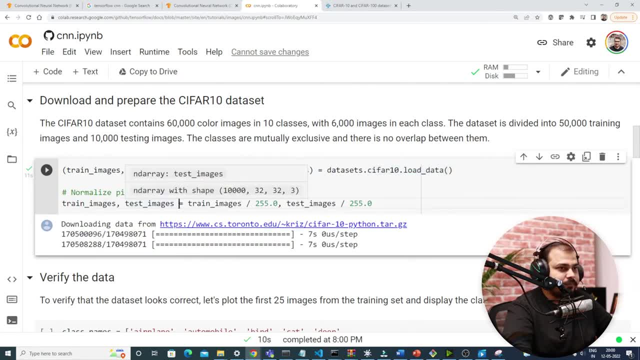 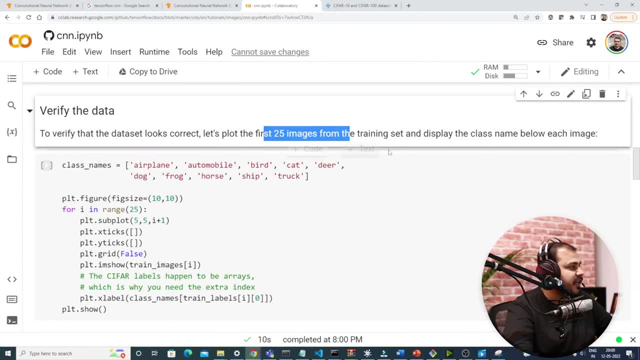 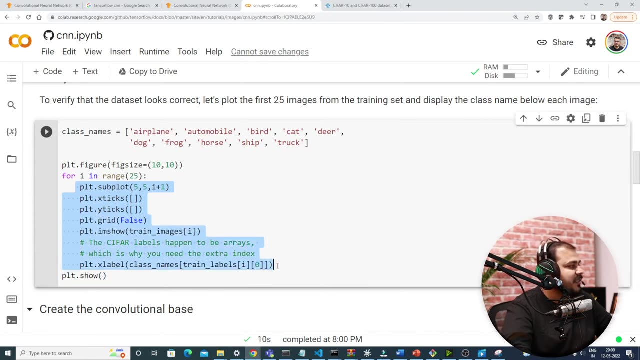 all the data set from using this specific uh example. okay, now verifying the data set. to verify the data set, let's plot the first 25 image from the training set. so we are just plotting it. that is the reason we use matplotlib. i don't think i need to explain you this, because 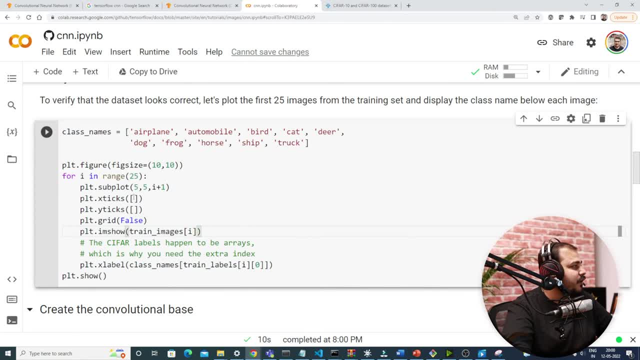 you already know, maybe knowing matplotlib. okay, so here what we are doing, based on the class names. we are plotting it and i'm taking the training labels and first 25 image. whatever i get, i'm just plotting it over here. so once i execute this, you will be able to see that. 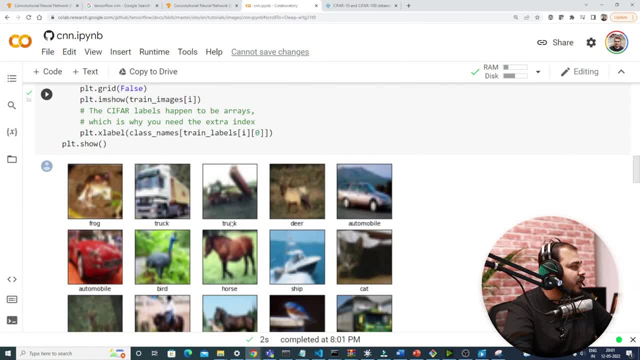 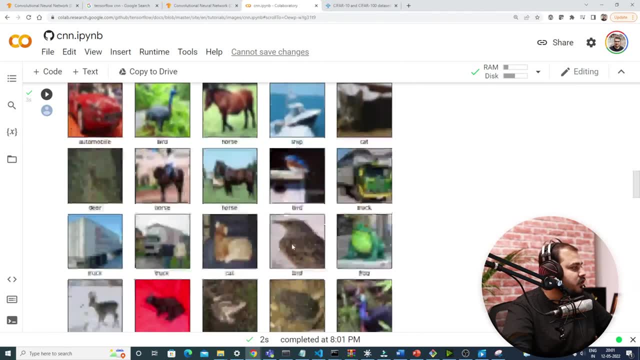 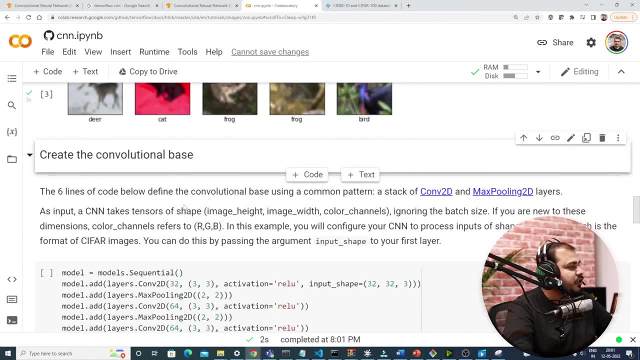 i'm able to get the first 25 images which looks like frog, truck, truck, deer, automobile, automobile, bird, horse, ship, cat, deer, horse, source, source- everything i'm actually being able to get. okay, then let's go ahead and create a convolution neural network. now see this guys. 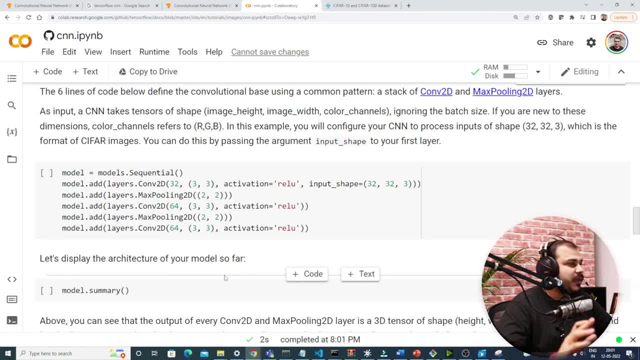 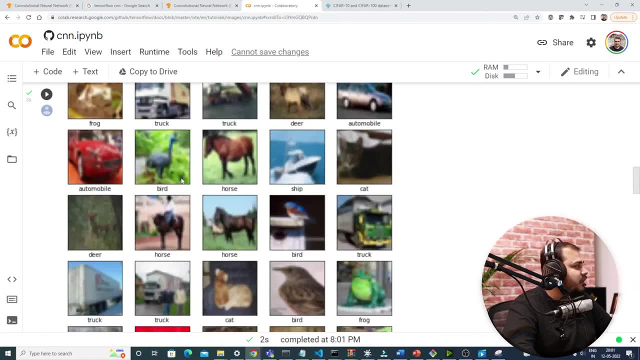 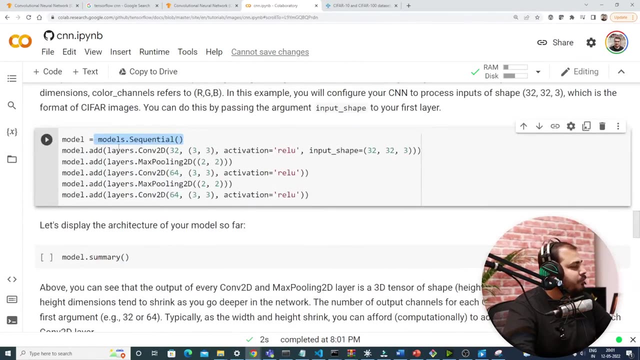 this is super important, super easy. if you are focusing away, you'll be able to understand. in the a and n also, we first of all initialize our models with sequential right. so in this also we will definitely first let me see that whether i've okay layers models has been imported fine. so 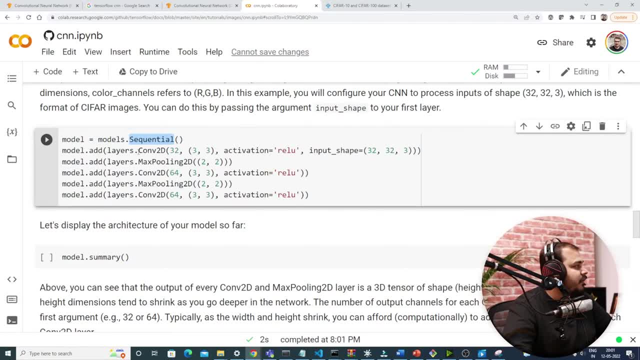 we have to again initialize with a sequential layer and then we will be using modeladd. we will use modeladd and then we will be using modeladd. again initialize with a sequential layer and then we will be using modeladd. layerscon2d- convolution layer. right now in convolution layer, this 32. okay, this 32 will. 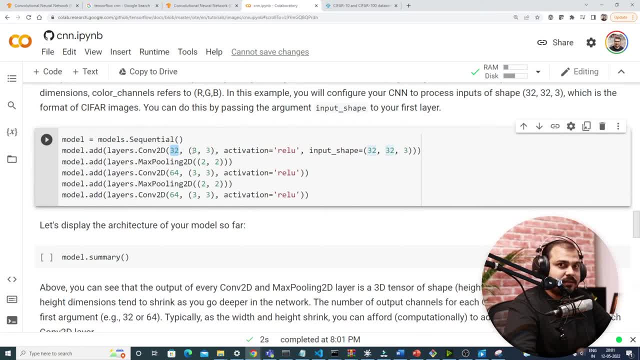 basically be my number of filters. okay, 32 over here. the first parameter that you see right, it will be number of filters. so that basically means we are going to use 32 filters and this filters are nothing but 3 cross 3 size. okay, each and every filter will be 3 cross 3 size, but how many total? 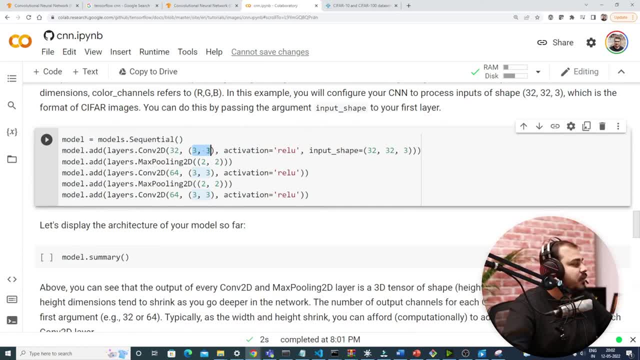 number of filters that we are actually going to use. it is nothing but 32. okay, and you know that after the convolution operation, i need to apply my activation function as relu. so i have applied an activation function as relu and this is super important, like what kind of input image we are. 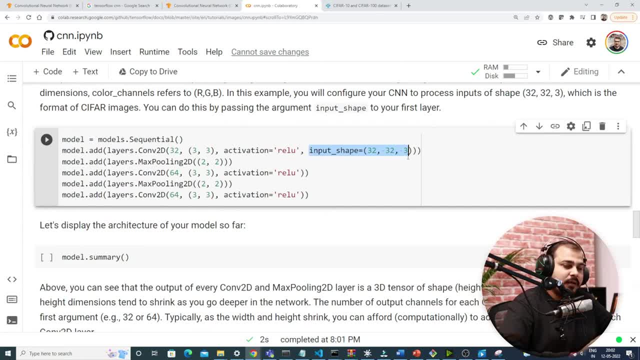 giving, as i said, that my input image, okay, will be basically in a rgb format. if it is in rgb format, this basically indicates that my input image is 32 cross 32 pixels multiplied by 3 channel. okay, so here you can basically see the 3 channel. so it is nothing but 32 cross, 32 cross 3. 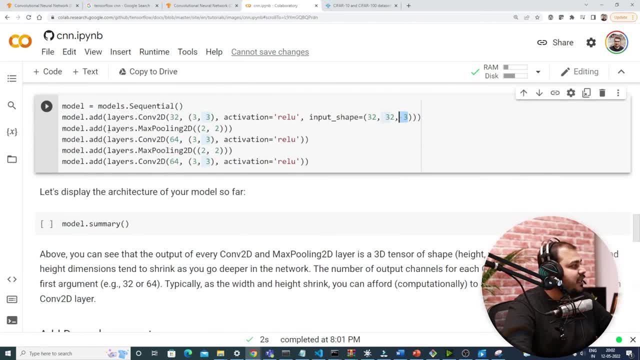 based on the 3 channels itself, and then i'm going to basically add max pooling layer. so after the convolution layer i'm going to add some max pooling, max pooling layer, 2d layer, basically like 2 cross 2 matrix. okay, so it will be a filter of 2 cross 2 and similarly i will go and add my 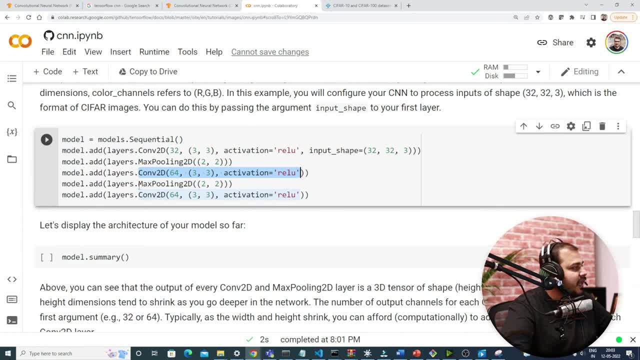 another convolution, then again apply an activation function. then again i can apply a max pooling layer with 2 cross 2. then again i'm applying an activation function, and then again i can apply a activation con convolution layer. over here i'm specifically using 64 as filters. now you may be. 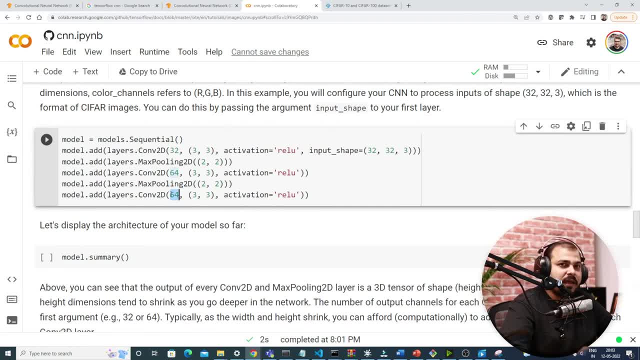 thinking: krish, how do you decide this number of filters? okay, see guys, there is no such thing that you can decide or you can do. you can write any filters over here, but it is a proper research that usually happens with filters. filters are just like in a hyper parameter, like how many filters you? 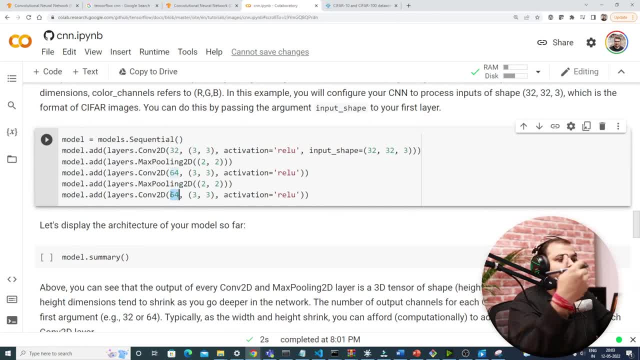 want to basically solve a specific problem. if you try to see in some of the state of art algorithms right in convolution neural network, there you'll be seeing different, different number of filters. so no such specific thing. yes, you can try with different, different hyper parameter. you can use 32. 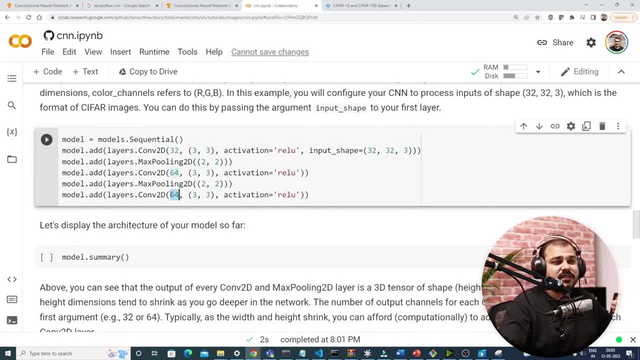 64, you can use the combination of different different filter and see how the performance is increasing right. other than that, most of the time for different kind of tasks like image classification, object detection, we basically use the state of art algorithm. okay, so i'm just going to execute this. so that is basically means that i have three convolution layer three. 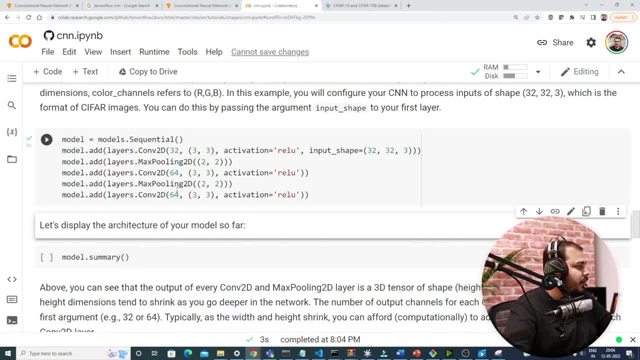 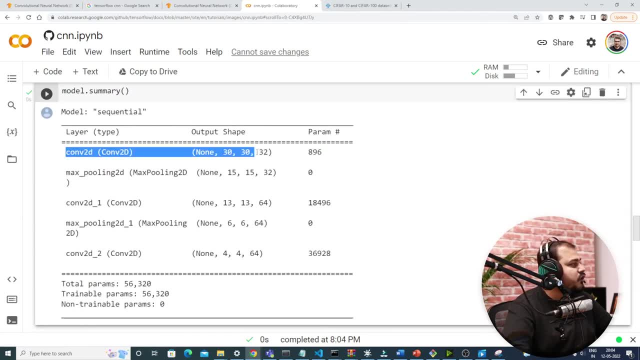 and one two max pulling layer, just stacked horizontally. finally, if you go and click on modelsummary, you'll be able to see the entire summary. see, it starts with convolution, 2d layer. it takes an input of 30 cross 30. the filters are 32, then we go with 15 cross 15, then the this is 32. 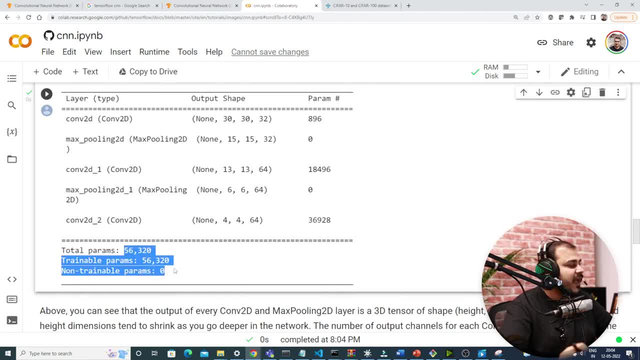 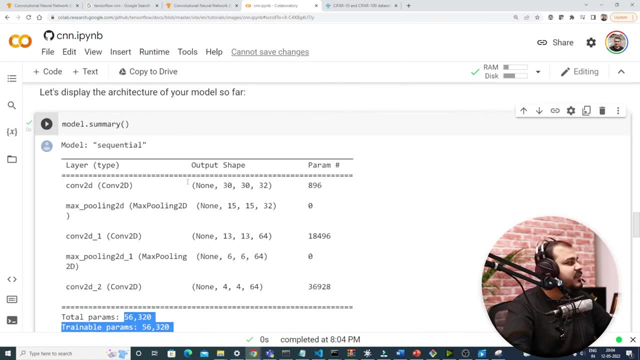 then total number of parameters. this is basically defining, and this parameters even counts the parameter inside the filters. okay, so by this specific way you are able to see the entire summary of the model, like how the model is actually created. now till after this i told you right. 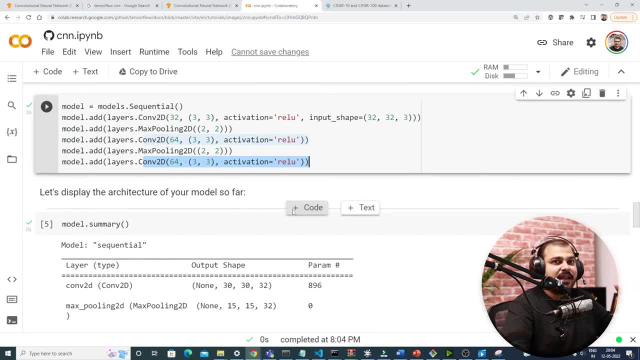 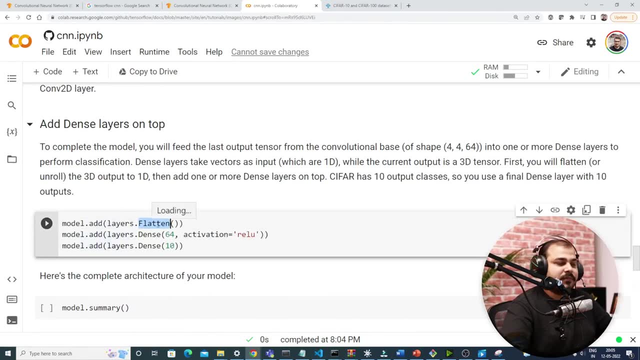 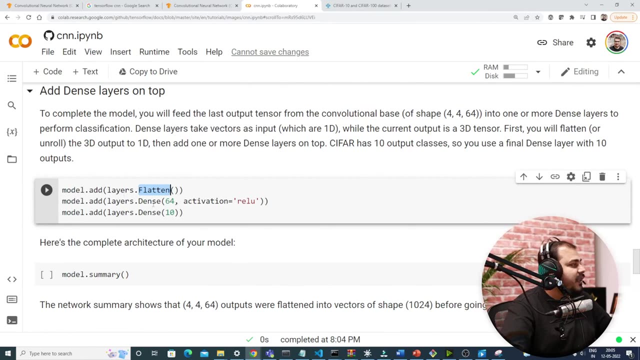 after we finish up this. you know we can have a flattening layer. now is the flattening layer defined here. you can see that model dot layer, layer dot flatten. so whatever we had over here, we are just going to flatten this entire layer and we are going to add it over here. 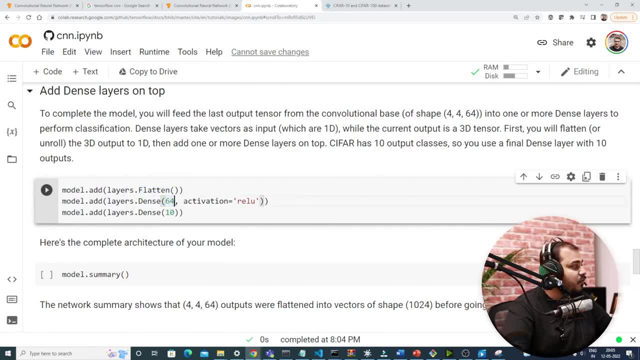 and then i'm going to add a fully connected neuron network with 64 dense neurons and to total number of output in my data set is 10, so i'm specifically writing layer dot dense of 10.. so this is my output layer and this is my hidden layer, right, the ann layer, which has 64 neurons, and this is 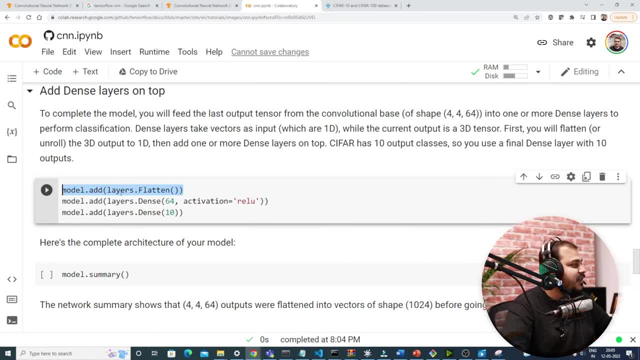 basically my flattening process and i've just written layers, dot, flatten. that's it. whatever is coming after the convolution layer, we are just going to flatten it and we are going to use it. okay, so once we execute this, you will be able to see that my model will be ready and, if i probably 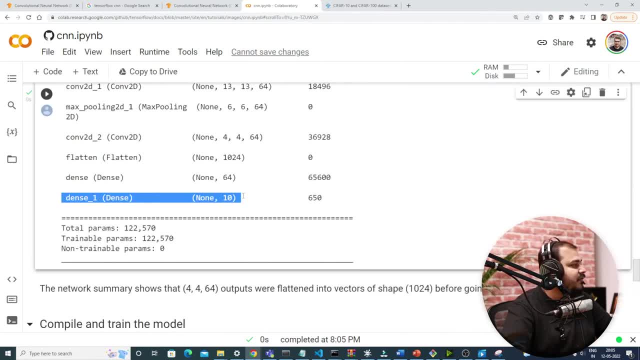 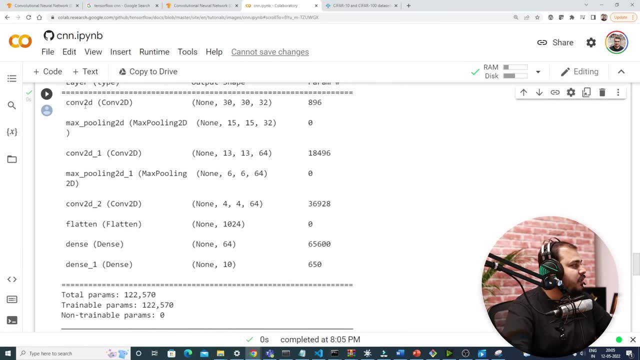 now go and see my model dot summary. here you can see my dense layer, which is my final layer. i have my 10 output, then i have my dense layer, i have my flatten layer con 2d max pooling: 2d, 2d, 2d right. so here i am. 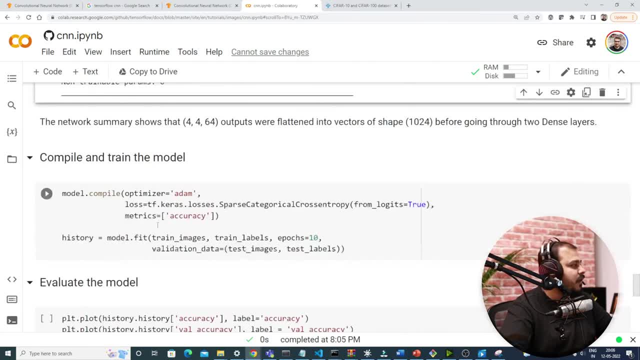 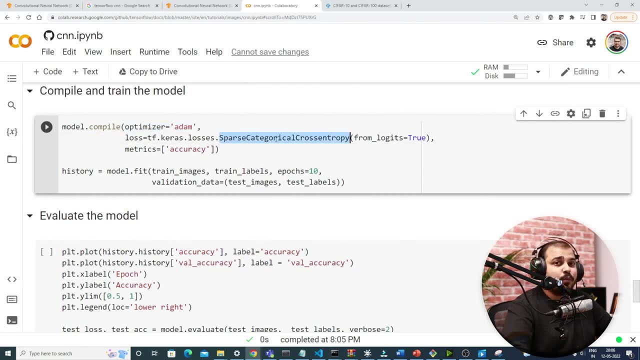 specifically getting all the layers that i specifically want. finally, for the compilation, we'll use the same optimizer, which is called as adam optimizer, and since we have many, many, many, many output, that is, 10 outputs, we are going to use something called a sparse cross entropy. i hope i have discussed about categorical cross entropy and this is what 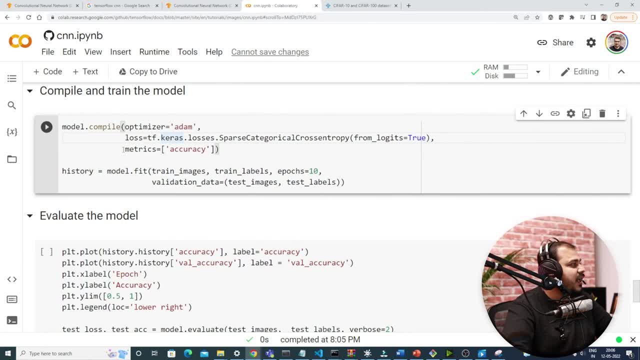 it is all about. you know, we can directly use that in the loss function. and then, finally, you can see my matrix accuracy and i'm going to do the fit on train images, train labels, epochs- i'm basically using 10 and the validation data also i'm giving by test images and test label. so finally, i execute. 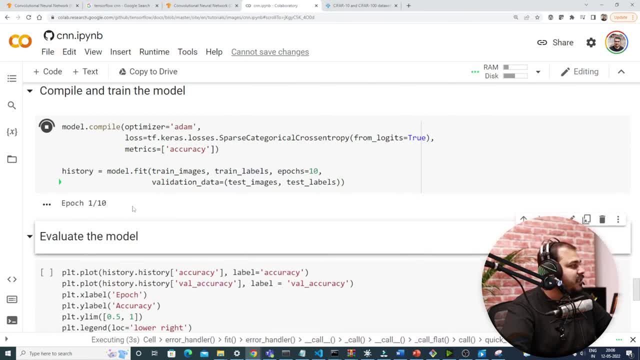 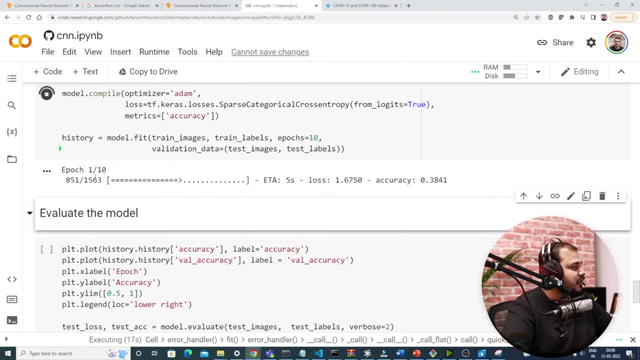 this and you will be able to see. my epoch will probably start, and let's see how much time it made take. uh, it depends on the gpu that we are trying to use, but i think this should get completed and started. here you can basically say that i'm basically using this one, and here you can see. 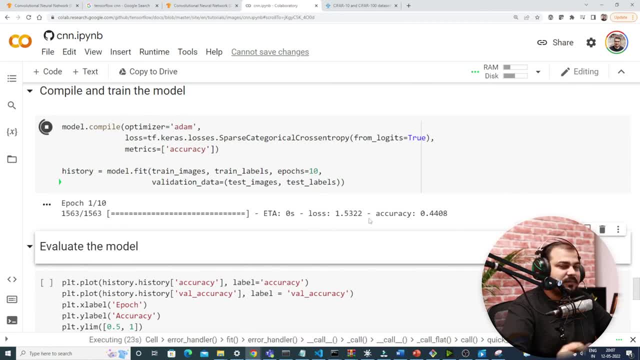 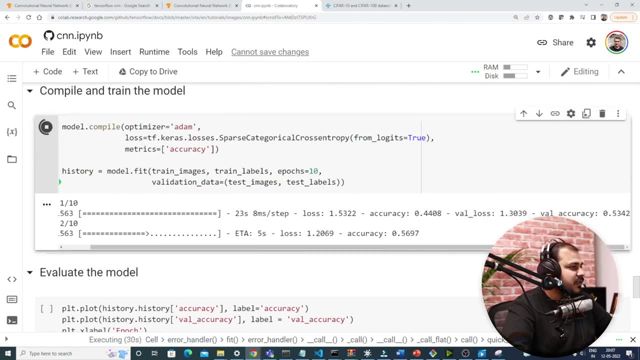 that my accuracy is increasing. my loss is decreasing. that basically means my neural network is getting trained. well, my accuracy has gone more than 56 percent. let's see: the validation accuracy is also 53 percent. test training accuracy is 0.44, when my validation accuracy 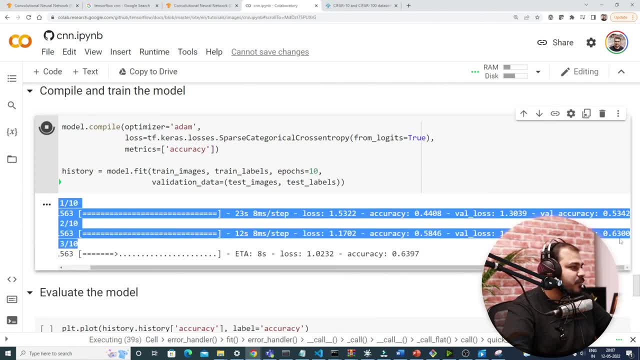 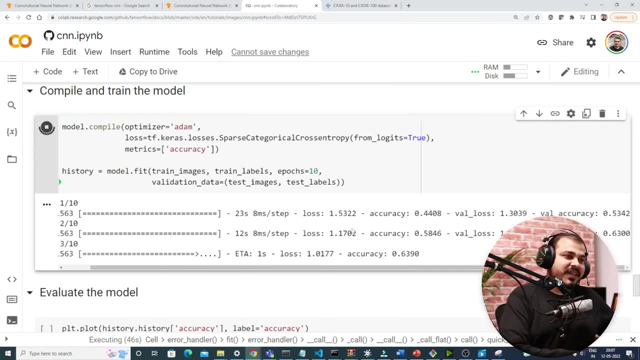 is much more better and here you can see my validation accuracy is much more better than my training accuracy, and this will keep on going right. so i hope you are understanding everyone. can i get a quick yes, and we'll wait till the training is going on. please make sure that you comment down. 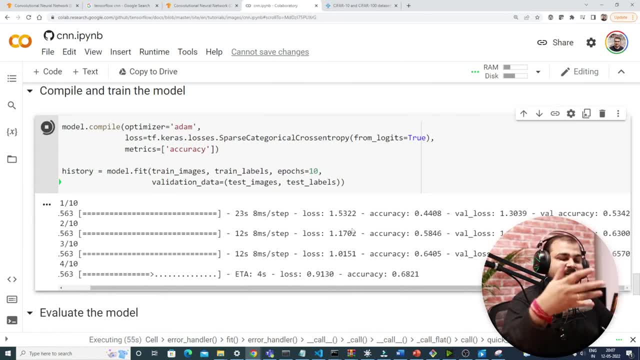 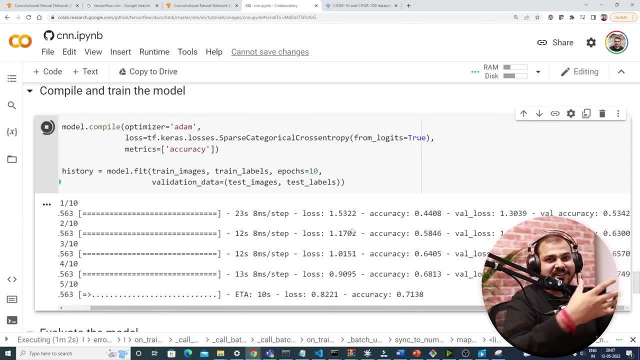 give some heart likes, something like that, you know, so that it will also help me boost my confidence with respect to teaching and it will energize my entire teaching methodology that i use. okay, yes, so we are in the fifth epoch. uh, right now, the accuracy is 70 percent. validation increase is 68. 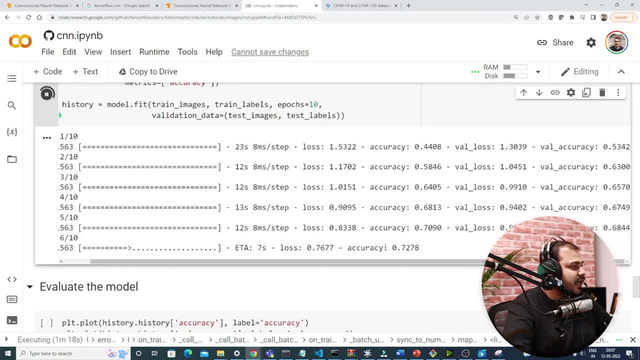 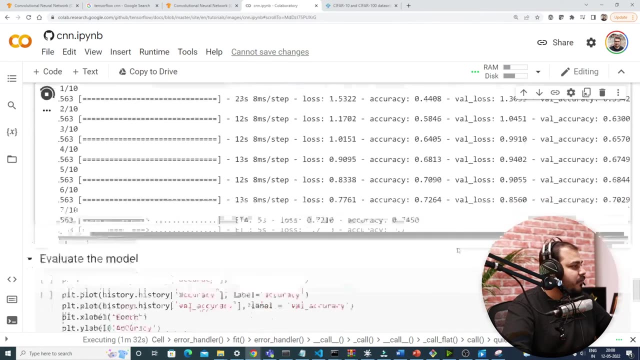 we are going on good, and on this also, you can apply early stop, you know, so early stop can also be applied onto this. that i'll give you as a task. okay, so here it is. your accuracy is got to 74, so early stop can also be applied onto this. that i'll give you as a task. 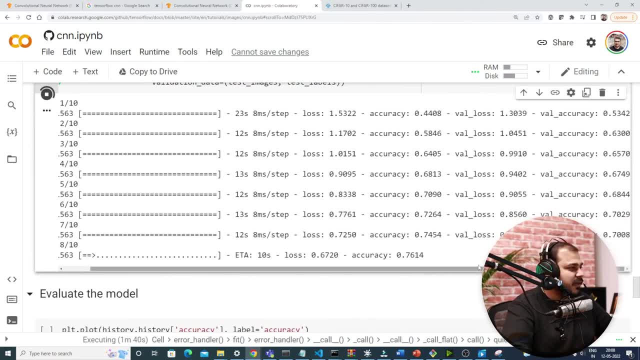 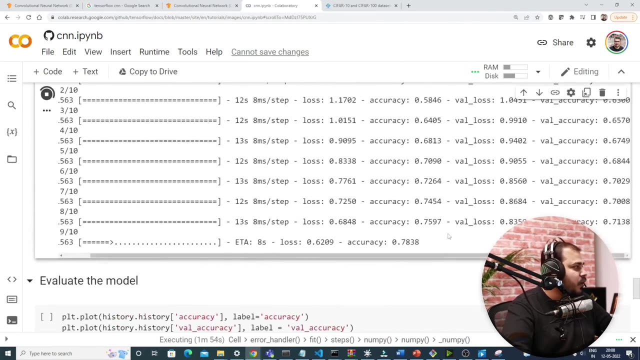 optimizers. you should definitely use adam optimizer because it is the currently the best one. okay, two more epochs and then we'll stop over here just to see that how things are going on right. so 76 percent- 70 percent is my validation accuracy. it's good, it's going on good and i think this can. 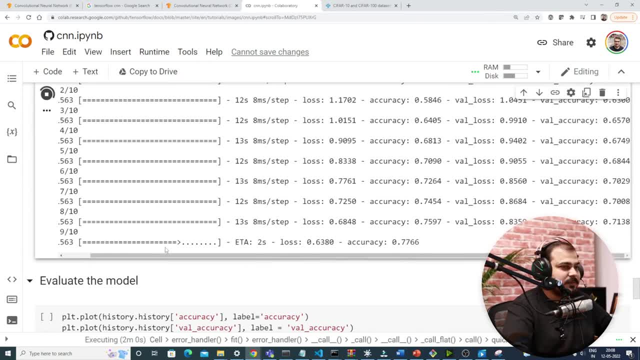 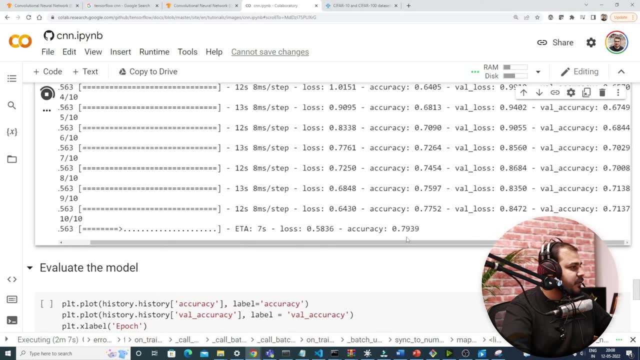 go more than 80 percent if you increase the number of epochs. okay, perfect, perfectos. now i am into 79, accuracy 77, validation is 71, which is good. i think it will be more than sufficient if we complete the 10 epochs, and i think you can also do it. so finally, i'm getting able to get 78 and my 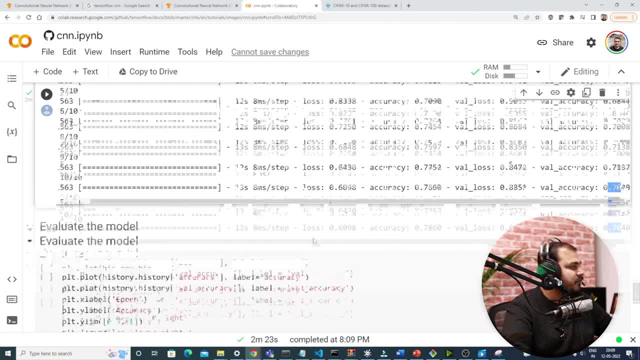 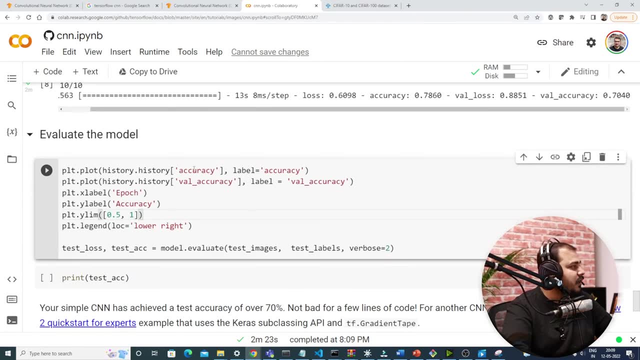 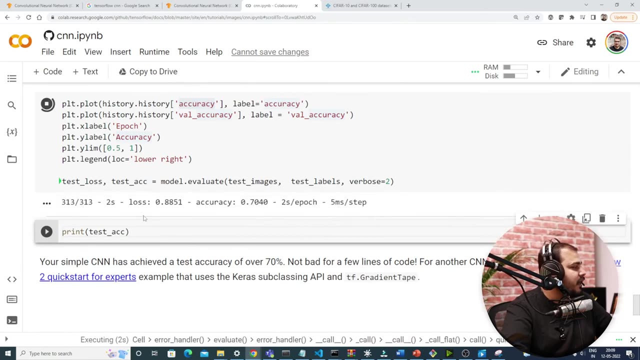 validation increase is 70. i have stopped over here. okay, you can continue the training, however, how many epochs you want, and finally, i will just plot the history accuracy, label accuracy and all with respect to this particular plotting, and we'll also evaluate to this thing, right? so here it is. 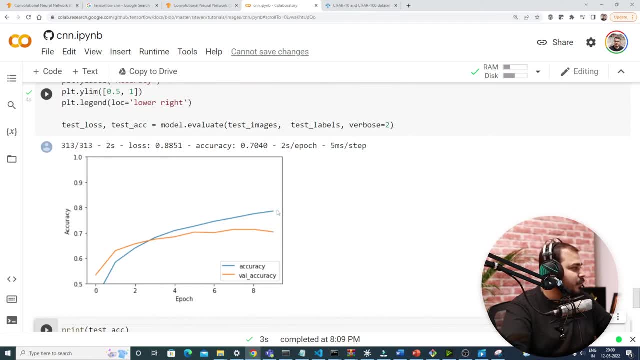 this is my graph. this looks good, right. the accuracy went up. the test accuracy, or validation accuracy, was going down, so we stopped over there. we can also do early stopping so that it will get stopped over here itself if it goes down. this gap should be minimal. okay, it should not be more. 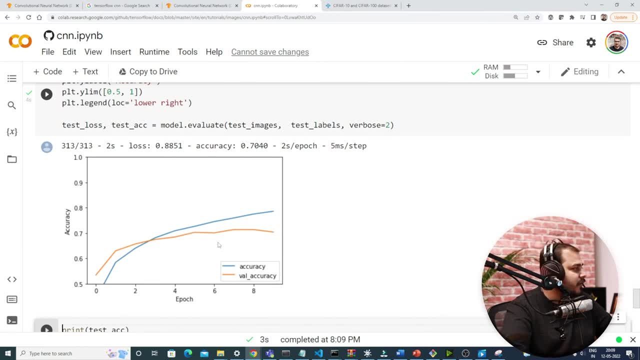 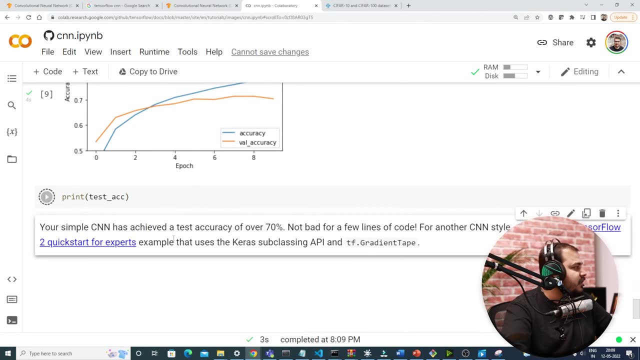 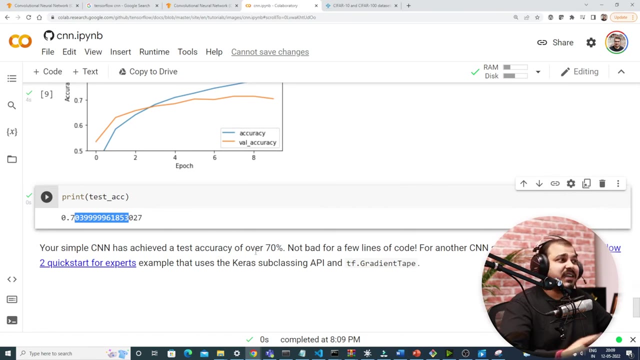 this gap should be minimal. so for that many number of epochs, if you are able to train like over here, you can see the gap was minimal. so so if i go and probably see my test accuracy, it is somewhere around 70.3 percent. not bad, we have achieved this. we can still train much in a better way. 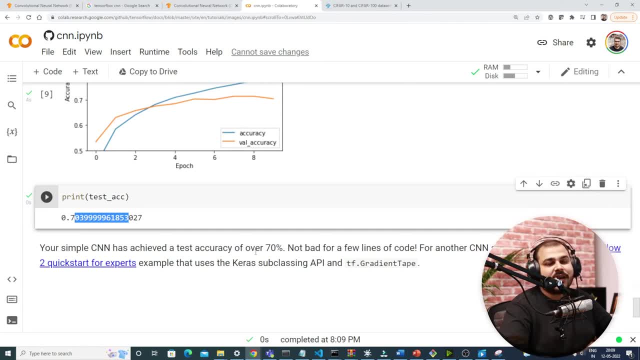 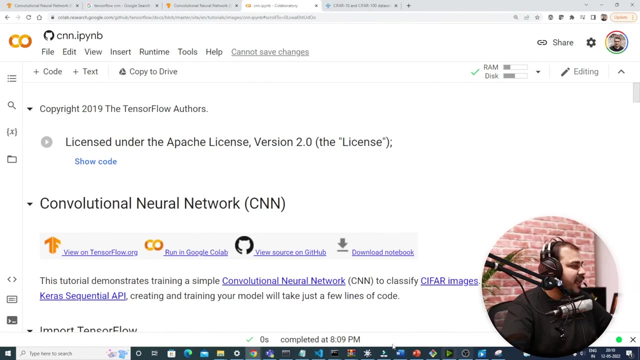 and try to add more layers, try to train it with the early stopping, try to increase the number of epochs and it will definitely give us a good accuracy. okay, so i hope you have understood this entire thing, guys. it was good enough. i have explained you completely in depth with respect to cnn. i'll take up one more live. 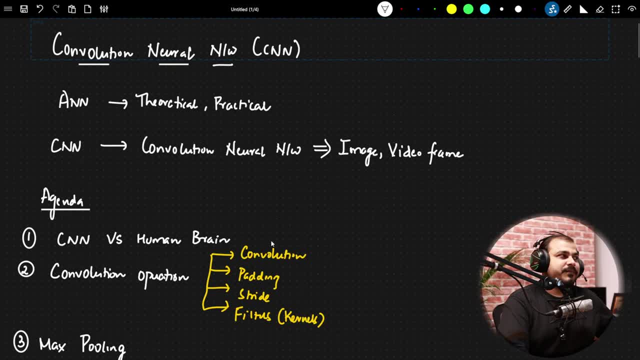 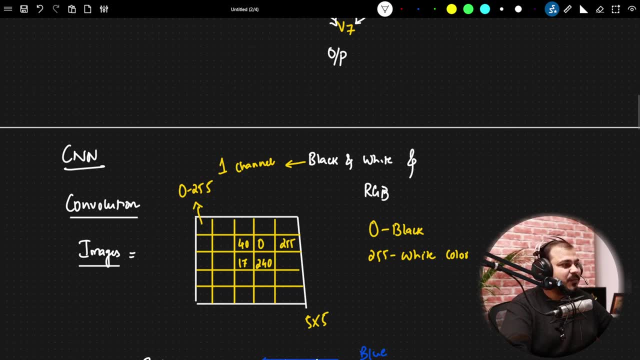 session to make you understand about transfer learning. uh, this was it from my side. i hope you like this particular video. can i get a quick yes, if you have understood this? it was somewhat important to you all. uh, just reload the video, guys. you will be able to find all the links in. 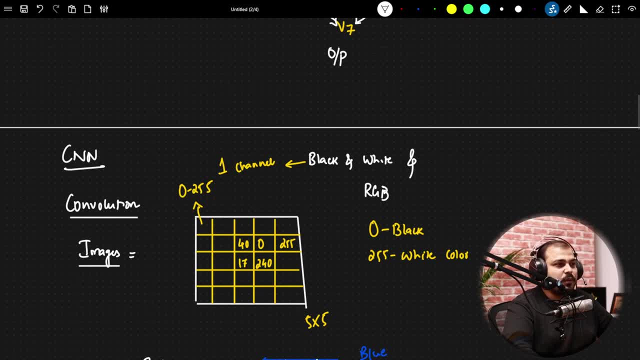 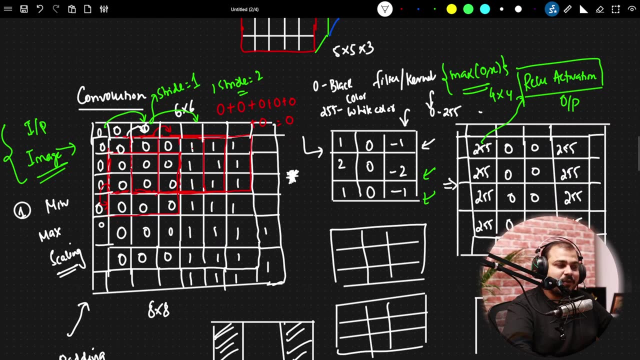 the description where this materials will be put up- everything over there in that community dashboard, which is completely for free. enroll over there, get those materials and use it before going for the interviews. try to cover up all these things, right? so yes, this was it from my side, guys. uh, i hope you like this session. 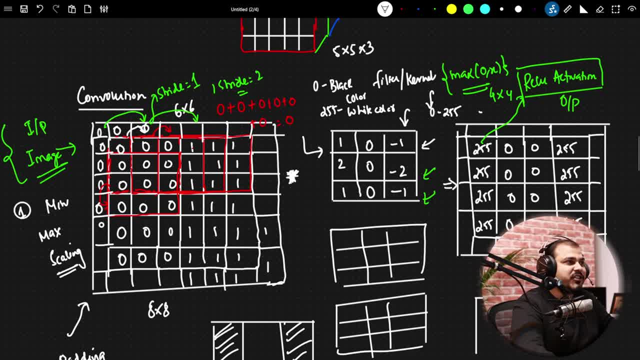 please make sure that you subscribe. uh. i neuron channel, krishnayak, hindi channel, right, and obviously my channel, my. my request is that please share with everyone, guys. please share with everyone. uh, it will always be useful so that we can keep on doing this kind of session, okay, so, yes, this was it from my side. uh, thank you, and uh rnn and all. 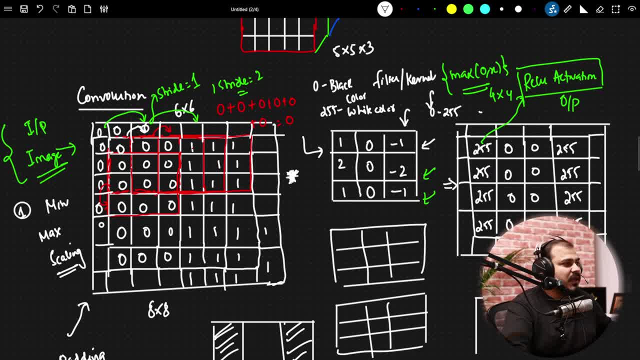 we'll try to do it, but before that, let's complete transfer learning. i'm not sure tomorrow if it is possible or not, but next week monday, let's try to do it. okay? so, thank you guys. uh, keep on rocking, keep on learning. never give up. i'll see you all in the next session. bye, bye, thank you, thank you.